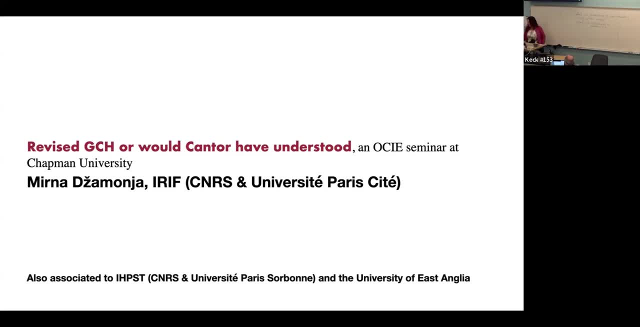 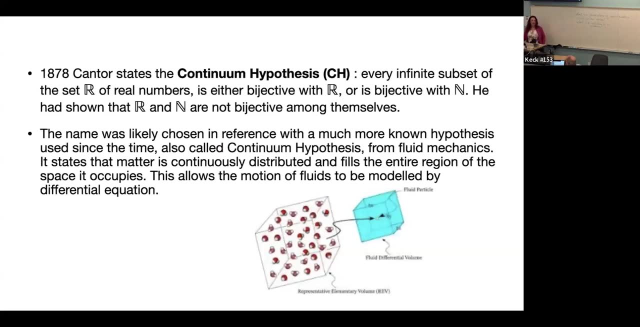 to all senior colleagues who know many things that I will say at the beginning. So it starts exactly there where Pino introduced us to this nice argument, famous argument of Cantor, that there is more transcendental numbers than there are observable numbers. 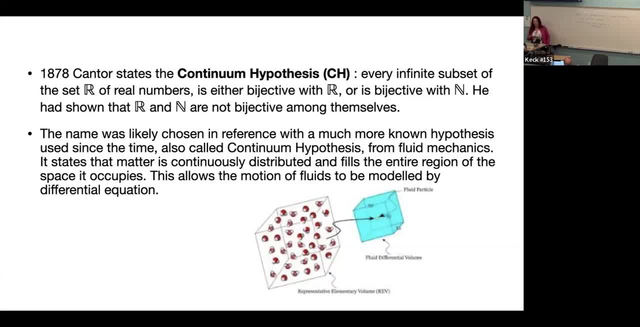 And I would like to say that this was a very big thing that he proved at that time. He was not motivated by sensitivity, by foundations of mathematics or by philosophy. This was certainly not what he was looking for. He, of course, was working at the time when the big thing was to understand series, And he was 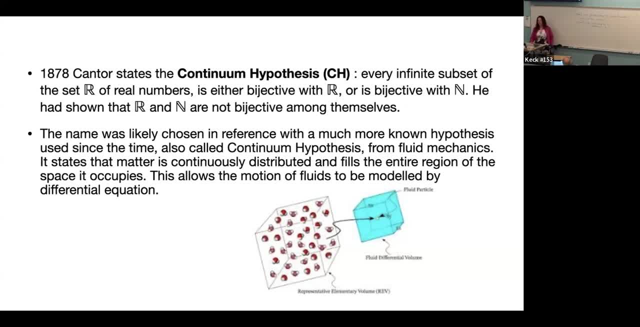 motivated by a problem in trigonometric series, And what this research in series brought at that time was the first transcendental number. So the first transcendental number discovered was given by a muted form of a series, And then, later on, the big question of why being? 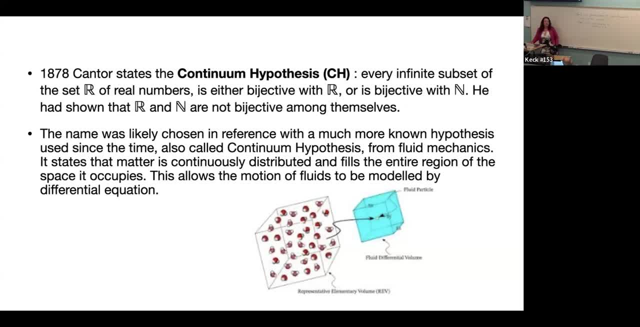 transcendental was known And then, later on, the big question of why being transcendental was known, And then, later on, the big question of why being transcendental was known And he being transcendental. But it's the question that starts to be: how many of these odd transcendental numbers can there be? 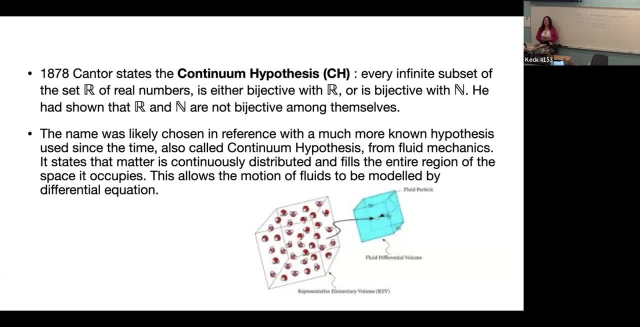 Are they somehow artificial constructions or we need them all? He proved by his method of projections that we have countably many algebraic numbers, So the majority of real numbers are transcendental. So that was his interest, And also let me say that perhaps 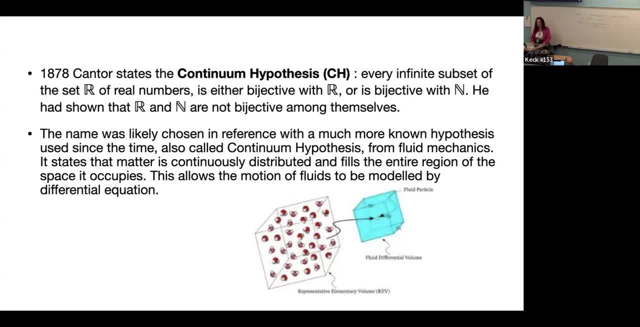 it's less well known that the word continuum hypothesis that he chose to describe his famous hypothesis that every infinite subsets of the real numbers is bijectively the n of the r was not so randomly chosen. It also had to do with analysis and what people were doing in applied. 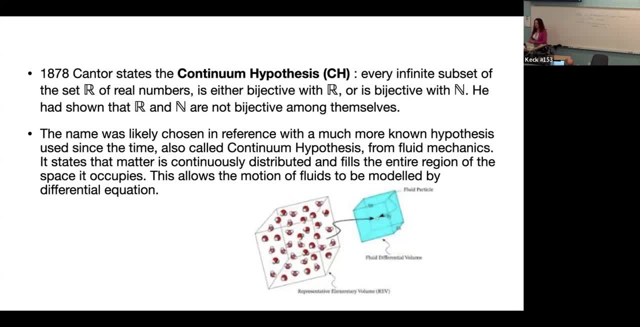 mathematics at the time. So there is a continuum hypothesis in fluid mechanics, which basically is the basic assumption that we can model fluid mechanics, fluids by continuous objects, Because they actually, in physics, are discrete. We have molecules And so these discrete objects are. 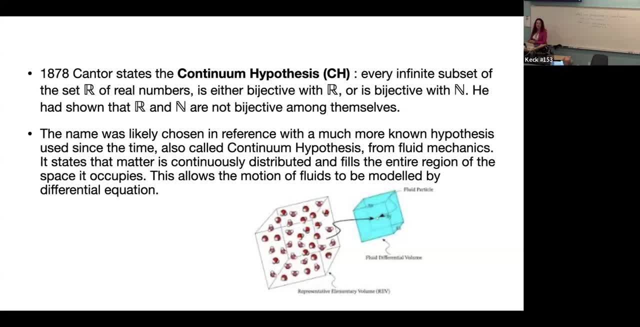 modeled really well by continuous objects, And this is the continuum hypothesis. I did not know. Did you know? Very few people know. actually Very interesting. That's why I thought it is nice to make it up. Yeah, Anyway, in this context, continuous fluid mechanics. 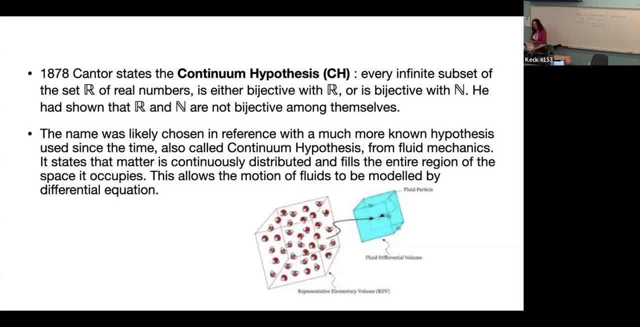 continuity means the continuity of a function, not real numbers. There are two kinds of continuity: Continuity of a function, Of a function. So it's not the same as the continuity of real numbers. Certainly you are right, But I think what Cantor had in mind is that the reals 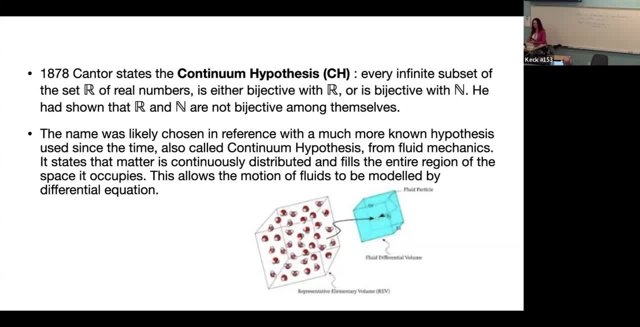 represent the continuum and that the natural numbers represent the discrete. That's right. I agree Absolutely. So this is his hypothesis, and the history of his very good hypothesis is very dramatic. We all know that he not saw the hypothesis, that he felt very bad about that, that he claimed on. 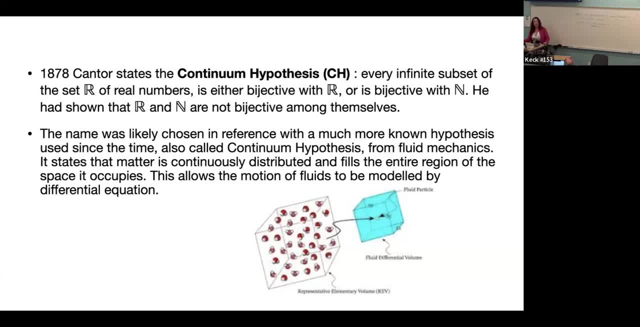 the margin of a paper in 1878 that in the next paper he's going to publish the solution, which wasn't forthcoming. And well, Cantor was mentally ill at the end of his life and some people think that it is because of his efforts to solve his uncertainty. 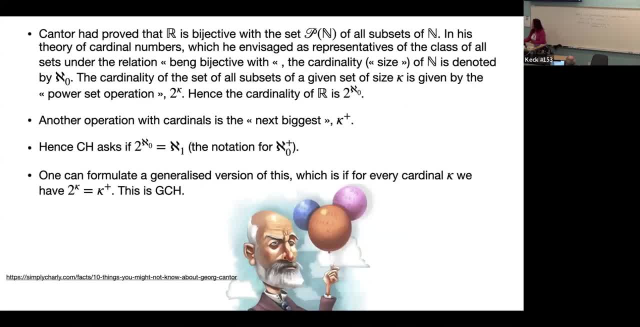 It's probably Sure. So he proved in the proof that we have seen that the reals are bijective in the sense of subsets of n, And this is also in this context that he introduced the operation. so he introduced. 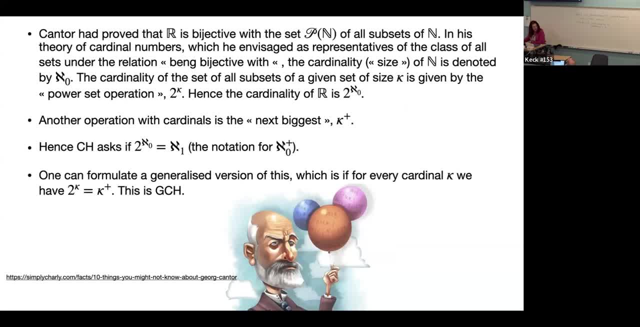 first, the idea of cardinality. So his idea of cardinality doesn't quite fit with what? the way that he defined it now, Because, well, so he assumed that he can just say that I have all the sets, so in all these sets, 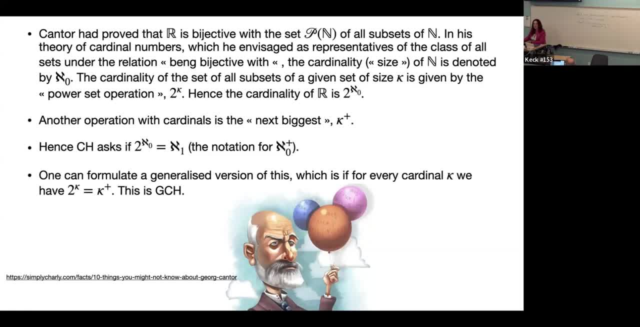 I can make two of them equivalent if they have a bijection between them, and then I can make a quotient. I can take a representative of each class and these are like arguments. So of course, the problem that was realized after the Russell paradox, that the object, that is a 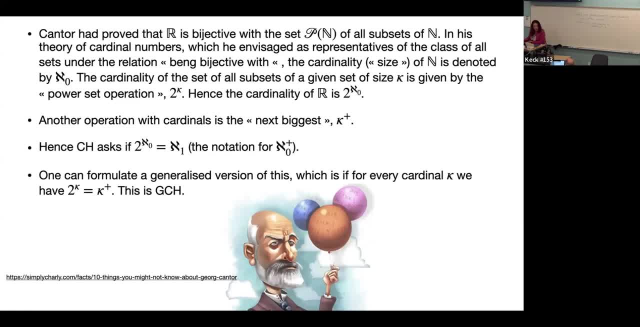 family of all the sets is not a set, so you cannot formalize it in set theory. But this is how he thought of cardinals and the good news is that, thanks to von Neumann, we have the notion of a cardinal. that's differently defined, but it has exactly these properties. 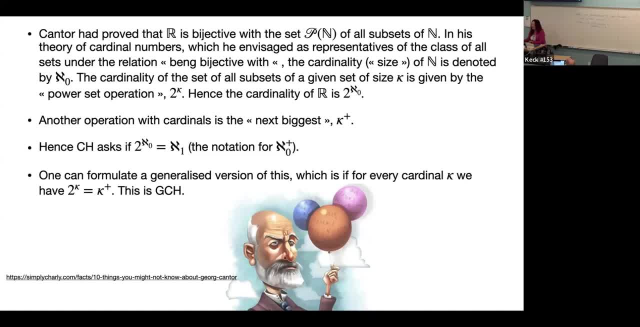 So we can informally think of cardinals this way. And so he defined the notion of the cardinality of a power set, of a set. and if the set has cardinality kappa, then the power set is a set. It has a cardinality 2 to the kappa and this cardinality is strictly larger than kappa. 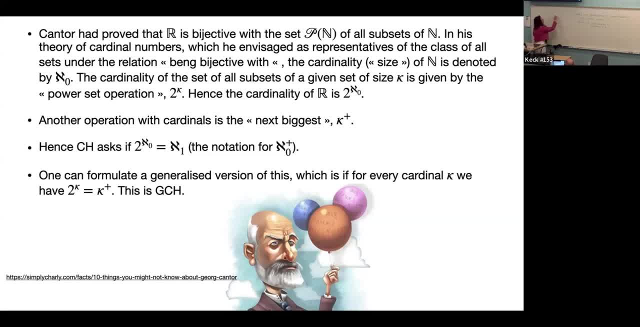 So this is in fact, this comes from this diagonal argument that no set is bijected to its powers. And what does the strictly larger mean? It means there is an ejection from this set to that set, so from kappa to the power set of kappa, but not vice versa. 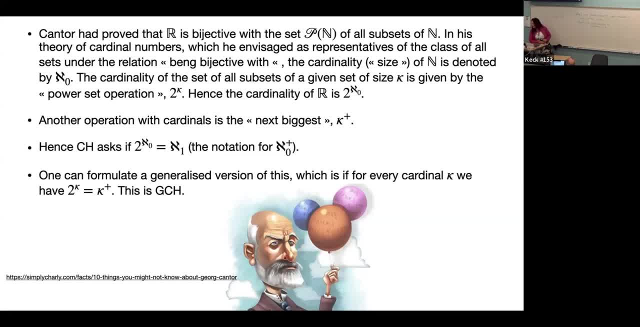 Then he also introduced another operation on infinite cardinals, which is the next biggest cardinal. So this shows that after every cardinal there is a bigger one and by different arguments One can see the cardinals are well-ordered. He has this argument, which is usually given. 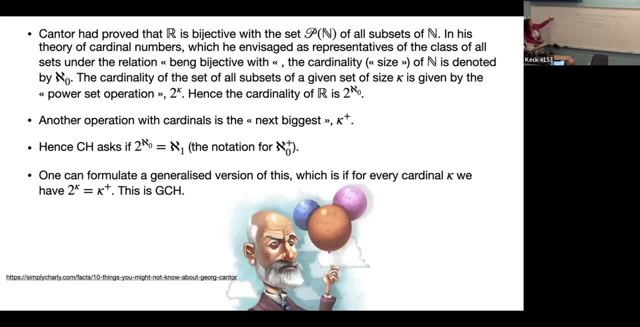 better for it. So there is the first one, which is bigger than kappa, which is called kappa plus, or kappa is less than kappa plus, and then one could ask: what is the relation between those two? And in the specific case of the continuum hypothesis, 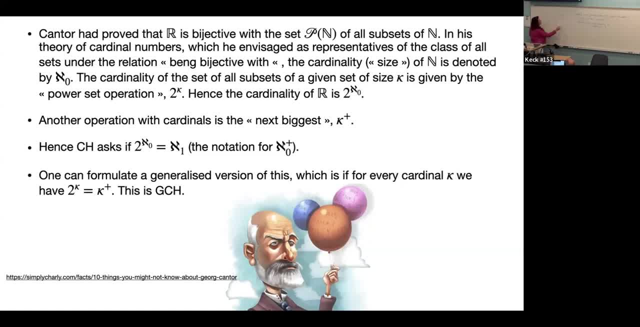 we can look at the relation between Aleph zero- the cardinality of n, the 2 to the Aleph zero- the cardinality of r, and Aleph one, which is the next biggest one, And the hypothesis is that these two are actually the same. 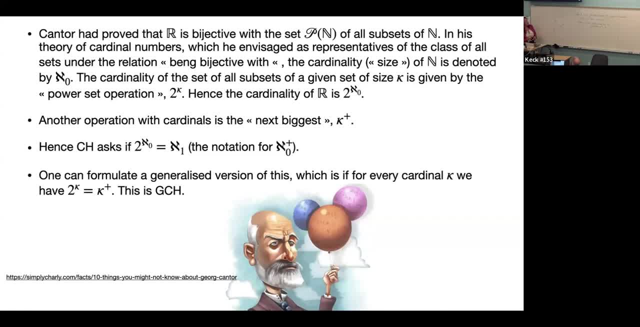 And then, of course, we can formalize this hypothesis More generally by saying that for every cardinal kappa, these two are actually the same. So that's reasonable. but why would he actually think of? why would he find that this was? 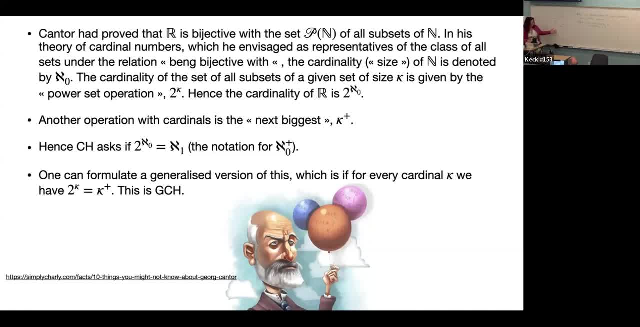 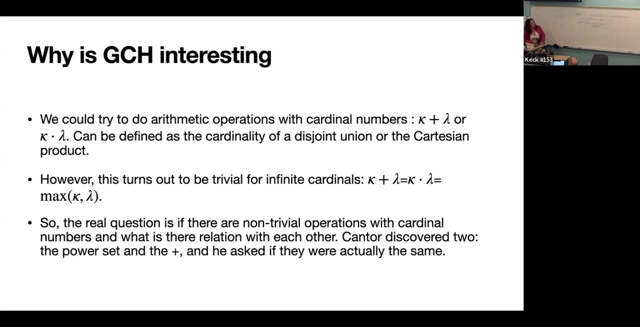 actually natural to have such a hypothesis. Why would we think that two very differently defined operations on cardinal numbers give us the same thing? Well, the thing is that we can try to do it in the same fashion with the cardinal numbers. We can try to do it by doing arithmetic with cardinal numbers. So when people discovered 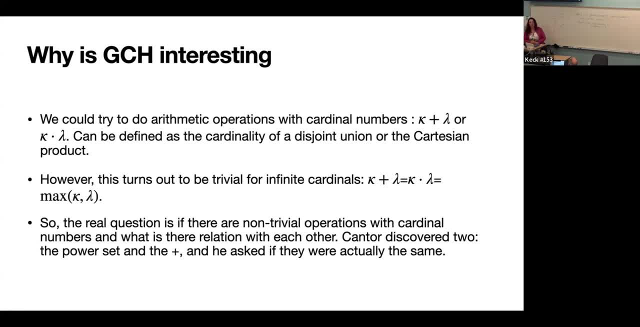 these infinite numbers, cardinal or ordinal, they tried to treat them as we treat any numbers. So one thing is to introduce an arithmetic sum. So in ordinal numbers it's actually quite involved and there are many things we can say about that. On cardinal numbers: 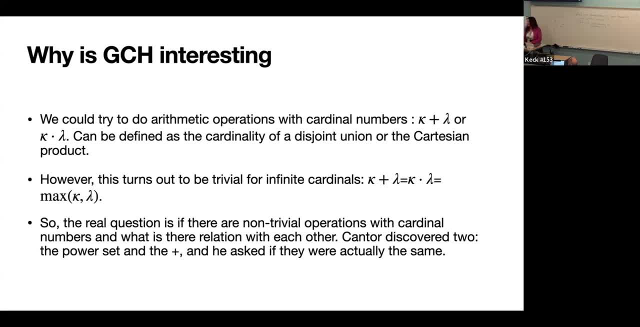 you cannot say much about the arithmetic, That's because it happens to be The sum of two cardinals, is the disjoint union of two sets with those cardinalities, as you would with finite numbers. And for infinite cardinals, kappa plus lambda just turns out to be the bigger one between kappa. 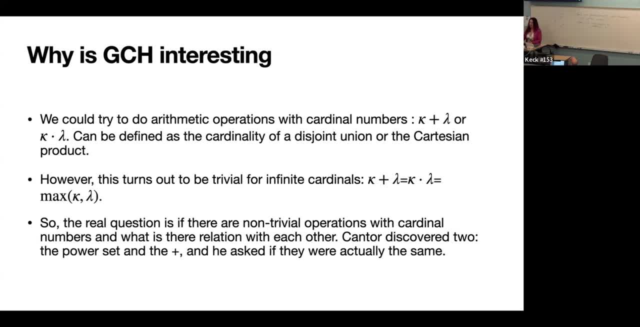 And you get the same thing with the multiplication. So if you define kappa times lambda as the cardinality of the Cartesian product, then you still get maximal till kappa. So the real question that was not formulated in that way by Cantor, but this is really the real question which I'm sure that he was interested in. 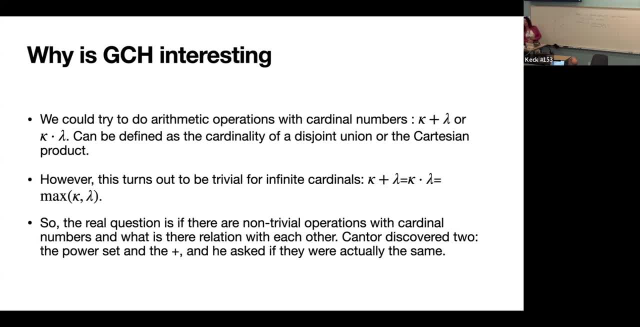 is, is there really a non-trivial operation with cardinal numbers? So he found these two non-trivial operations and, with the experience of the second point, reasonably asked if these two actually are the same, so that we only have one, One non-trivial operation. 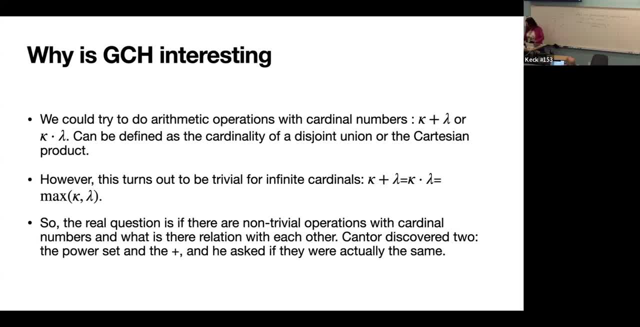 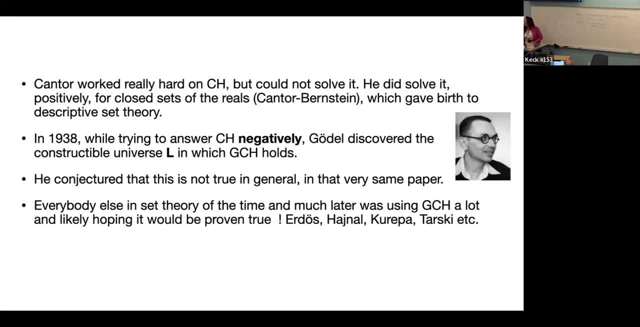 So that's why he was interested in the generalized continuum hypothesis. Now he worked really hard on the continuum hypothesis and couldn't solve it, But he did solve it positively in a very important class of sets. He showed that if we have infinite close-upsets of the reals, 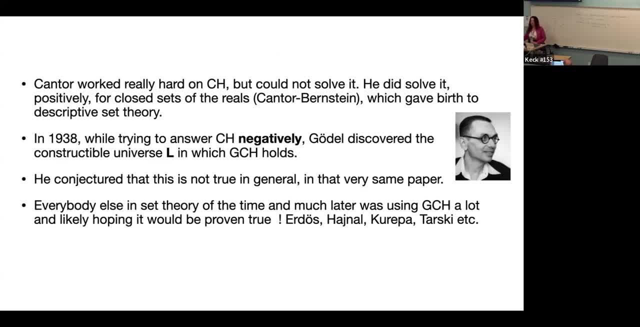 they behave, they do obey the continuum hypothesis, So each one is either countable or has the full power set size. And this is the Cantor-Berstein theorem, very beautiful and deep theorem that started the field called descriptive set theory. And so, many years later, 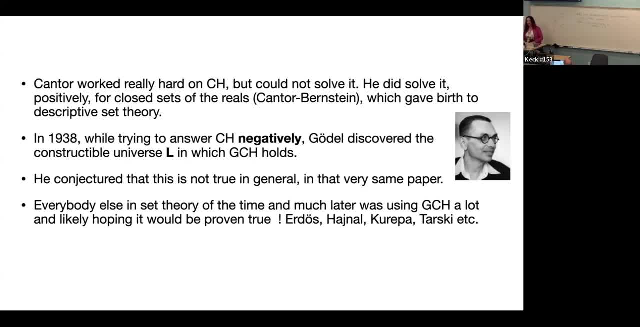 this theorem was extended to more complex parts of the Borel hierarchy and then extending them to bigger, more complex things like analytic sets, projection sets, leads to some accurate consistency theorems with large cardinals. So you see that this thing that seems very simple. 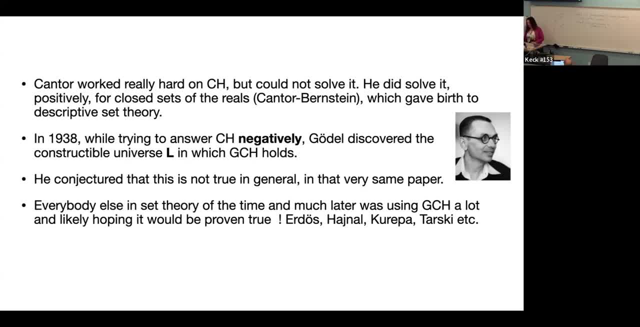 when it comes from very natural constructions, actually can lead to a very sophisticated set theory. Okay, so then he wasn't obviously Cantor the only one wanting to solve CH. So in the 1930s people managed to solve some important problems. 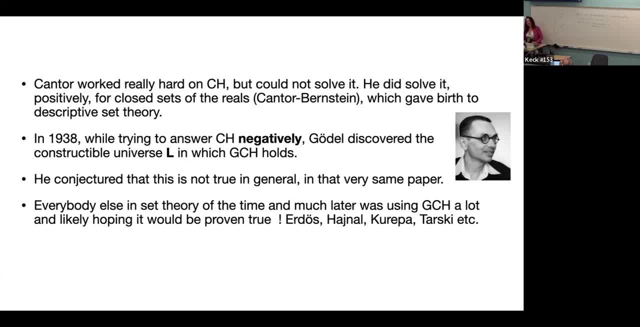 the solution of Turing the Hilbert problem. killing the Hilbert problem. Turing did kill the problem which asked to show that every mathematical process is algorithmic. So there was this enthusiasm about solving all guys' problems. I don't know if Gödel was influenced by this enthusiasm. 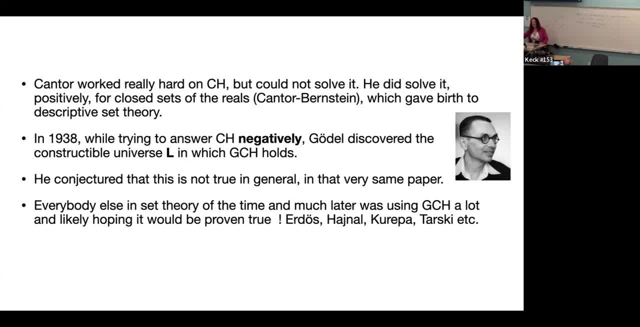 but he was very enthusiastic. He was very interested to show that Cantor was wrong And this is something interesting that also people do not often know- that Gödel was not interested or did not at all believe CH was always true. He actually started working on trying to find. 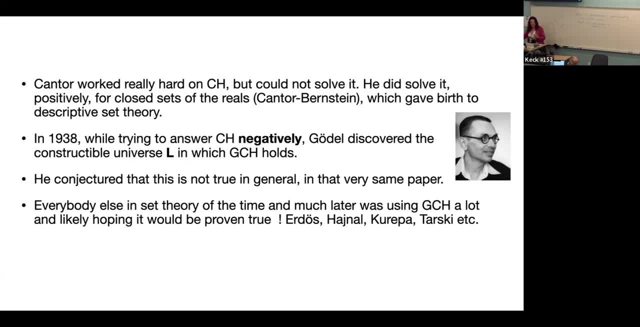 to show that CH is not true, But in this, as he says at the end of his paper in German that this is, he believes that this is the case. but, however, what he discovered is the constructible universe, so a model of set theory. 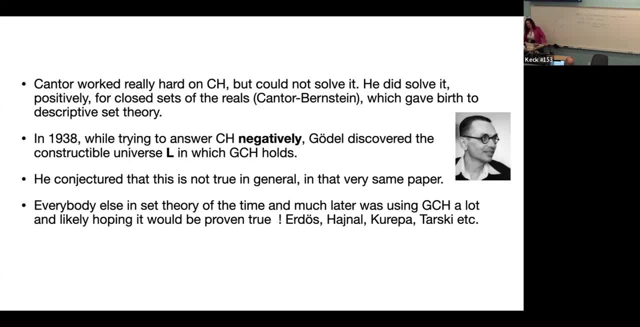 it's a set theory in which the generalized continuum hypothesis is actually true, And so, interestingly enough, Gödel was one of the very rare ones. you mentioned how rare it was at that time to make distinction between a constructive mathematics and existential mathematics. 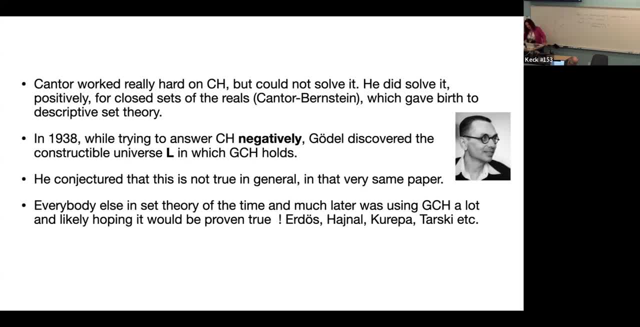 and how we show people there on that philosophical level of understanding. I think that this is also true of the generalized continuum hypothesis, because it seems, by looking at the work of many important mathematicians from that time, that they really assumed that Ante Hades would be proven true. 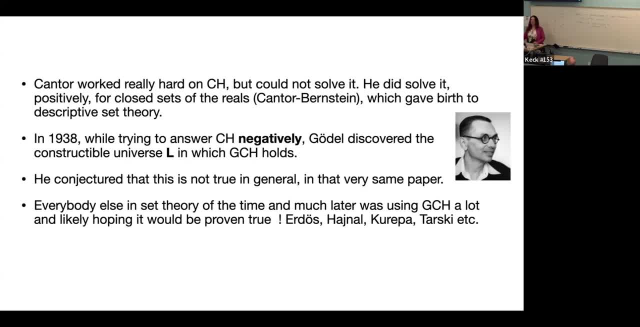 And Erdos, like Steve Nelson happens to know, have known Moinal Ureta. all of them produced papers in which they used GCH very much so, and GCH gave them very nice results. So, for example, the position theorems. 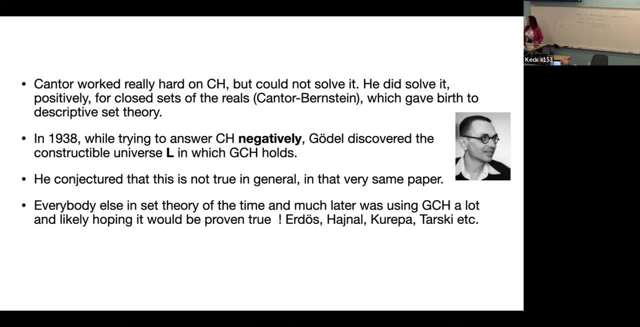 in set theory of the time. they really depend on GCH. Tarski worked in model theory but many things in model theory are much nicer if you are in GCH, So people really thought it would be proven true and well. 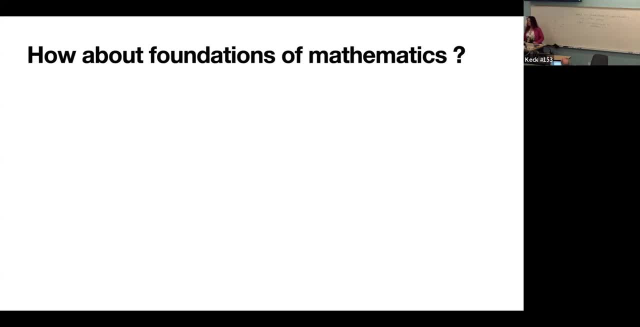 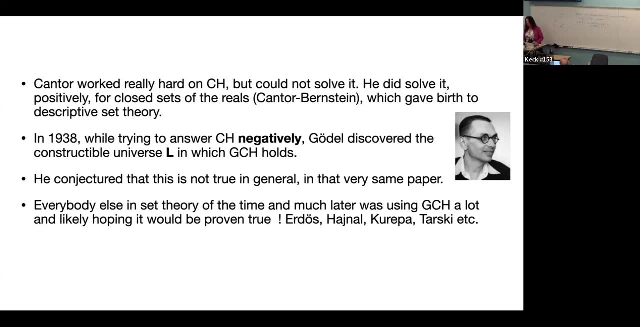 how about foundations of mathematics? So you mean that the generalized continuum hypothesis was pervasively used before Coyle? and proof of independence, Indeed, Indeed. That's what I mean, Yes, And so how about foundations of mathematics? Well, 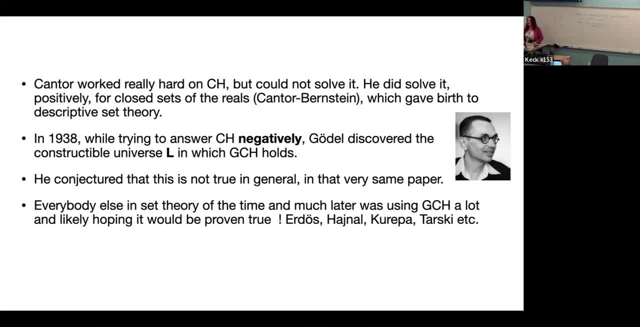 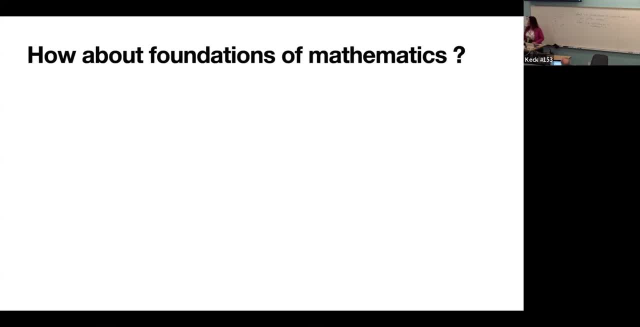 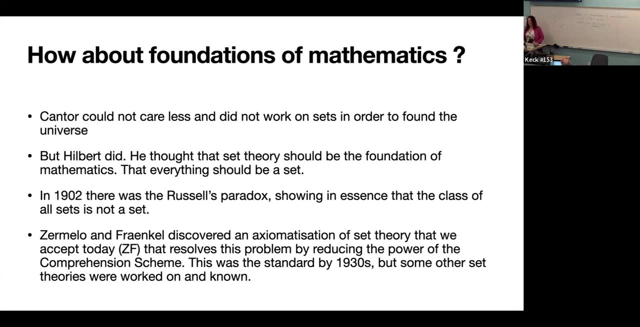 again another thing that may be only good or thought about very, very deeply so at the time, but let us just think what Cantor really thought about this. In my opinion, Cantor couldn't care less about foundations of mathematics. I do not think that this was his purpose. 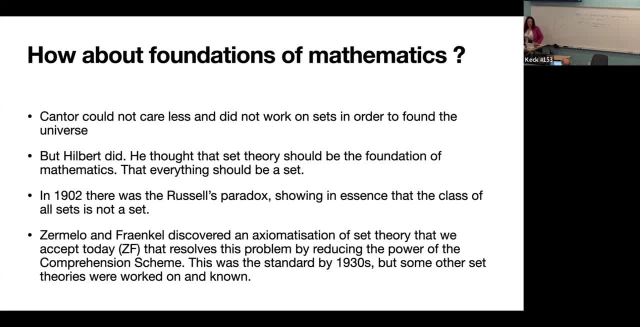 He was very much a mathematician, So one can be a mathematician and philosopher. I think Hilbert was both, and this was probably the strongest point about Hilbert: that he had a philosophy that was leading him to discover new directions in mathematics. 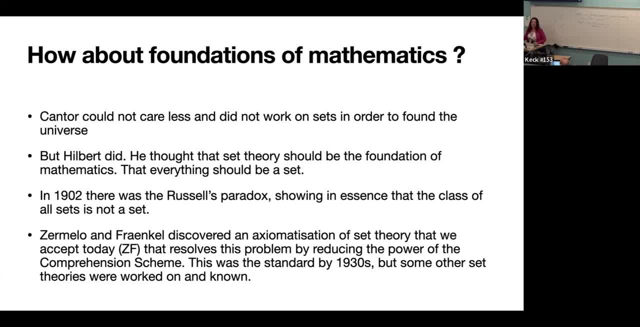 And that was actually Hilbert who made sense theory a subject in philosophy, That is, that's Hilbert who had this idea that sense theory should be foundations of mathematics. Cantor clearly, of course, realized that many objects, maybe all the mathematics of the time- 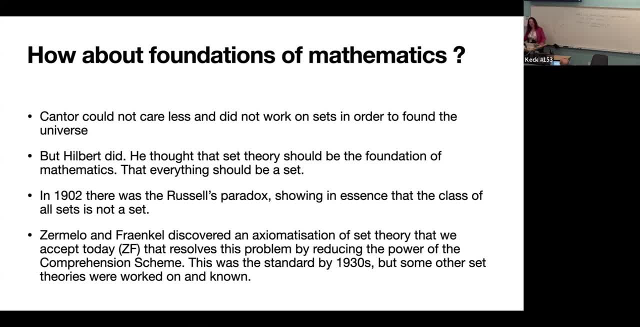 was expressible in terms of sense. But that's a big leap from that to say that the foundations of mathematics are given in terms of sense theory. But Hilbert was very much into this And, as we know, in 1902, when Russell did this paradox. 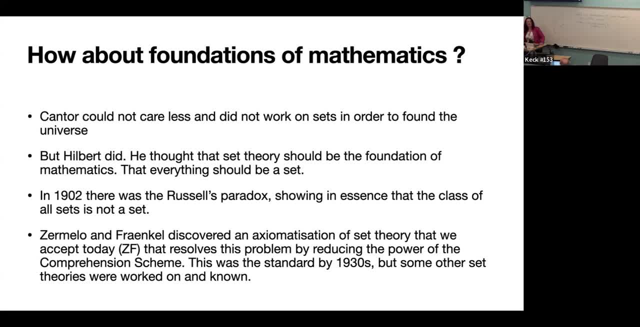 that was evolved in the next, in the previous talk. Hilbert's answer to that: well, you know, nobody should take us out of the paradise that Cantor has created. We should just work harder and fix this problem, And indeed, 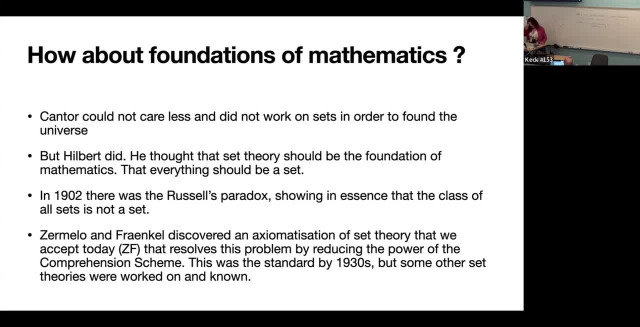 that the axiomatization that was developed by Sir Norman Frankel, today widely accepted axiomatization, is not a problem. It's a problem And it's a problem, And the problem is that the axiomatization that was widely accepted. 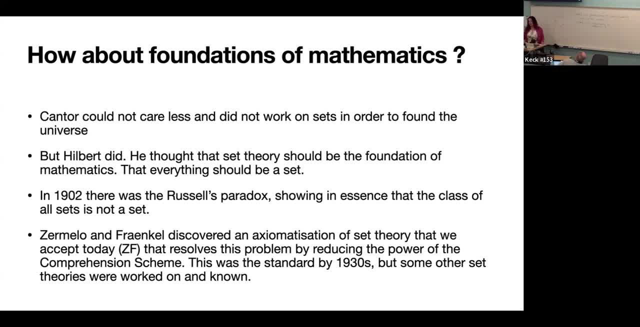 axiom iterations resolves the problem by reducing the power of the partial scheme, which was exactly the point that Mark was making by showing us this proof of Cantor, given in that term, in those terms. So this is how sense theory kind of introduced itself into the foundations of mathematics. 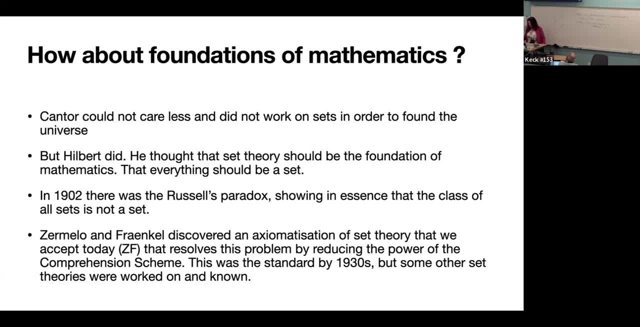 as a- well, I would say as an accidental history. This was the time that people looked for foundations of mathematics and deceptively looked like a choice, Sorry. when, where, if you remember, Ilberto expressed his idea that sense theory. 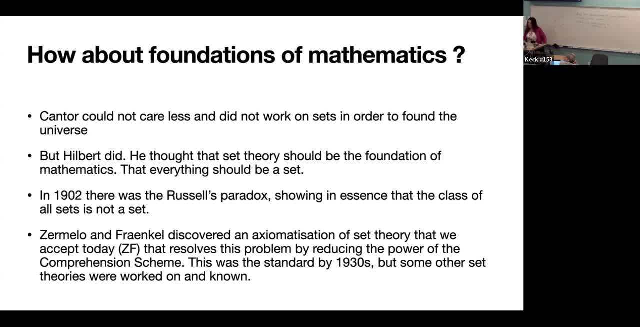 could be used as a foundation of mathematics. what do you refer to it? Well, so he said, nobody should take us out of the paradise that Cantor has created, And his first problem on his list is generalized continual processes. So this must have been. 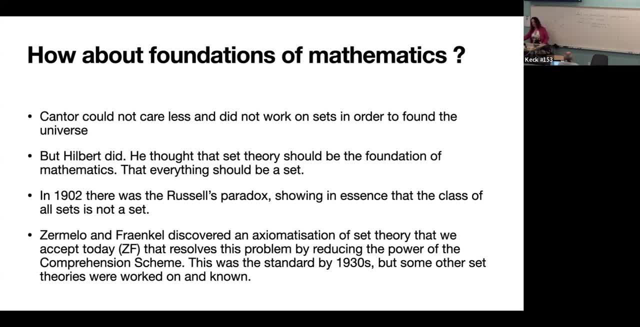 before that that he Anyway. at the same time, I mean, I think that in the 19th he provides, he develops the idea of axiomatic theory, axiomatics for real numbers, axiomatic for geometry. 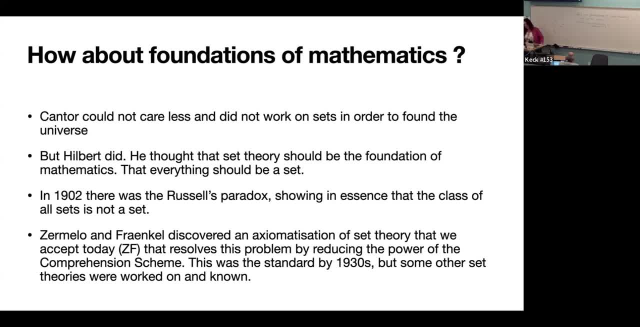 So it's not satirical attitude. Well, so I think what happened is that the first big theorem, recognized theorem of Ilberto was axiomatization of geometry. This was an amazing theorem, So he managed to axiomatize, give a complete axiomatization. 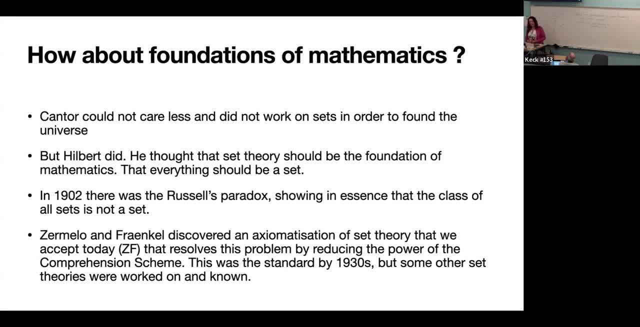 of geometry. So it was a big surprise, a big possibility for Ilberto, And you know, of course, Euclid's axiomatization was so typical, And then he was ambitious, so he wanted the axiomatization of this and that. 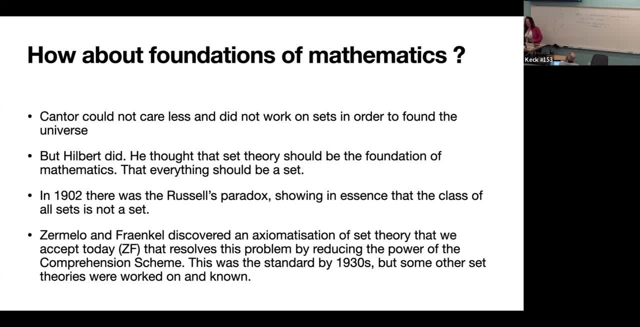 And finally, he wanted the axiomatization of the whole of matter. And so how would you even start? Well, you would have to have objects that speak of the whole of matter. That's how you essentially think. One thing is axiomatize. 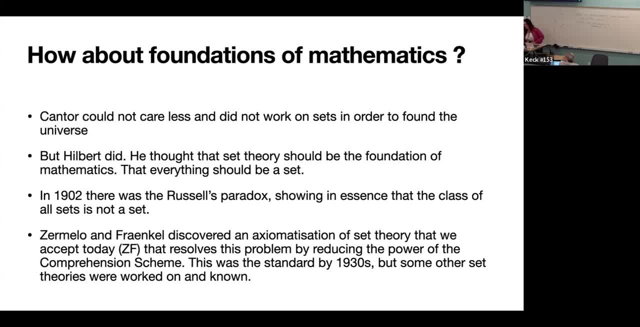 the theory, because paradox can't make a lot of nice things in theory. We want to see the axiomatics that are actually present in the axiomatics. Another thing is to say that we think it's axiomatics that can reconstruct. 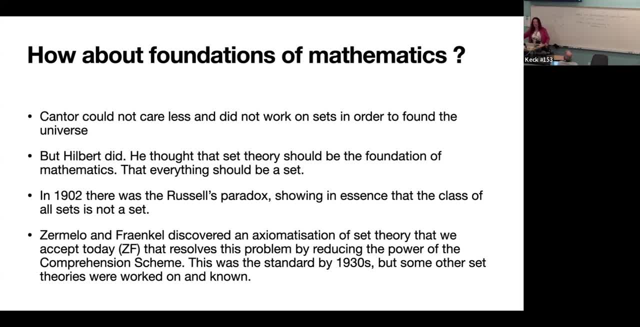 all mathematics. No, this is exactly my point. This is important because in the 19th century people thought differently than we do today. I hope that you think differently. today. There was this idea of expansion, colonizing, doing mathematics, This universal power. 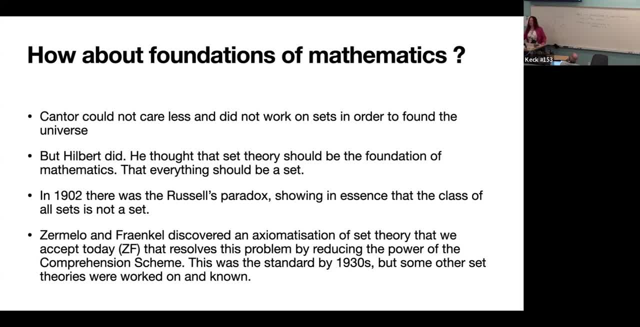 we just have to find it. And you know, when Hilbert was retiring he said in a famous speech: we have to know and we will know. So that was the 19th century idea, kind of romantic idea- that human knowledge can give you axiomatization. 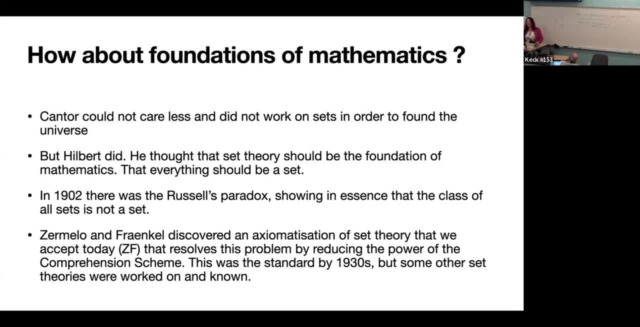 of everything. So, as we know, it has positive and negative things behind it. But in mathematics, I think the Hilbert theory has much an idea of its own time. I think. well, I wonder if anybody, if we didn't have Hilbert in the 19th century? 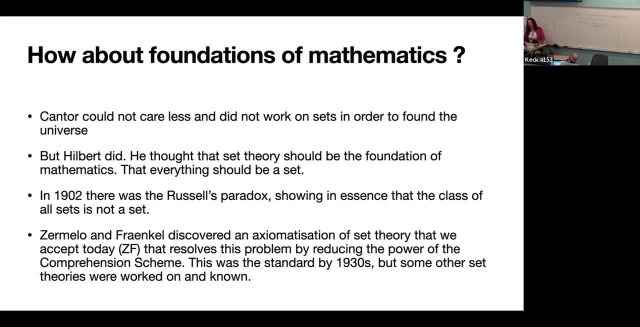 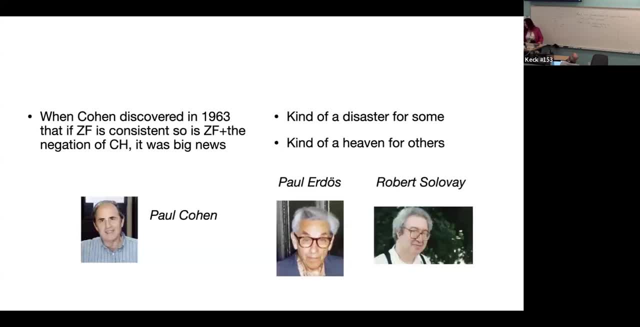 would people these days think that it's possible to find one theory that relaxes everything? It would be different attitude, So yes, So this is, these are the kind of the theories that are the most interesting and interesting and challenging to see, because 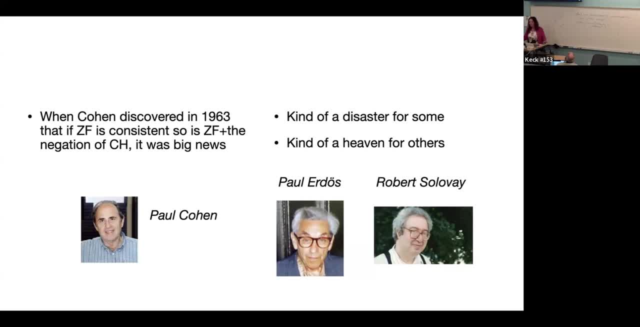 there is a lot of real evidence, but so I would too. My last book came in 1995, so just shortly before he died, maybe a few months- and he said: do you really understand forcing? And so he somehow felt this was very puzzling to get. 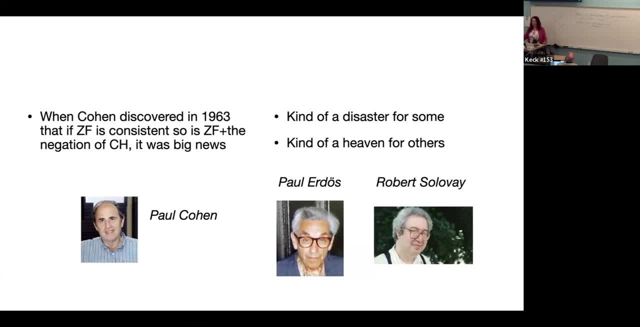 independence. Of course he understood forcing these simple combinatorics and things that he do in history. but yeah, what he didn't really didn't agree with is this idea that you need to have philosophy, and logic was kind of philosophy. Then other people, of course. 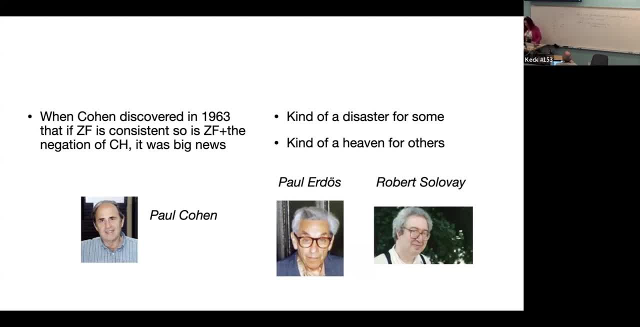 thought that it was a heaven, and young Robert Sullivan learned about forcing and then made it his own and made fantastic theorems in set theory starting from that point. And so forcing was big news in set theory. and so what does forcing do? Just to, 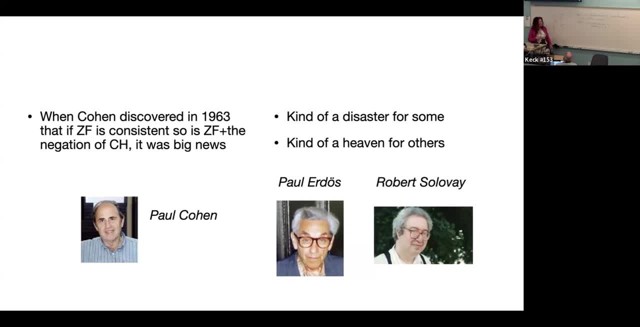 recall the picture. so the following forcing does the following: You start with some transitive model of set theory, which has to be countable and not transitive, And then you extend it in a very clever way to some somewhat bigger model which is called m of g. Let me just picture actually That. 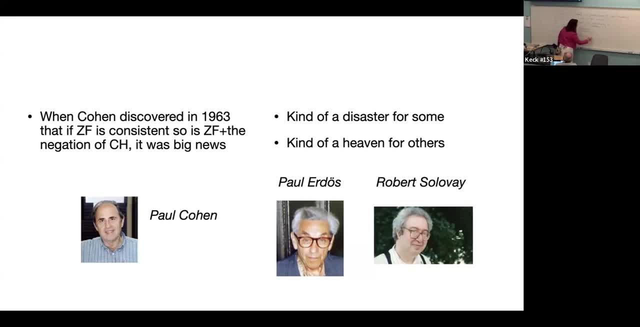 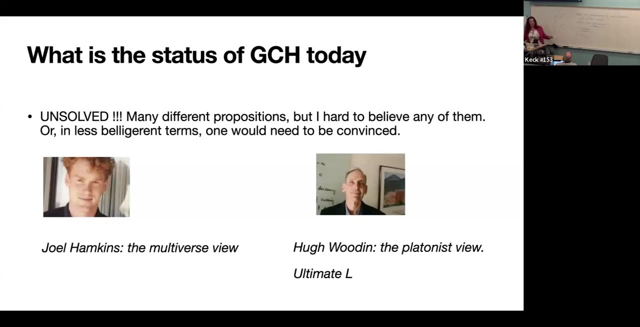 satisfies the same amount of set theory plus whatever it is that you want to satisfy, if you are lucky. So let's say the negation of the continuum hypothesis. So that's what forcing is. And well, so if CH is independent, this means GCH is also independent, of course. 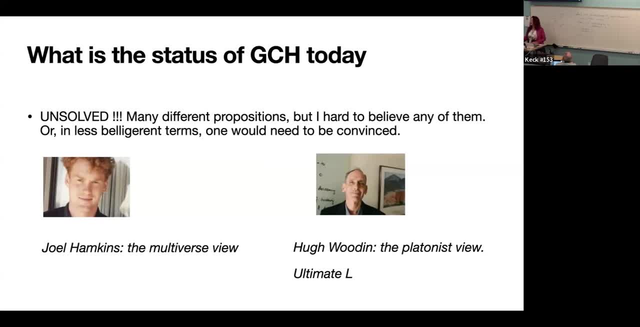 because if you value CH, you value GCH, And what I would like to talk to you about now is: what about the state of the set theory? What is the status of this GCH today? What do people think of this? Was this the solution? 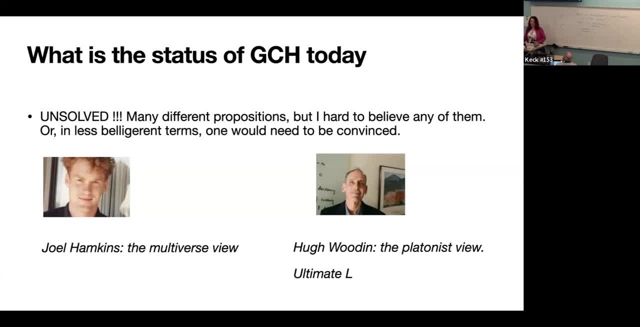 that there is no solution? Or should we work harder and find another solution? Or is this problem even interesting? So what is the status of this? So let me just say a few things about things that we already know with points time. So people worked a lot on large cardinals. 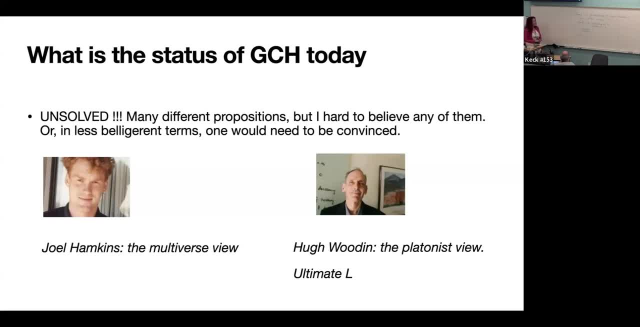 So what's a large cardinal? This is a statement. Actually, a large cardinal is not a cardinal, It is a property, And it's a property of the form p of kappa, not p with the form phi of kappa, such that Z cannot. 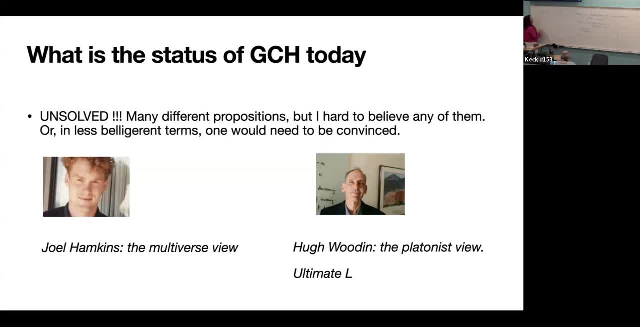 prove that there exists a kappa, such that phi of kappa is true. So a simplest example of this is an inaccessible, strongly inaccessible, cardinal regular limit, cardinal closed under the power set operation from below. Why can't you prove that this exists? Well, that's too. 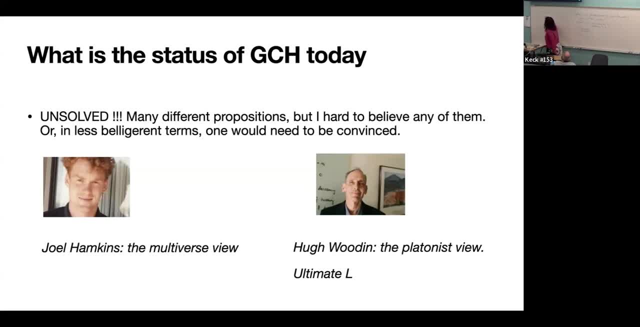 good that we can state such things, because if you had a kappa strongly inaccessible cardinal, then when you look at the cumulative hierarchy you have kappa notation. then it's actually a model of ZFC. It's a set, a model of ZFC, And ZF cannot. ZFC cannot prove that there. 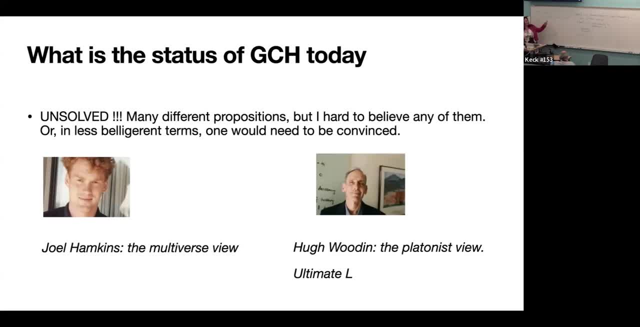 set model of Z, of C because of Guido, so that's why we cannot prove such thing. So then there is a whole plethora of large cardinal axioms, properties that become stronger and stronger and stronger. so you might think: well, since they are so strong that they can prove the consistency. 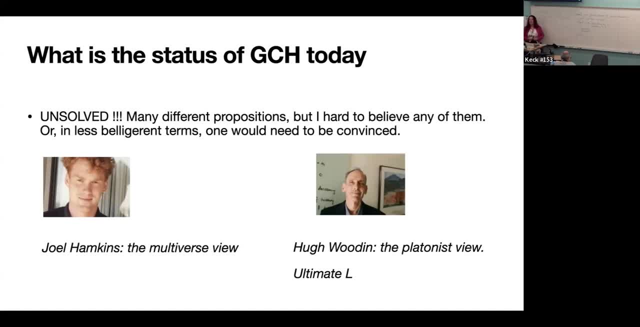 of Z, of C, maybe they can solve ACH, And actually no large cardinals do not solve GCH, because Levy and Solovey proved in the 60s, very shortly actually after this Cohen model, I think 1967.. 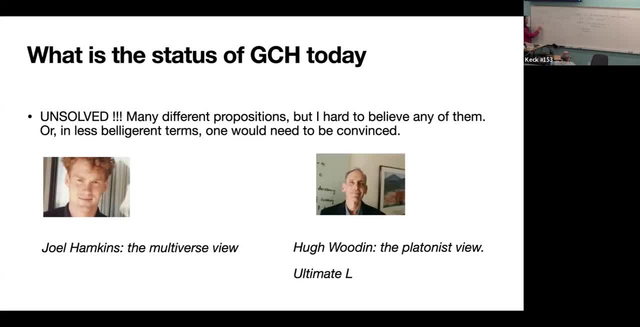 So what they proved is that if you have, for example, a measurable cardinal for consistency of that exist, a measurable cardinal implies that it's consistent that there exists a measurable cardinal And not CH, and also with the positive, so also with positive. So this means that the measurable cardinal cannot decide CH either. 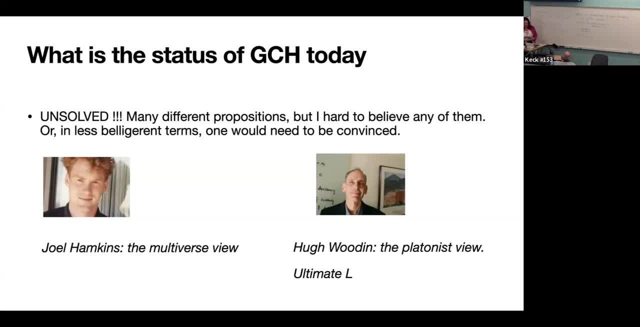 and this argument can be repeated in basically any large cardinal axiom. So this is not the way to go. So what is the new wisdom on this subject? Since the time, people haven't given up. So some people have given up, some people haven't given up. so let's look at some propositions. 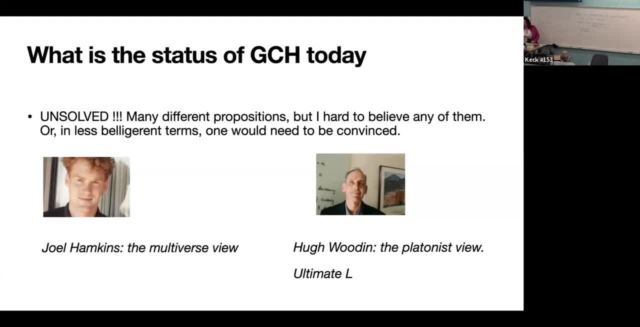 Okay, so here I have pictures of two mathematicians, Joel Hamkins and Hugh Wooden. I must say I took a picture from Joel and he was very yummy. I liked this picture. How much time did you take for taking a picture of two mathematicians? 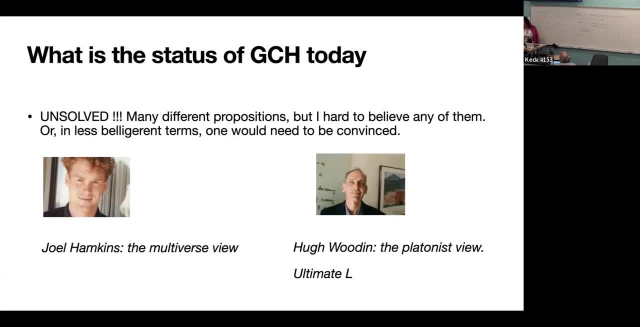 Graham, I didn't have a photo. How long did it take you to take a photo of two mathematicians? How much time ago- I think this was at least that year- I wrote the joint paper with Joel in 2001, and he looked exactly. 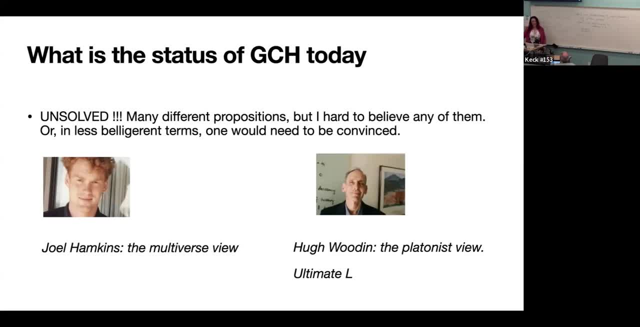 at it. So I thought it would be nice to include his face. So that actually was before he started doing- very successfully as he is doing- philosophy. So he developed a view of this continuum hypothesis problem, which I think is very interesting. 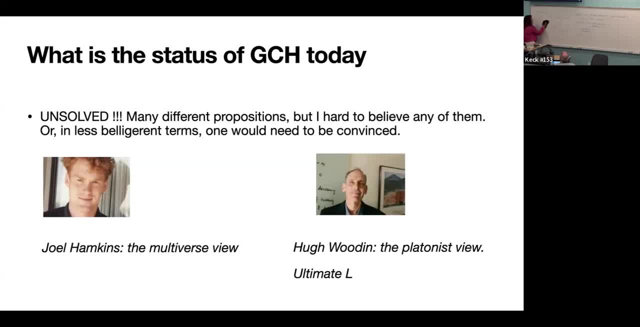 very unusual and somewhat controversial, but this is philosophy, so I think it's okay to be controversial, Otherwise it was too boring. The philosophy student here perhaps forgetted it. Yes, you have to think like Marco Paz: Absolutely not, absolutely not. but you should try not to be questionable then. 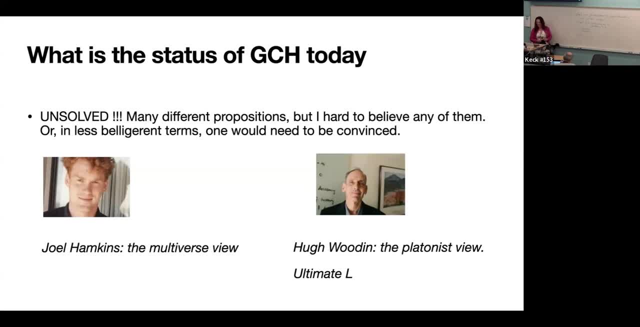 It's very difficult, but anyway, not to be questionable. It's controversial, it's a name that you cannot reach, but you have to tend to it. Yes, so what are the classical positions in the philosophy of mathematics? Yes, so one could have some people go in and explain the details of the work. 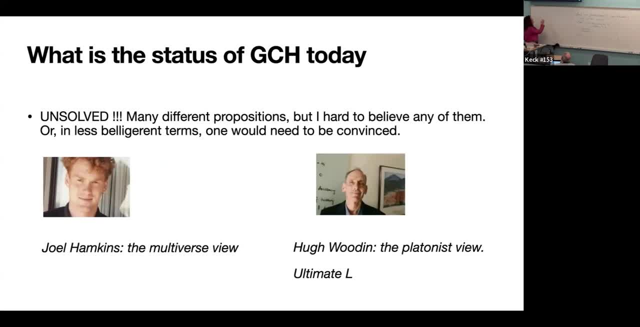 we could think of. well, there are many positions, but one important one is Platonism. Well, I think it is on Platonism that belief or non-belief of Platonism- that satirethic controversies rely on. So let's just recall, Platonism would mean that there is 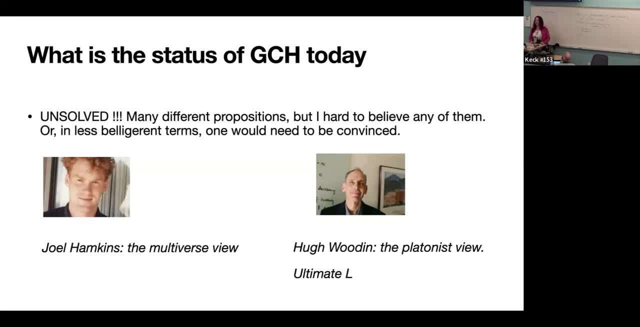 in this context would mean that there is some universe of all the sets, and in this universe of all the sets, the truths of all the statements are known. So there is this. we imagine that somehow there's V, and this V knows the truth. and well, we try to find that that's Platonism. 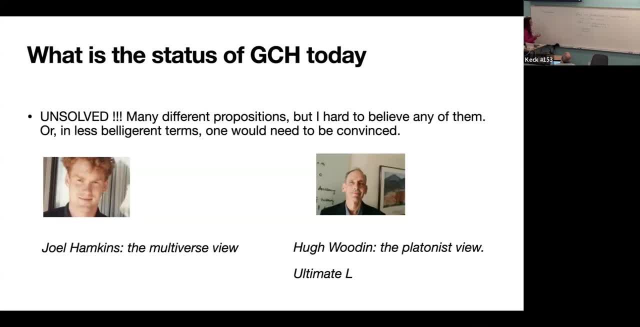 Now Joel's view is the following: No, this is not what I believe His view is what people would call the Platonism. Now Joel's view is the following: No, this is not what I believe His view is what people would call the Platonism. 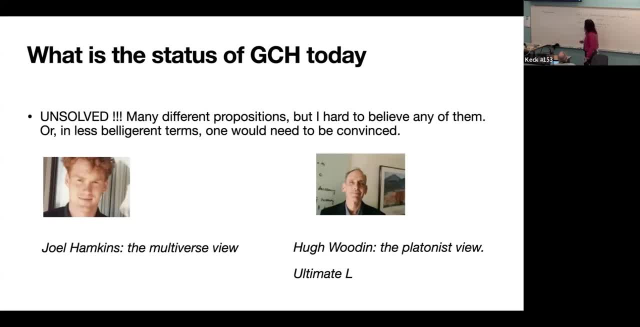 Now Joel's view is the following: No, this is not what I believe. His view is what people would call the Platonism. So he says: no, I have this method of forcing, So I have not one universe. 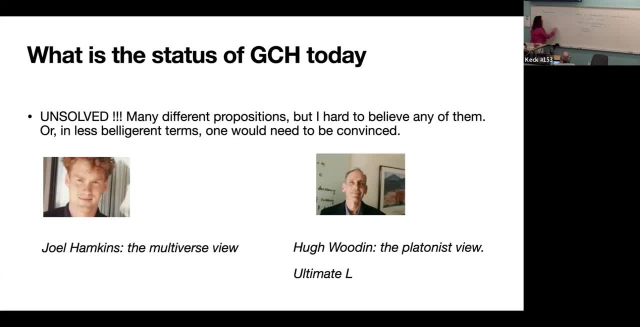 but I have many universes and in these many universes I can do many forcing extensions. They look like that and then maybe I can duplicate that. So I have tons of different universes of satirethy and they do not agree at all on the values of Platonism. 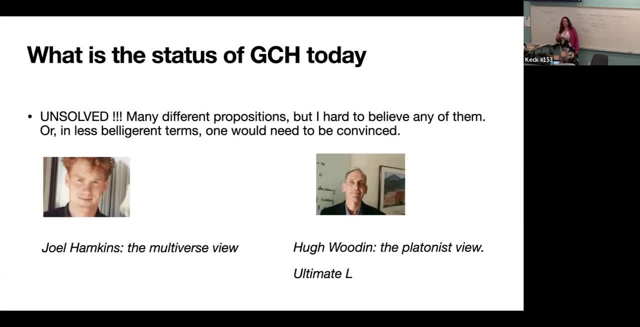 of the continuum. In some of them the continuum hypothesis is true. In some others the continuum hypothesis is totally false. But then the value of how false it is, it differs. So what he states in his very cited paper on the multiverse of Satyug- so this is the multiverse- is that it's? 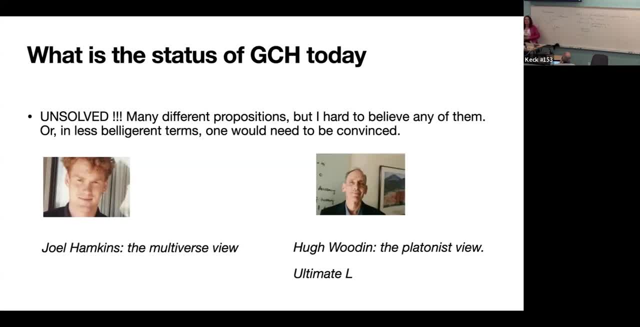 actually this multiverse that gives the truth. So this is, I think, a very 21st century vision. We don't have the truth, We have votes on the truth. So you know, everybody can vote for the continuum hypothesis And we are not looking for some agreement. We are not looking like in the 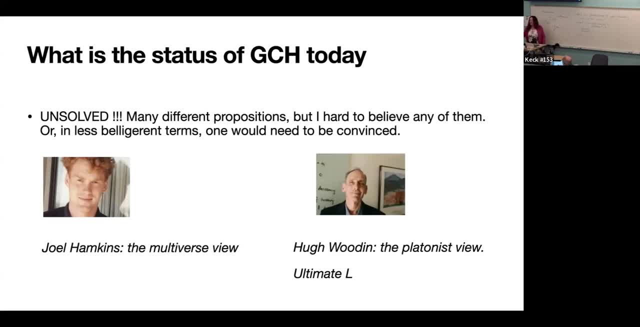 classical voting problem to find the winner. No, we just know. well, you think it's our 13,. I respect that. We are not looking for some agreement. We are not looking like in the classical voting problem to find the winner. No, we just know. well, you think it's our 13,. I respect that. 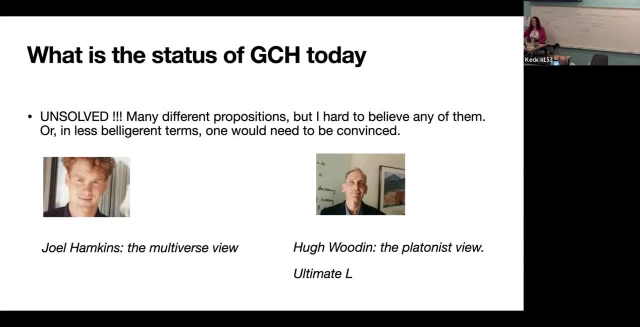 your opinion. I actually think it's our 15. But it's not a bad view to have, I think, in many, many situations. You may consider what you think of it in this situation. But there is one reason. This is very clearly explained in this paper, but most people who read this paper do. 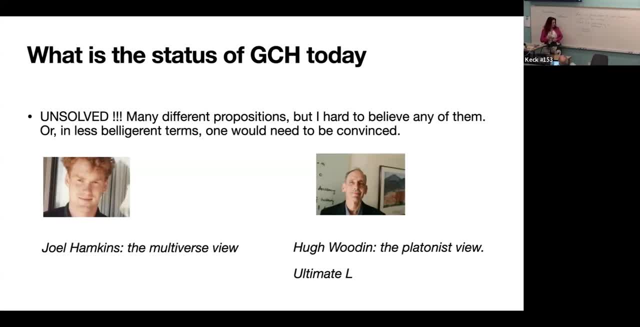 not notice this. For this method to work- forcing- you don't start with a considerable transitive model which lives in thin air. This model actually has to live in some outside universe. So even to do forcing you have to have outside universe, Otherwise there is no forcing. 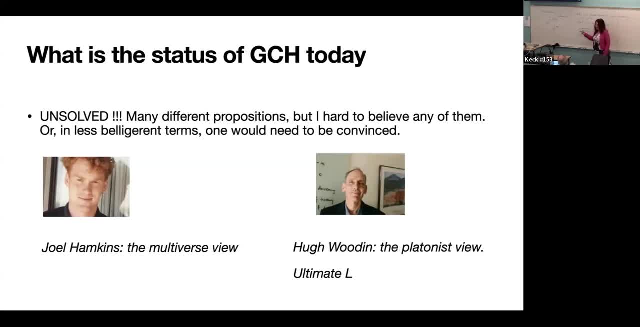 So what is the outside universe for this? Is it one? Actually, in the paper there is one outside universe, And then inside of it we do these things, And then inside of it we do these things, Because there are more than one. Maybe the one for this is different, the one for that, But there is. 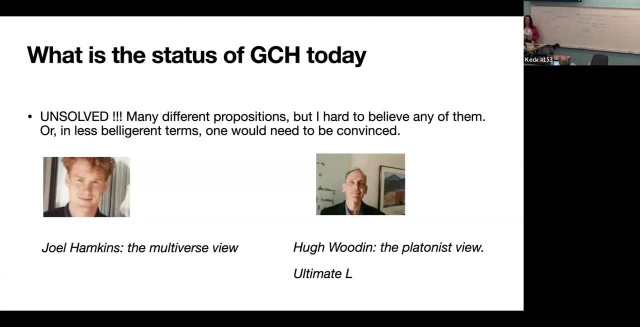 the outside universe. So this is not a complete divorce from data. So can we repeat the other way, That there's something outside the universe? Why? Why? Because the forcing method. just to be able to do this, you have to know that this M actually is inside of some V And you have to argue in V. 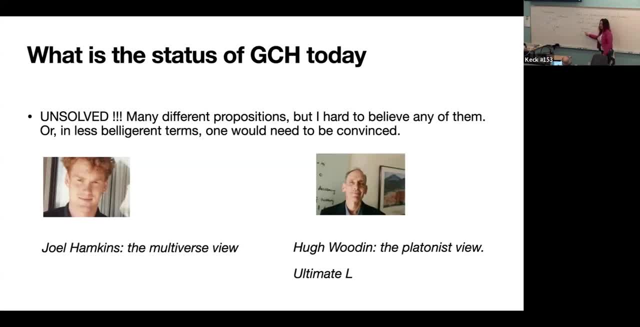 a lot to make this to this, for this to exist, I mean technically, it's because you have to enlarge a model, So it has to have already been a model in something. Yes, to enlarge it to something that exists, Yes, exactly. 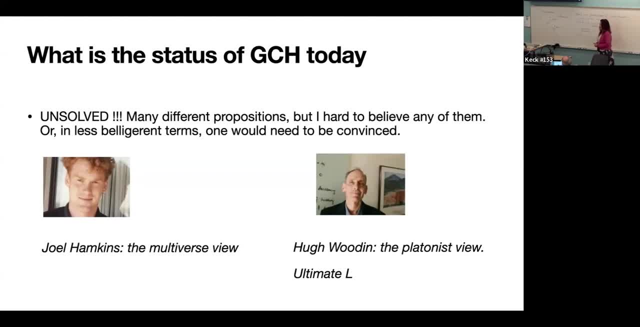 You can put your point the other way around, That if you do not accept that there is something outside the universe, you cannot prove an independence of it. Yes, You cannot make forcing. Exactly, Exactly, So this is So. do I have to be a Platonist to make sense of? 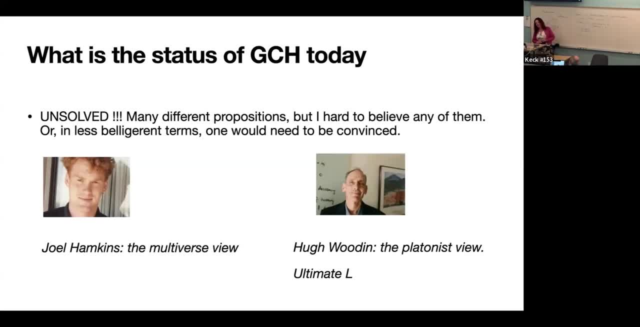 the set's theoretic multiverse. I think, yes, You are a Platonist. Yes, and I think actually it would make some sense. yes, I'm not sure, because you can have opinions about which V you want to use. 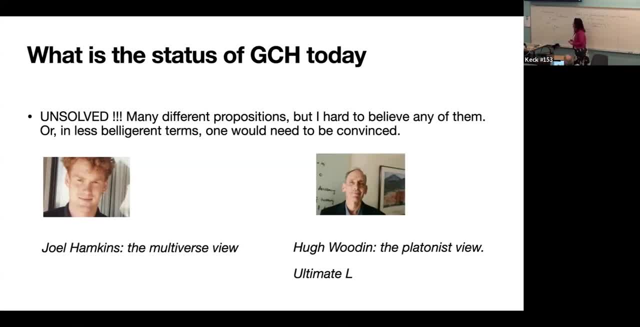 Yes, yes, I think this is the right answer because, actually, what we could imagine? that this one comes from some different V and this one comes from this green V, but then, if you do that, then it looks like you are arguing in a circular system. Yes, If you do that, then it looks like you are arguing in a circular system. 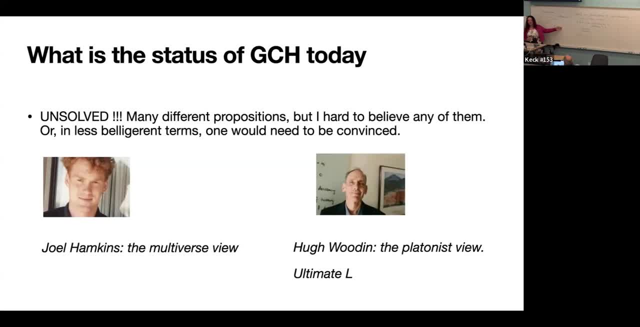 way, because, anyway, you already know that you have a multitude of universes, so then constructing another multitude of universes. Am I wrong? but what you are underlining is that the hypothesis of the multiverse is formulated in terms of models, not in terms. 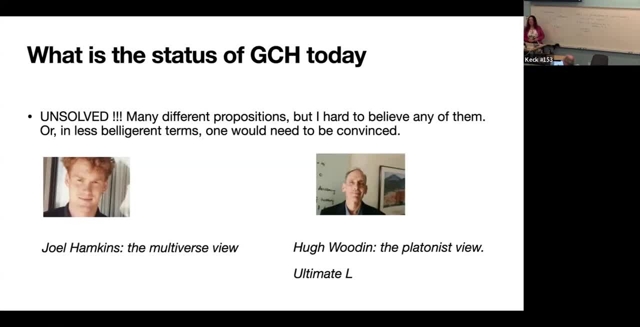 of universe. Okay, and if it's formulating in terms of model, you do not mean Platon. That is not seem to be the goal. No, I think there are two kinds of Platonism. One kind of Platonism is that the structure of our theory constrains models and the other level. 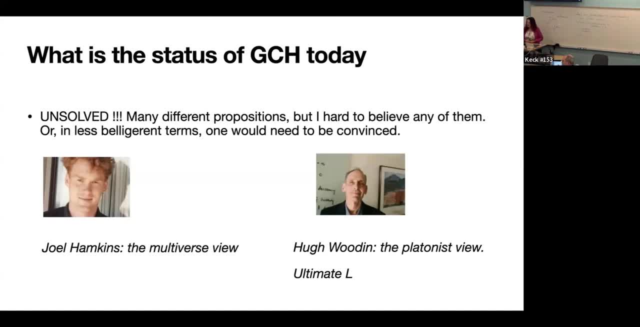 is more radical is that our theoretical structure constrains the universe, which is much stronger. These are two levels indeed. So, yes, there is some Platonism around, but anyway, this is a very interesting question, Thank you. I have a question about the original view, which is not at all shared by Hugh Wooden. 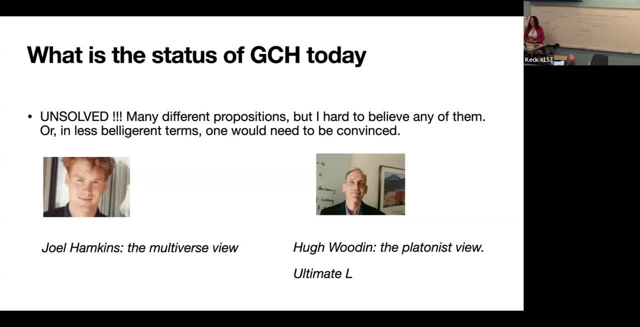 for example, Hugh Wooden has a very Platonist view. Hugh Wooden has done a very important one, one of his loves in his life, of course, but I think they have- and he confirmed this in his book- that they were motivated by this idea of completing the axioms of sexism. So 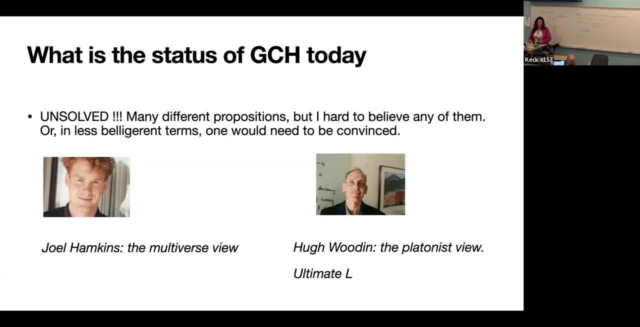 he truly believes that the axioms of sexism are the most important. He believes that there is some completion of the Zermelo-Frankel axioms that will solve the continuum hypothesis. That's not hard, You can just put the continuum hypothesis as an axiom. but that's not what he wants. Something that's natural, that shows up, that. 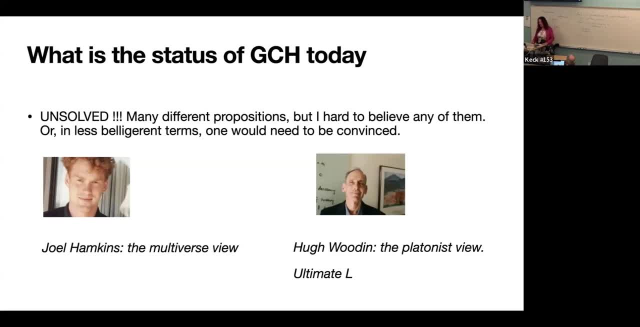 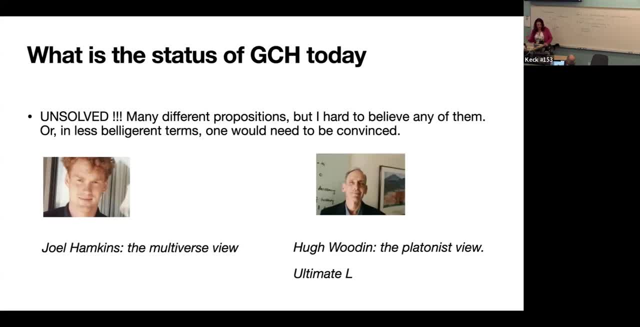 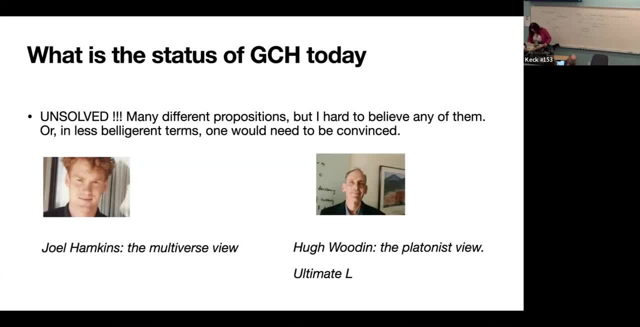 out of several different approaches to this, the one that has been mostly spoken about recently is this ultimate L-conjecture. So what's the ultimate L-conjecture? Well, let me read one paragraph from this paper in 2019.. There's a 109 pages long paper, which 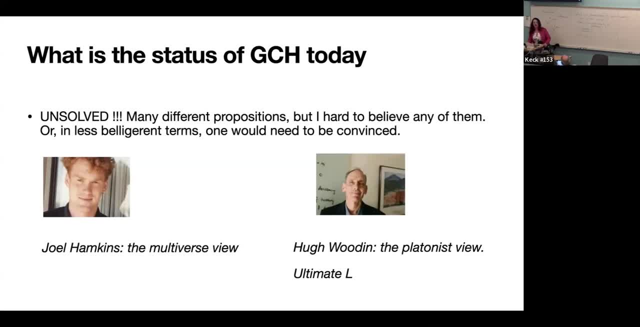 is for children. wel earth kettlebell books put весы account of the situation, of the ultimate health conjecture at the time. Why then we write this account now, before the issues are resolved? The collective impact of all the obstructions which are the focus of this account. 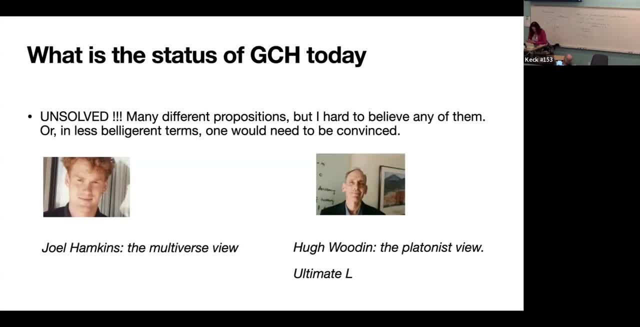 leads us- I paraphrase a bit- to a form that the ultimate health conjecture must take. So what I'm trying to say: he doesn't have the proof of the conjecture, but there is more to it. He doesn't have the conjecture if he is working to find the right conjecture. 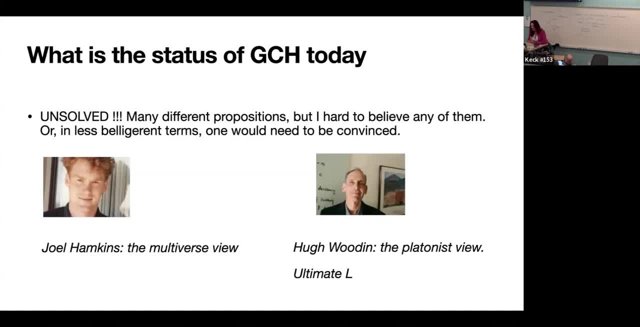 that is the ultimate health conjecture, And it takes 109 pages of deep mathematics involving a set theory. that's very, very pessimistic if you want to even understand what this could possibly be. Well, so I can tell you in two words what it is supposed to be from one point of view, that 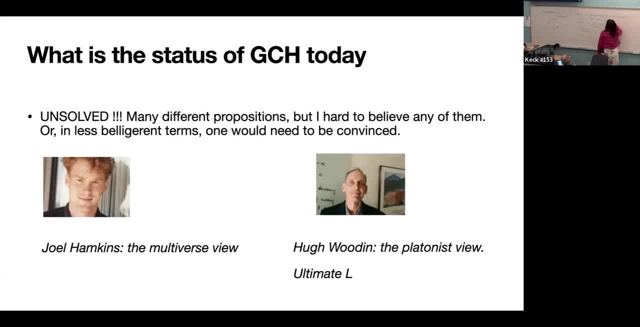 he can understand, and then I will then ask us to think about what's an axiom. Okay, so we have L that Gödel has constructed. L is a lovely model of the axioms of Z, of C. it's resolved GCH, but it's too tight for most people purposes, because it was proven by Scott. 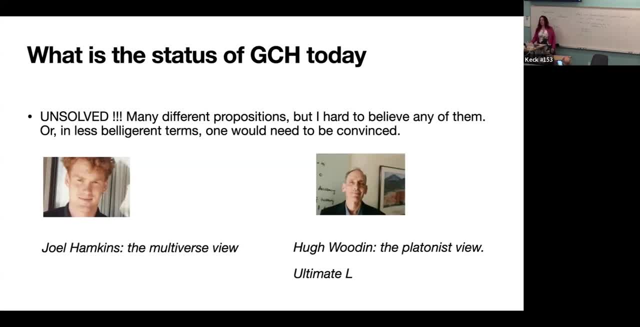 in 1965 that a set theory favourites the measurable cardinal cannot exist in L, So L is well. you might ask why you want to have L. Well, you might ask why you want to have L. Well, you want to have a measurable cardinal. Well, if you don't want to have a measurable cardinal. 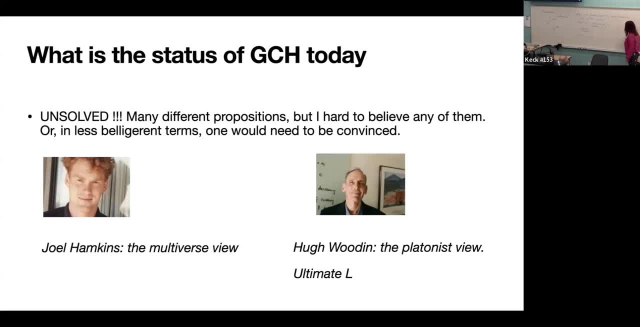 you might be working in L, but most people think that these large cardinals are important in mathematics and so most people essentially think that at least So in L there is no measurable cardinal. So this was proven in 1965.. One of three seminal papers. 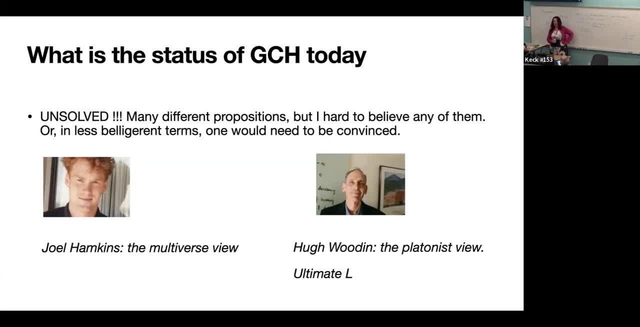 that Dana Scott published in 1965. Amazing quote. If you are curious, you can check this on the internet. He published the proof for Babel-Scotty, and totally different subject. I'm very proud to say this is my grandfather. Okay, so then, what to do is to try to pump up L with something that 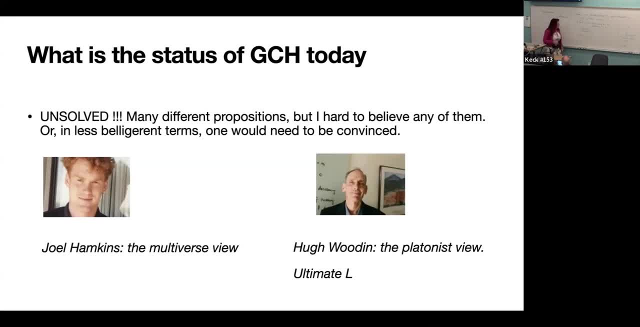 could make it look like it has a large cardinal. L is an axiom of the axiom of the number of points, And the first very important progress on this question was achieved by Marc-Marc Kempunen, who constructed L of mu. So L of mu is basically: you do like this, you start with V? mu side of it, you have L. 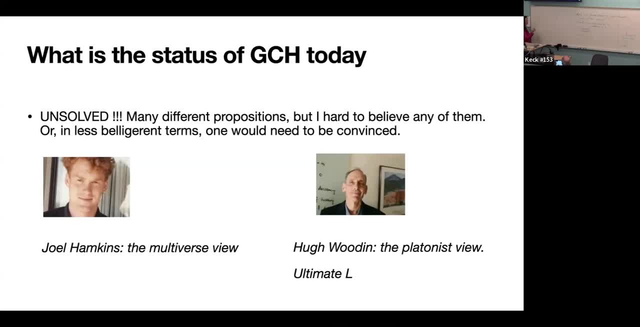 but in V you assume there is a measurable cardinal. so there is some cardinal kappa and on this cardinal kappa there is a measure called mu. A measure is a two-value. it's an ultra filter with certain nice properties. Okay, now you would like to combine these two and he develops Kuhnen. 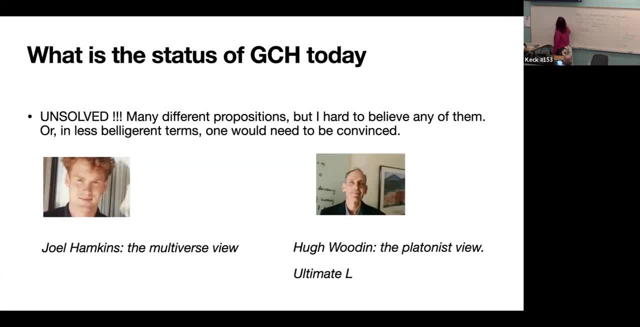 this nice way of doing it and constructing the model that's called L of mu, which is like L, it has some structure, theory and it has a measurable cardinal, because this kappa is measurable in L of mu. Okay, so now you could try to play this game for other cardinals. 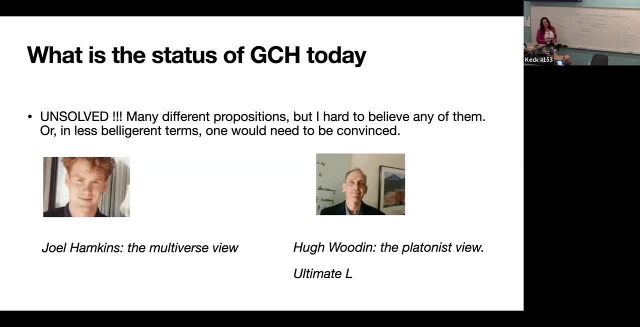 stronger and stronger cardinal notions and you come to the inner model theory, which is a big problem, which attempted to construct models of this type for larger and larger cardinal notions And there seems to be the. actually, there probably is kind of a limit of how far you can go. 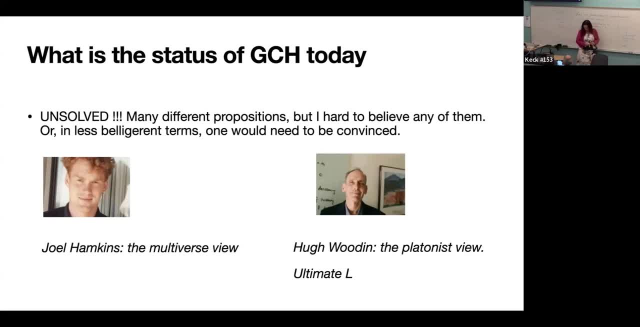 There's a paper from a few years ago by Steven Jensen, who gave this limit in terms of some number of wooden cardinals. At the compact limit there are super compact cardinals. So what are wooden cardinals? Wooden cardinals are defined in terms of some. 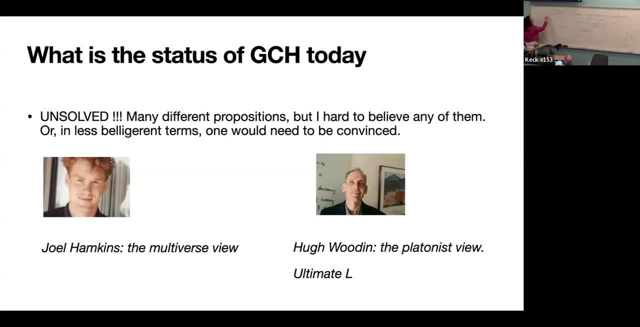 combinatorial property. They are not very strong but the strongest to have a measurable limit of wooden cardinals And this gives to wooden. there are many theorems of wooden that under these circumstances can prove a nice theorem, For example that consistency that the AD volts in L of R 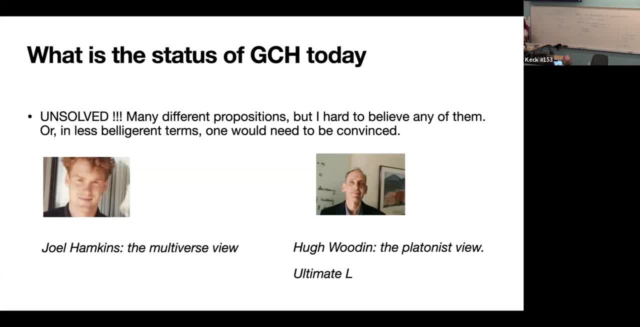 So that's why they're important. But above all of them there is the super compact, which is kind of a pumped up version of measurable, Very useful in set theory everywhere Considered. kind of high end of this business And above all of that. 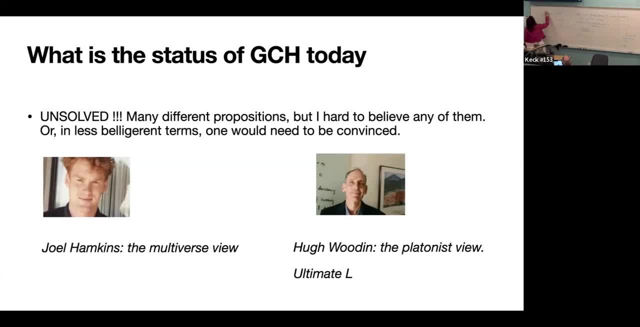 there used to be something called row bottom cardinal, Also defined, And row bottom cardinal doesn't exist. That's theorem of Kuhnen. So if the Kuhnen proved that actually you cannot play this game as far as you like, you can just keep putting stronger and stronger. 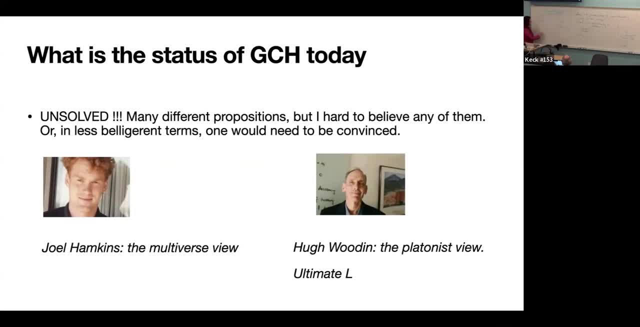 So Kuhnen proved that ZFC actually proves that there is no row bottom cardinal. But you see, the point is that we cannot prove the existence of these cardinals in ZFC, But for we know, some clever new Kuhnen could prove they don't exist. 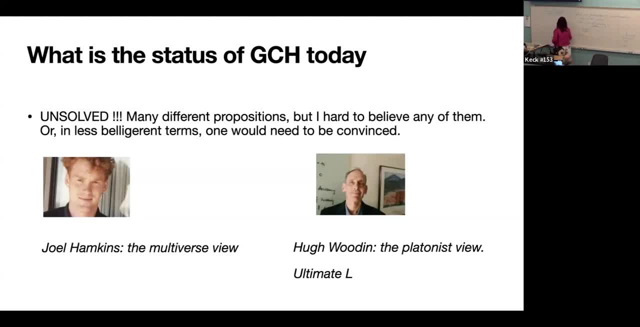 But the super compact. I think many people, including myself, would be very sad if we have such a proof. Most people believe that super compact cardinals are actually a natural concept. The existence should be happening And this ultimate L is basically like L of a super compact. 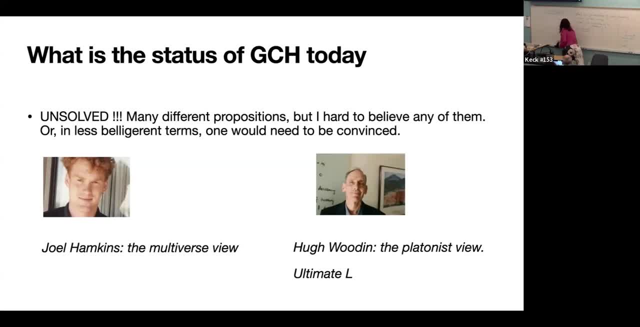 So L of lambda, that would be this idea of the ultimate L, But of course you cannot construct it in the way that Kuhnen constructed this model, because of the results of Steven James. So if such a thing existed, you would need to have a new way of building inner models. 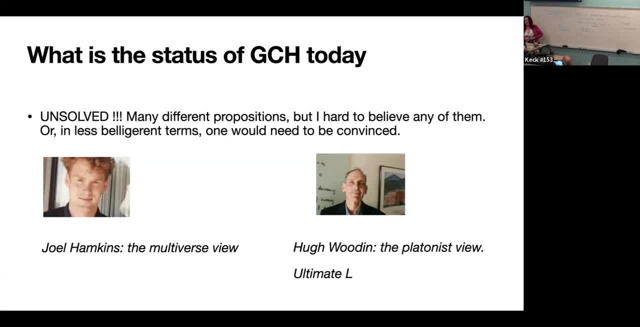 And that's why this conjecture cannot be formulated, because you don't know what this new way is. So is this an axiom? Not for the moment. Is this ever going to be an axiom? So the axiom would be: V is equal to L of this. 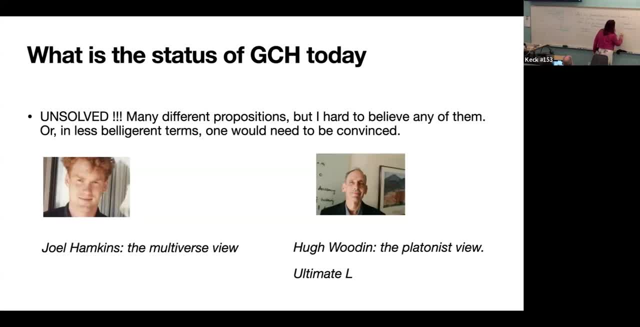 V is equal to L of this And this would be more annoying. Extenders lots of things to even say what this means. I don't know if this is an axiom. There are people also who think that forcing axioms would be axioms. 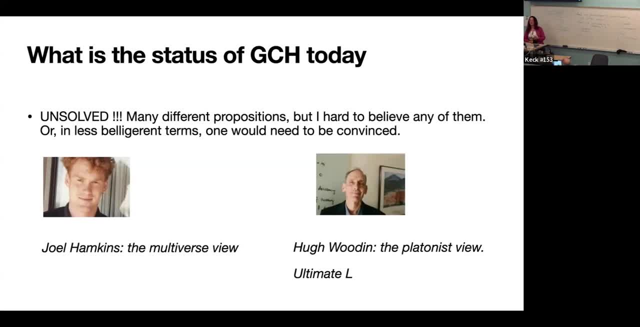 I won't bother you with forcing axioms, but there are forcing axioms which say that the universe is saturated by some forcing, And then some of these axioms decide that the value of the continuum to be L of 2. That's kind of nice. 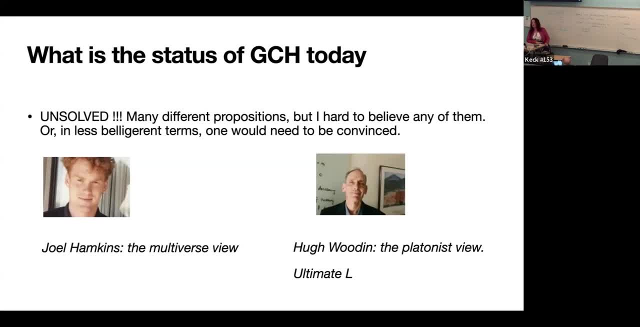 This is nice. But then okay, is it an axiom to say proper forcing axiom, I have a proper notion of forcing and I have L of 1, many bandsets. I can find the generic filter to intercept them. Do you think that is an axiom? 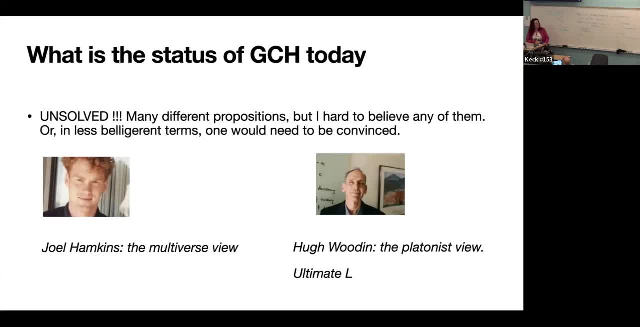 I'm out of taste, So I'm not really sure that this. well okay, this is not an approach that seems to me to lead to a completion of the universe. Is that because it doesn't sound natural? Yes, That's what you mean by an axiom. 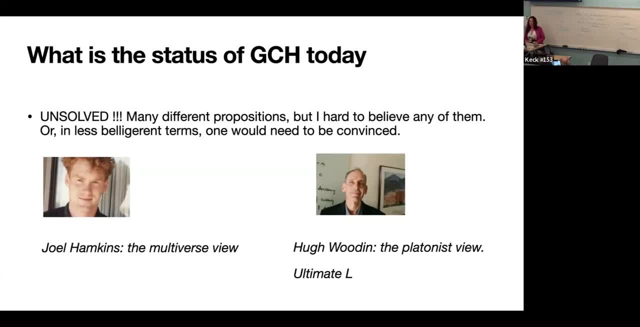 I think for me an axiom is something that sounds natural, something that people can actually outside of the field can understand. So the great cardinal axiom- not axioms will nobody outside the field can understand. I think this one, I think you put it. 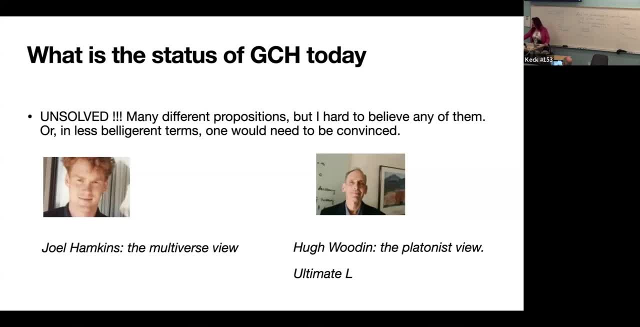 yeah, the measure is, you know, something quite natural. Now, some of them are, you know, perhaps not so natural, but many of them you can give as a combinatorial statement- I don't know- strongly compact means, if you take the logic. 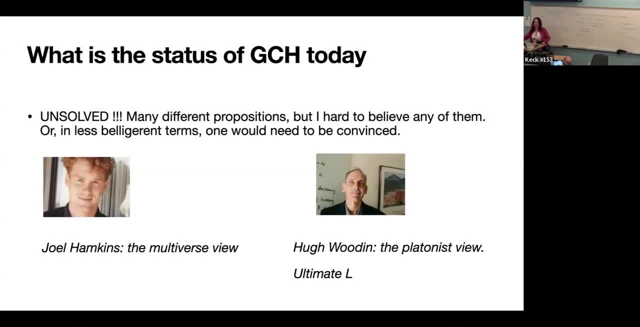 which is like first order logic, but you allow conjunctions and quantifiers of things of size less than kappa that is countable. then you obtain a logic which is kappa comma. I think this is a great definition You still can understand. 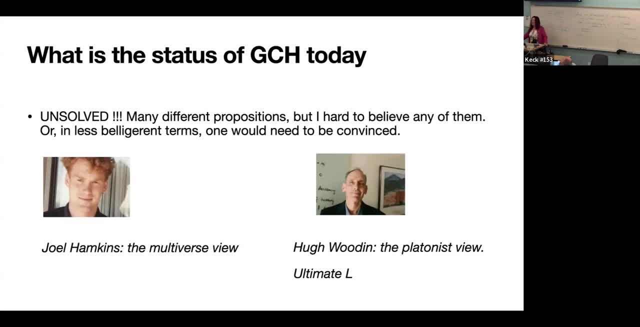 Everybody can understand. So this is, this is not. You seem to say that an axiom should be not ad hoc, Yes, And secondly, sufficiently general- Yes. That's what I feel. Now, of course, what Wooden has done. 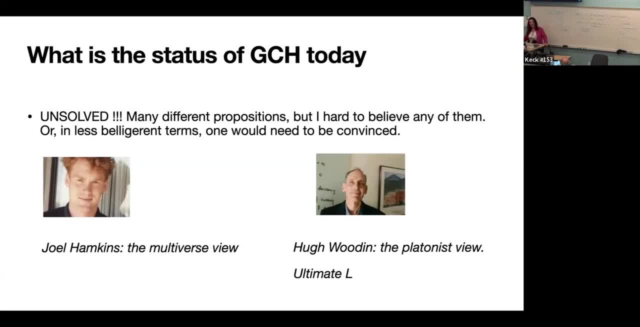 in developing this ultimate L. that L is not ad hoc. It's a result of many, many years of deep mathematical work, but it is not natural. Well, perhaps more work on it will give something that's natural. Can I just ask? 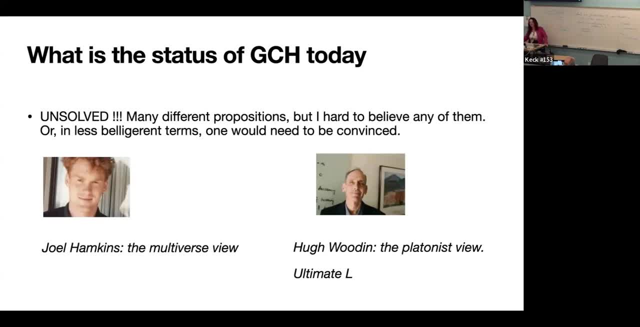 with the ad hoc requirement. does that rule out the continuum hypothesis as a axiom, Because that's understandable to people outside the field. That is the question. It doesn't rule. I think this is. this could be a good axiom, Only the reason for that one. 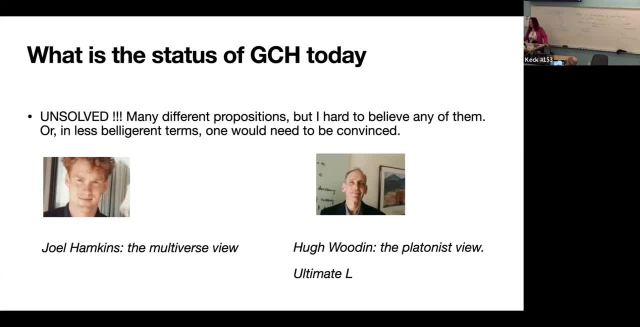 actually is. why would we accept- Sorry, Why would we accept such an axiom? Because that's another thing that we need for an axiom. You have the recommendation. It says that we should find new axioms which entail GHCH, for example. 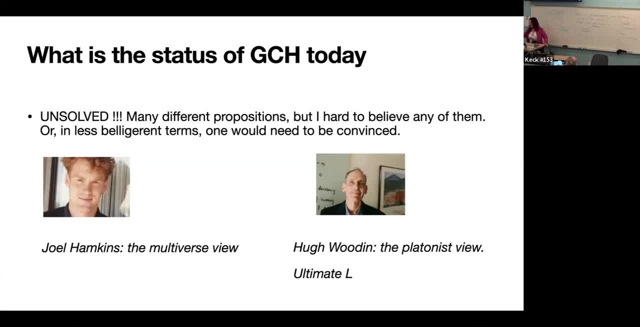 CH. Yes, this is what the whole California school, including Wooden, has tried to do. So this, this is the problem with CH. It's not that it's not natural, but that we don't see why We should choose it. 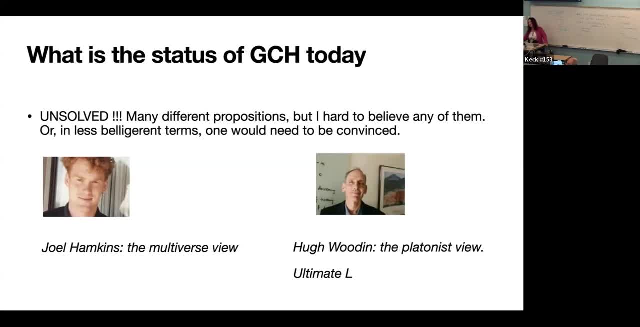 But then Wooden's program is that he's going to find something that we can see why That's right And this ultimate L conjecture implies CH. The proper forcing axiom implies the negation of CH. That is our problem, that both of them 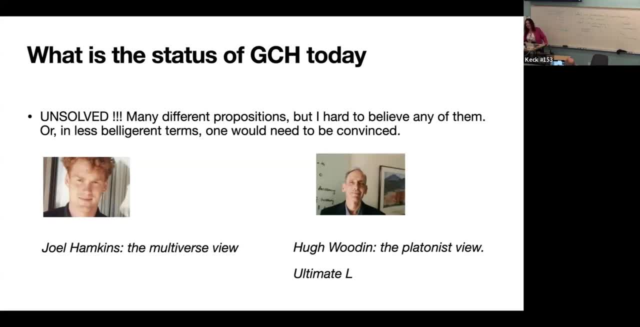 are interesting to saturate and they have contradictory. But then again I come back to the issue that Wooden. he says that you should find new principles, formulated by new axioms, which would clarify the notion of set, And this would entail decision of CH or of GCH. 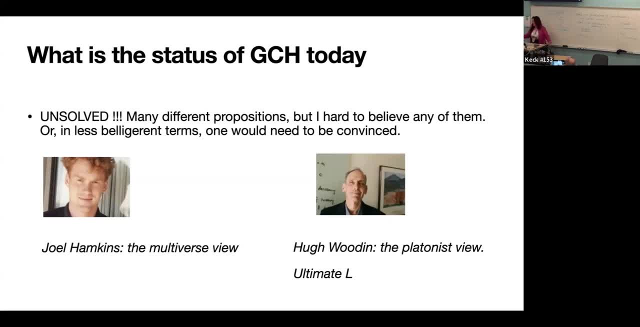 This is an excellent idea. I don't know that there is progress on that. Maybe people will categorize your DC sets, And I wanted to come back to your questions, because what is an axiom You are defining it? No, I'm just saying negative things. 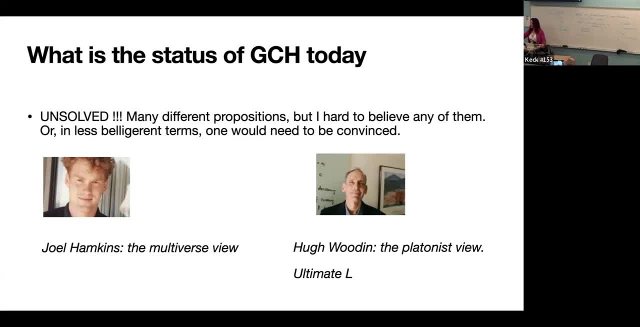 But still it shapes something, Because an axiom is something general, something which helps us understanding the structure. Yes, And what are foundations of mathematics, apparently, is to find a set of good axioms, in the sense we just said, which ground everything. 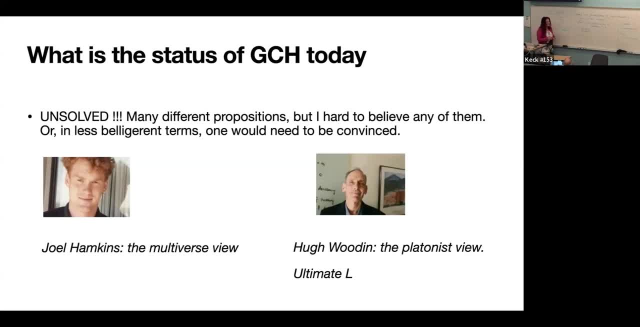 Well, yes, So this is another question. Actually, I do not believe in this, I don't believe that there is such a thing. No, No, That's what I just want to be. I was trying to clarify you, No. 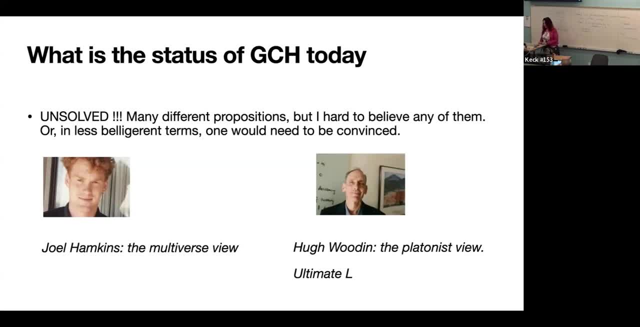 Yes, So, Michelle, I think that we will come later in the discussion on that, But if this were the condition, so the point would be why we need an axiom to solve the continuum hypothesis, Because apparently set theory does its work very good. 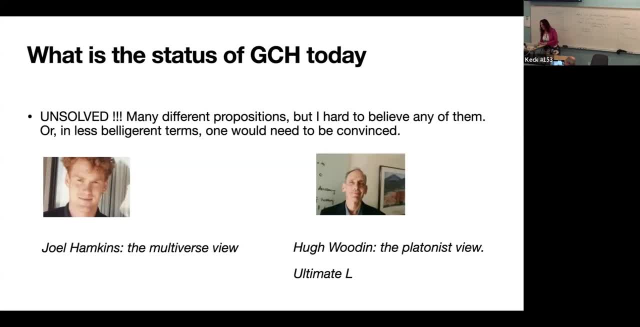 very well to learn mathematics even without knowing the solution. Yeah, So we don't need any axiom to solve the continuum hypothesis in order to find mathematics. Yes, It's good, So clearly we have. we need something else. Finally, 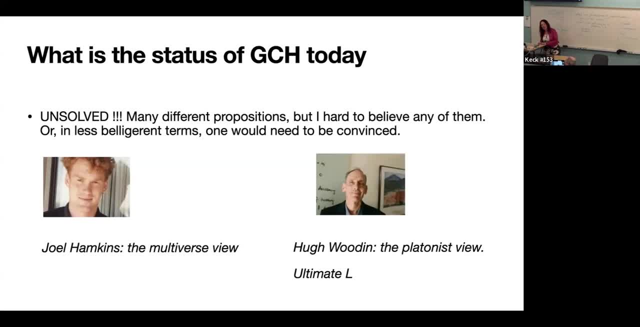 there is, set theory is also mathematics. So what I think is that modern mathematics is not really set theory does not give foundations for all of modern mathematics, And I'm very convinced it is. I'm one of the rare set theorists who feels this way. 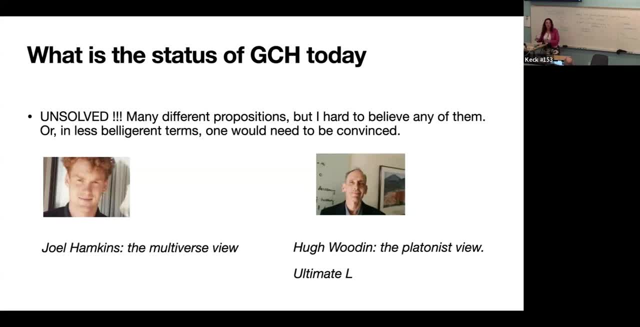 but I don't feel that way. I feel that there are okay. first of all, we know about category theory for a long time, But there is the work of Fefferman and others in the 60s and 70s that show that. 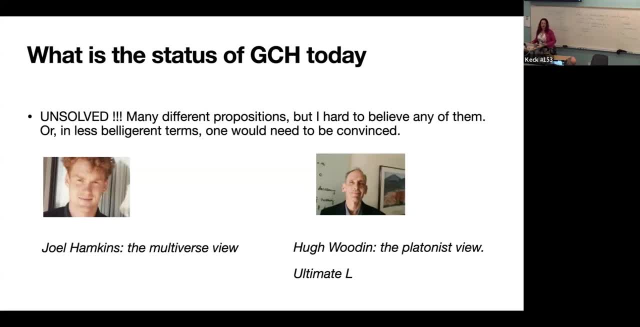 even though in some contexts it's more natural to use category theory. if you accept set theory with a couple of large axioms, cardinal axioms, then we get categories. So this is kind of bi-translating. So I think that this is very comforting. 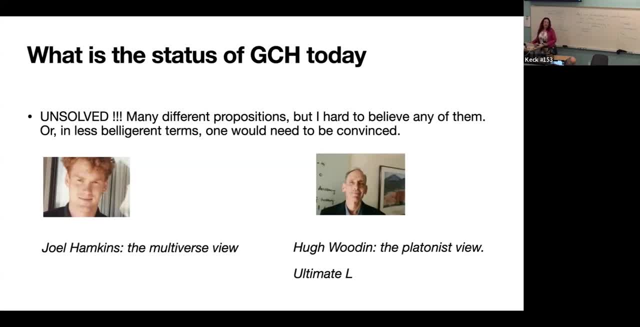 And I do still think that it is much better to work in mathematics with a language that actually helps that part of mathematics grow. So I don't think that algebraic geometry should translate their arguments into set theory just to please us who know candidate sets. 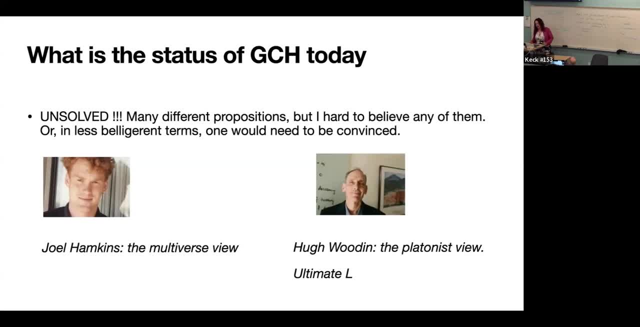 Whatever people should be using foundations that fit them. But there are other things. There is, for example, this homotopy type theory. It is somewhat different Then set theory. it has a different notion of a basic object. It creates types. 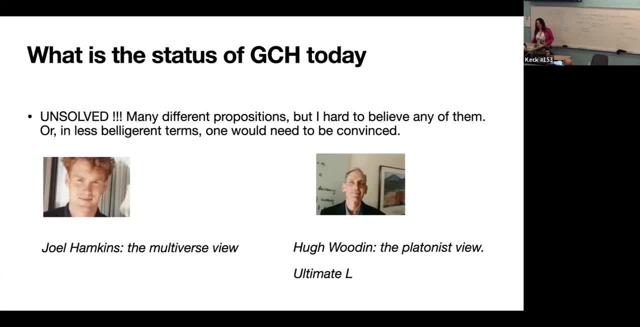 It doesn't have. it's much more syntactic than semantic And it is a base of the notion of types, particular types, And I think it produces very interesting mathematics. It collaborates very well with theorem verifiers, especially with many languages. 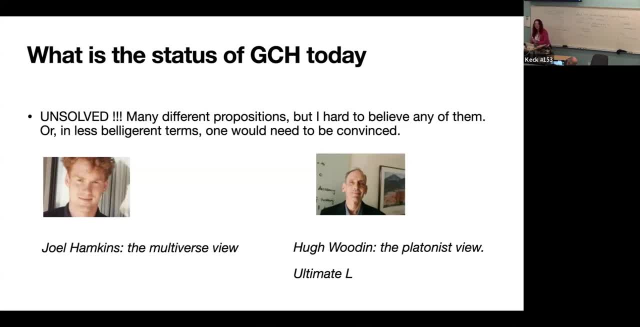 that are developed for the facturals now for subtextuals et cetera. Should we just reject this? It doesn't fit the mathematics we do. I think this, I think this would be stupid, But I also feel. 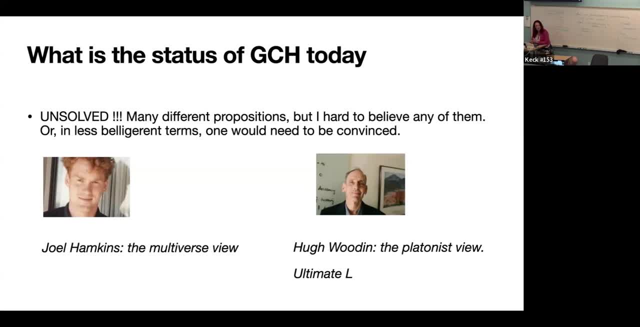 that it would be stupid. the other way around That, because there is some theory that says that it is good for theorem verifiers and then then we should reject the set theory Absolutely. I couldn't agree more. I think we can do mathematics. 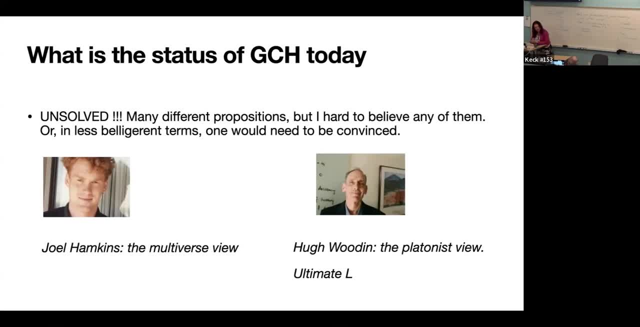 We haven't seen any contradiction yet. It doesn't seem likely that we're going to find anything soon. Yes, Why shouldn't? why shouldn't we use set theory to do mathematics? It's true, Exactly. I agree totally with you. 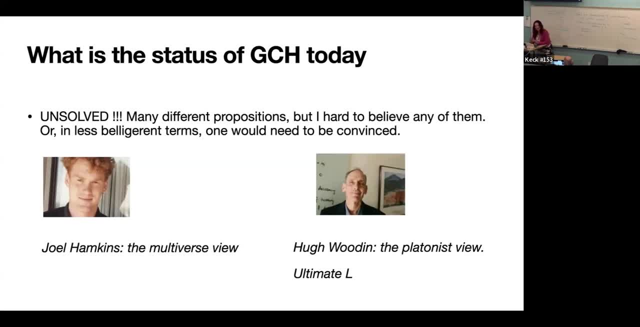 We should use set theory to do the part of mathematics that set theory can formalize. But we shouldn't take it as the world's greatest tragedy to know that it doesn't form everything. It's just perhaps what we should do to find that, to explain it. 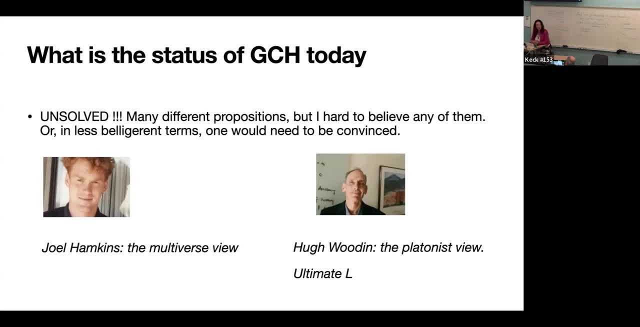 Maybe we managed to find big foundations for 19th century mathematics already. That is not that, But the the most clear argument in favor of the fact that there is mathematics that sounds set theory is. there is a discussion about the hypothesis that this discussion 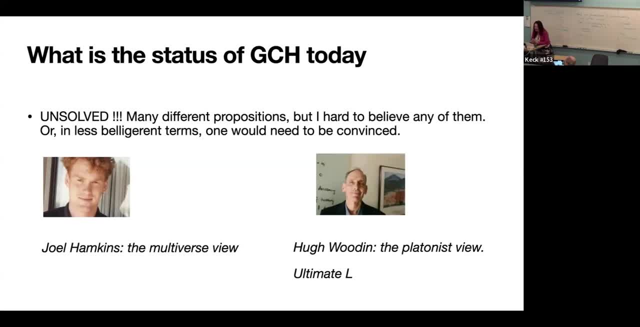 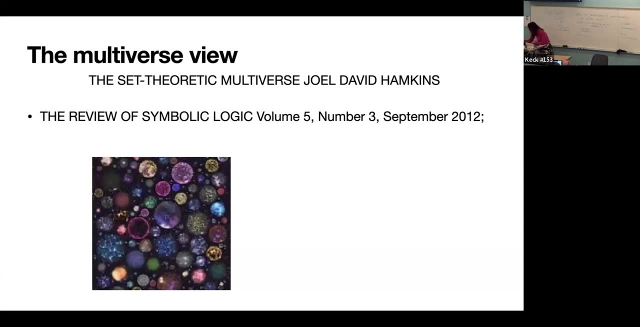 is not mathematics or it is a set theory. So maybe let me tell you some other things, because you're talking, you have other things to show us. This isn't a discussion. part of it: Yes, this is, this is so. this is the multiverse view. 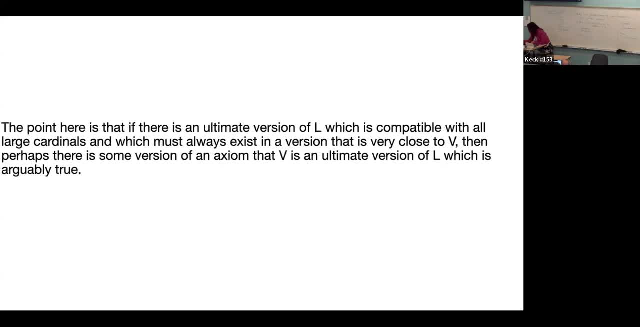 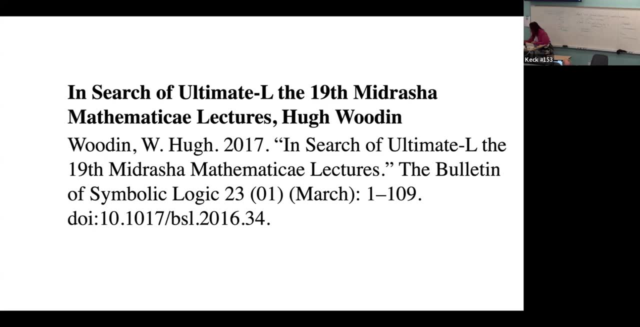 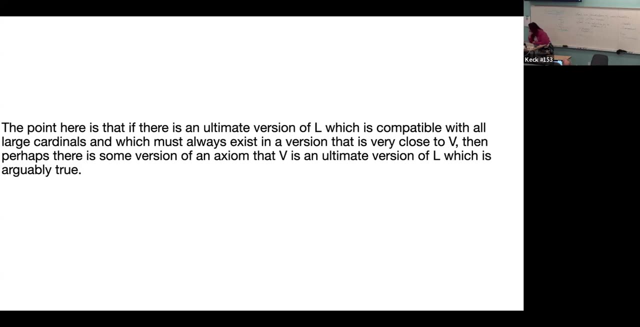 I wanted to talk. this is about this reference to a newspaper. Can you give me the? can you go back to the reference? Okay, Thank you. Yes, Then this is what he says. Let me read it. Maybe there is a which which. 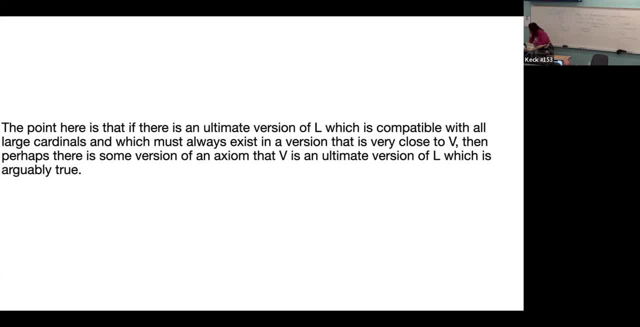 which must exist. There is some selection that we need. So here I have a question, because we heard in very recently in the conference organized by the MPP program And he seemed is going to give an answer to ch and gch, but he seems to think that ultimate l is going. 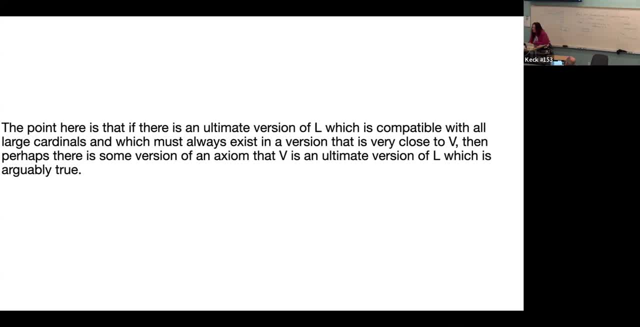 to decide everything in set theory and it's going to deliver the whole and complete truth about sets even more impressive. but you cannot ever this would make, uh, that fc decidable. that it cannot be, because i'm going to hear it- he doesn't go that far, but, yes, this is. 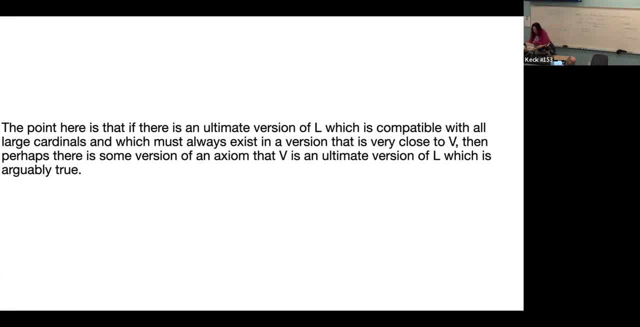 strictly what he believes. as i say, he, that is what. that is the search for these ultimate axioms for mathematics that motivates him. so, uh, in this conference in barcelona that i mentioned before, in which there was a discussion of what philosophy can do, set theory. well, i much of the view that uh. 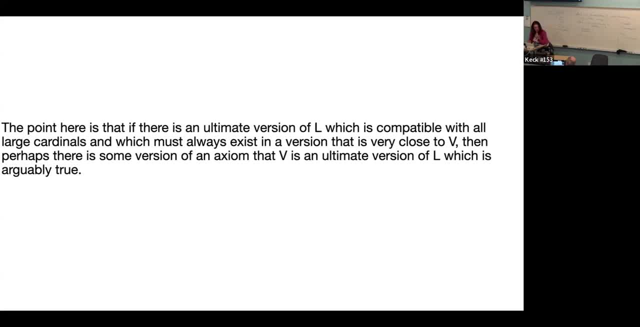 some of greatest mathematics was done by some, uh, political motivations, even though that person perhaps in that question did not formulate this philosophical motivation in public, but had the philosophical motivation and since he was there he discussed this. uh, there was a discussion section that i asked him this question he very much confirmed. 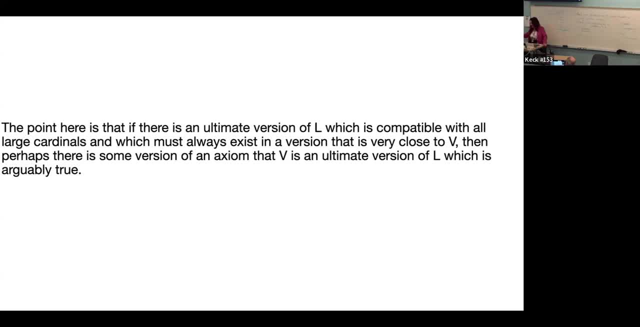 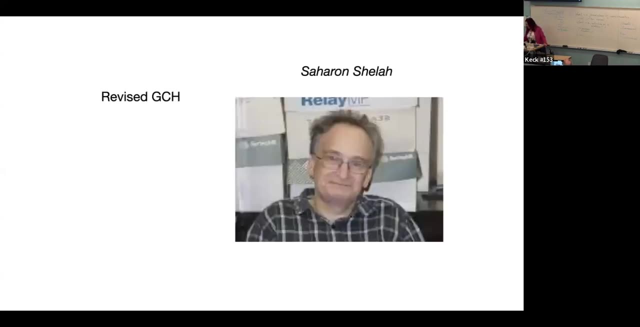 this so few- has a philosophy that leads to have this opinion and, uh, he's arguing for his philosophical view, and i think this is a fantastic cue, etc. i don't happen to hold it 100, but that's. that's what philosophy is all about. so let's go back to mathematics. 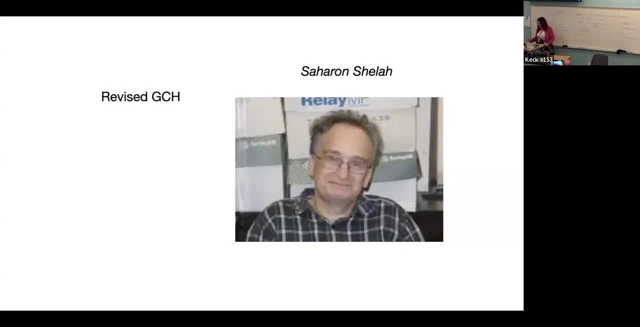 so revised this age. so what does he think? see, he also does uh have philosophical views, of course, but uh not. he doesn't consider this as a uh part of mathematics. so his view of mathematics is very mathematical. we do mathematics uh to uh to solve mathematical problems. so what is the real problem? 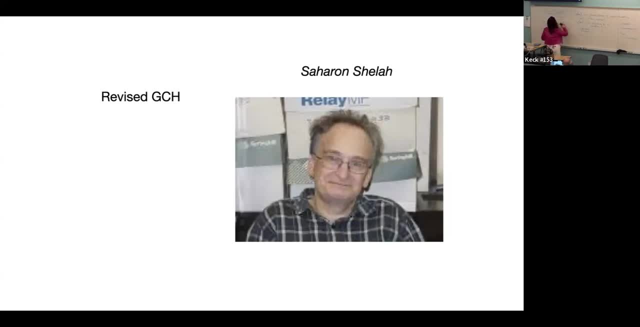 about gch in the opinion of you also. someone is that uh canton found these two operations on the cardinal, then couldn't find any other ones, and he formulated this hypothesis, which makes sense if you think that there are only two operations, but if you find some other non-trivial operations on cardinals. 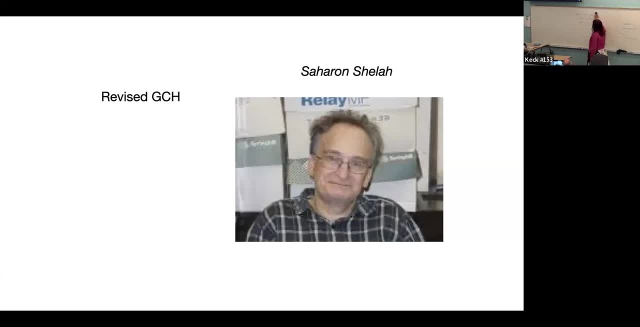 then you're going to realize that maybe it is not at all reasonable that you should think that they should coincide. so let's go and look for some revised version of this each, which would be: you find some non-trivial operational cardinals and you prove that these calculations of the 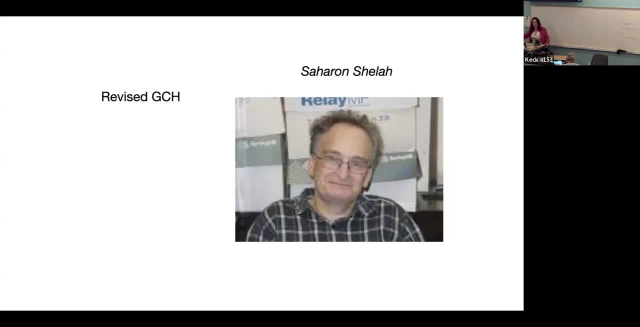 value of this operation are independent of force, that you cannot destroy the value by forcing. so here is the operation that has some background. uh, the operation is like this: you have two cardinals, one by kappa, and now what you are into is the dot in is not just subsets of lambda, the whole cardinals subsets of lambda, but you are 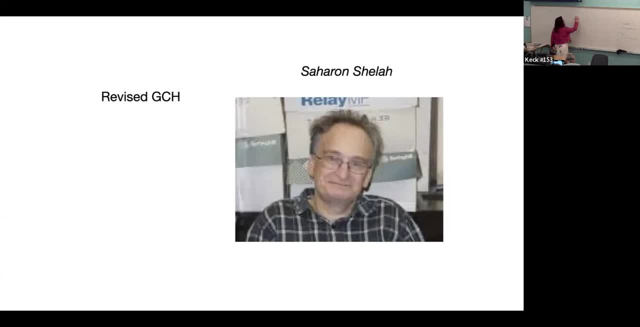 interested in subsets of lambda that have cardinality cup, so kappa is smaller and you want to say something like that. so, uh, some people denote this way, some people do not this way. that's like this notation. so what can you say about this thing? so you can count them, but that counts. 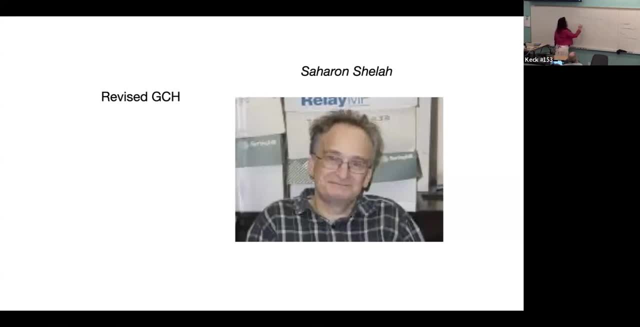 this is something that also depends on the continuum considerations. let's think of them this way, but you might do something different. you may say: well, these sets maybe have some, maybe they are not just disorganized sets that we want to count, but maybe there is some relation. 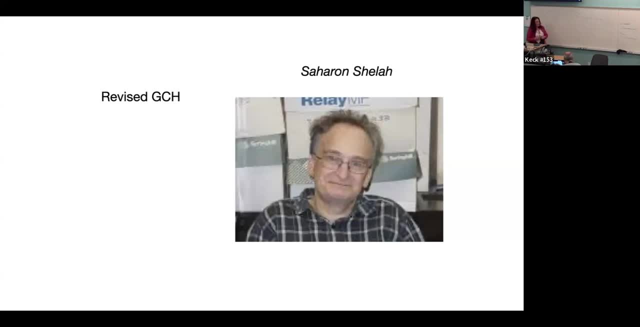 between them. so, for example, you may say, like in mathematics you sometimes look at partially ordered families, so this is a partially ordered family by a subset relation. this one should go to the garbage. i don't know that garbage is there- partially ordered by the subset relation. so this gives you now, rather than just a pure set, you have some structure. 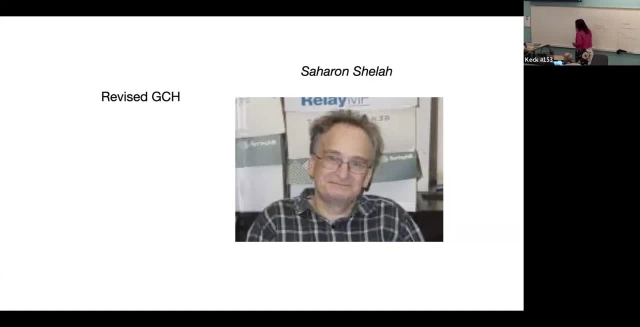 ordered structure and then you could maybe gain some knowledge about these cardinals by looking at some order structured properties of order, material order, properties of this. so one thing that people like to look at material order is to look at kind of dominating families. so what, what would be a? 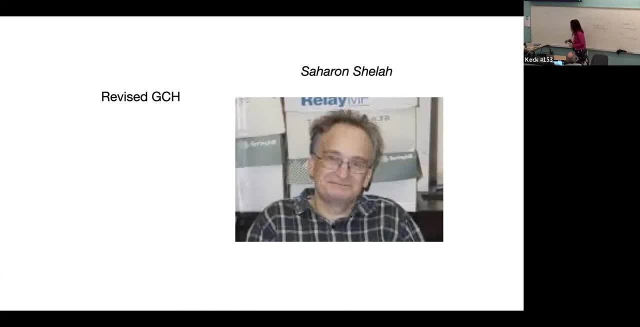 dominating family. you would like to isolate a family, a small family, inside of this set. save his pipe so that whatever element you take, it's below one of those, or maybe it's a below of a join of of a small number of these. so those working in boolean algebras will recognize this concept. 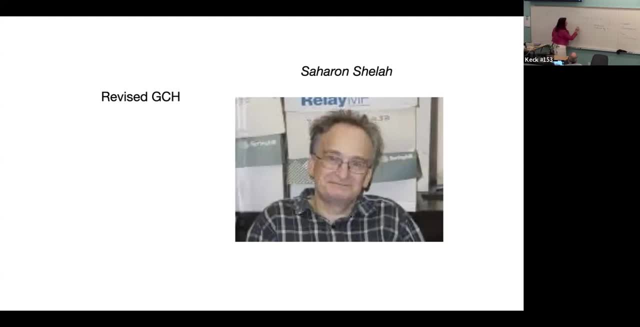 very much so told you horn to look at. is there some family like that, such that whatever subset i take it's, It's contained in the union of less than kappa, many of those special sets. That's the definition of this operation. So this is the minimal size of a family event of P. P is contained in this lambda. 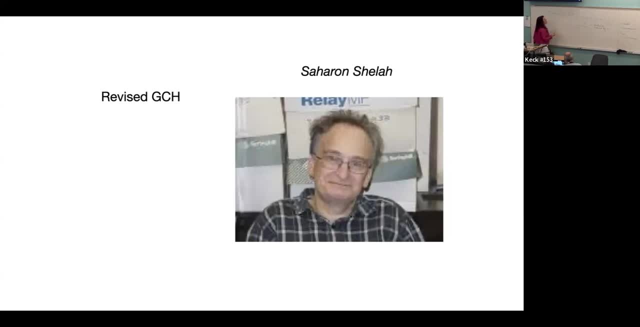 I like this and it's dominating the sense that for every element in lambda kappa P is contained, as a union of less than kappa, many elements of this P. So this has many motivations to consider. It's a nice definition. You could ask: okay, great. 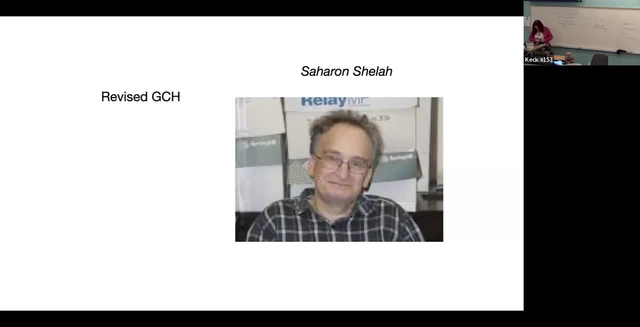 So now, why would this be interesting? Well, because what he proved is basically so. his revised continuum hypothesis, GCH, would be: let us look at this cartel and say: for I don't know seven, Here's lambda kappa. whatever, most would be. 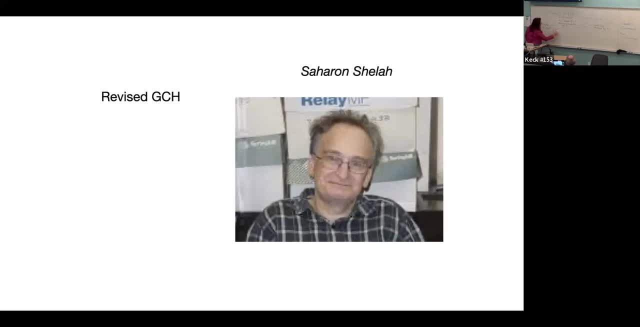 This is just equal to lambda. Is this set? Let us think of this state. So you see, the biggest value that this can take is the number of all subsets, the two to the lambda. The smallest value that it can take is lambda, because obviously it cannot be. 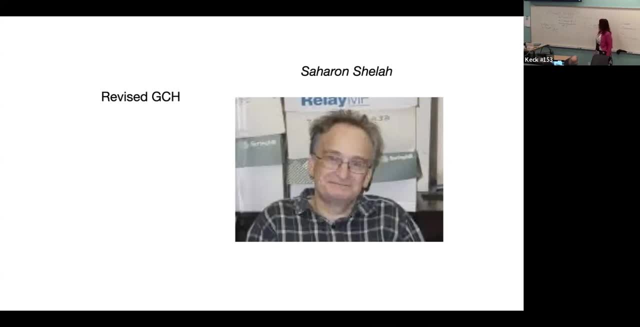 So this is said, this is as small as possible, as often as possible, Okay, And he actually gave a wonderful truth. That's really. this is something that happens often, So let me show you this theorem. Just call the device. 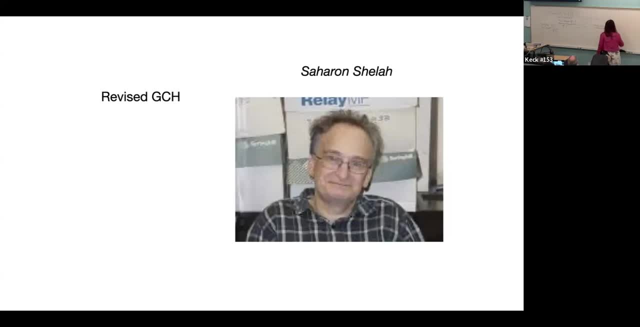 This is theorem. It says the following: Let us take two cardinals. What we will be looking for is the situation where kappa and lambda are kind of separated by some nice cardinal. So let us take the following: I take two to the other zero. 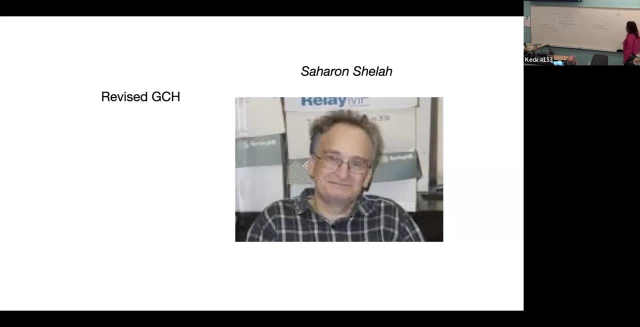 Then I take two to the other zero. I do this operation And I take the limit. The limit of this is called beton Here. so let me consider this cardinal beton, which I obtained this way. And now what I have proved is that if I take a cardinal lambda, 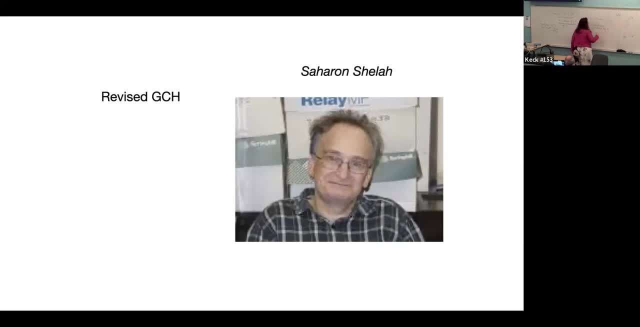 which is strictly above this beton omega. and now I want to calculate this with the kappa which are below. So kappa and lambda are separated by this beton omega, And this is only interesting when kappa is regular. So let us think of kappa regular. 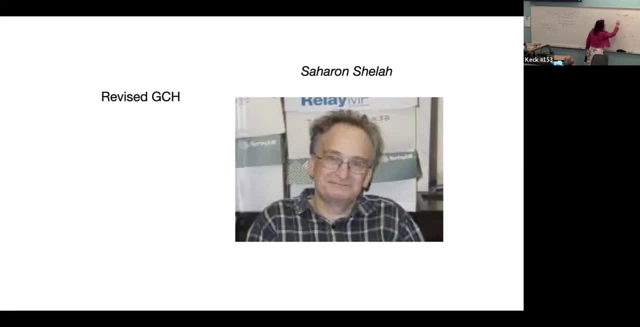 And here is this beautiful theorem. It says that there exists some for whatever lambda you take. for every such lambda, as above, above beton, omega, there exists some cardinal which are called kappa zero of lambda. So I said: for whatever. 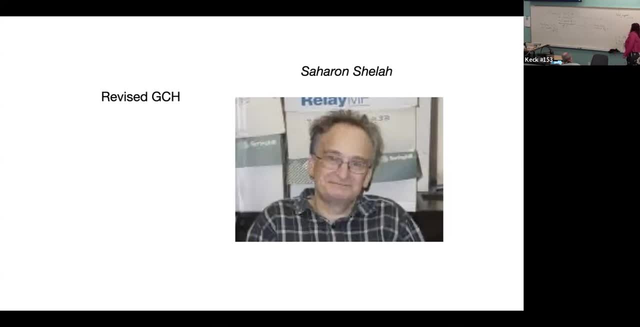 kappa. you take above this kappa zero, but still less than beton, omega and regular. you get a fixed value of lambda kappa equal to ice. I hope that some people can see it here: Lambda to kappa is actually equal to lambda. So this revised JCH is actually true. 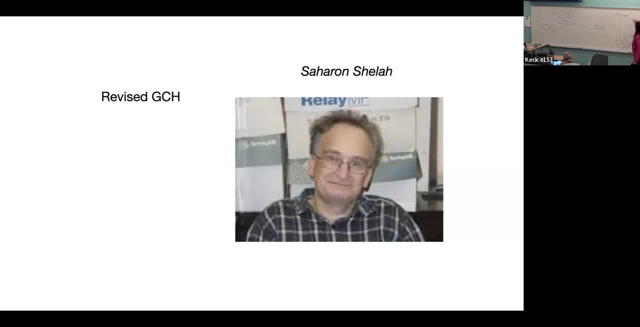 So let me say it again, I take the cardinal lambda which is above beton omega. Then I can find some kappa zero, such that for every regular kappa I take between kappa zero and beton omega, the value of the revised power set lambda to kappa is equal to lambda. 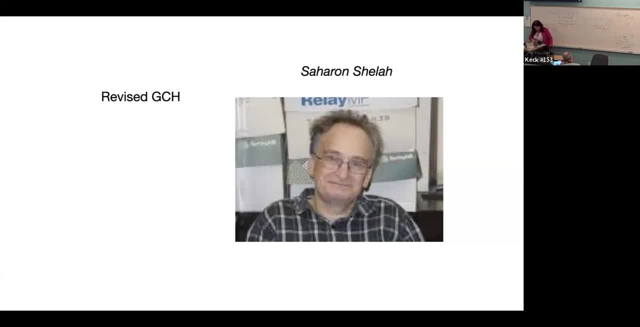 So I think this is quite an amazing theorem. There are many proofs of this theorem that are given in the literature. Key and his original paper gives three different proofs. And there is a recent paper just appeared by Todd Iceford which gives a three basis proof of this theorem. 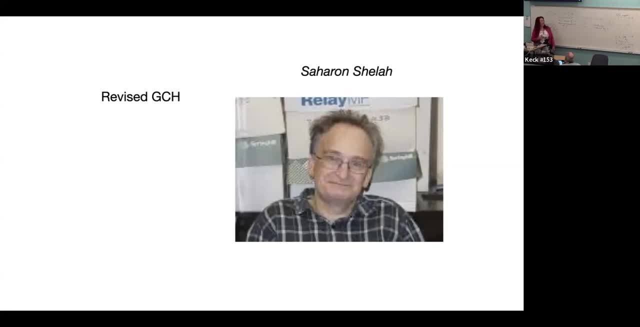 It's very nice, elementary almost, And so I just would like to recommend reading this paper, Perhaps looking at this part of mathematics, because for me, what's, What does this do? for somebody like me, It says: okay, philosophy is very difficult. 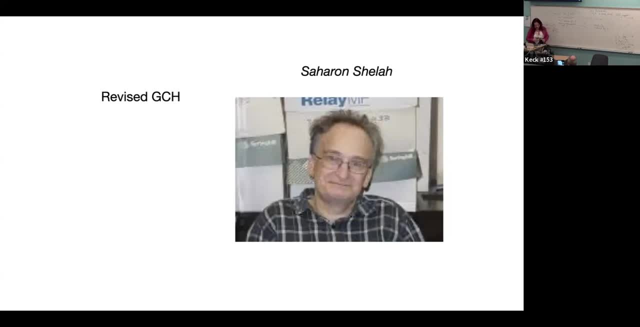 and we can think of it and we can discuss it, But this shouldn't stop us from doing mathematics. It should not stop us from doing mathematics. Yes, So in other words, we can still do something with the methods that we have In set theory. this is quite a beautiful combinatorial method. It tells us something about the structure of the universe of set theory, without any additional axioms. And well, I think this is something to know. I'm missing here this: what would be the new operation that you're mentioning? 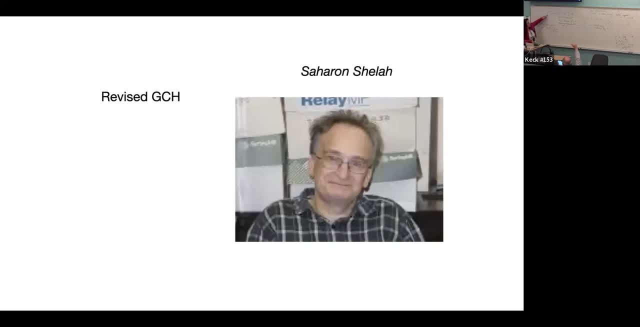 Is that the lambda to the Kappa is the minimal size- Yes, of the family of subsets of lambda, each one of which has size kappa: Yes, Such that for every set is a subset of lambda of size kappa: Yes, It's contained in the union of less than kappa. 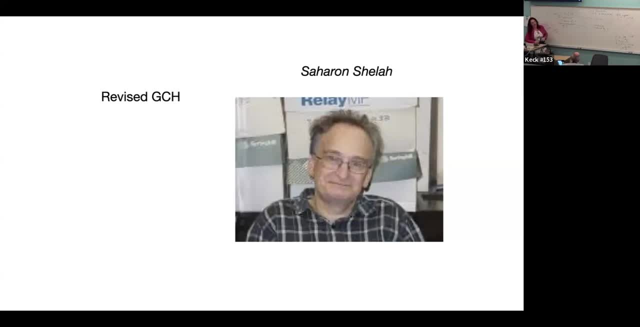 many elements of this special family. Yes, So the other two operations that we considered before, which is the powers- Yes, power set, and the next, cardinal- Yes. Does it always give us some cardinal that is larger? Not always, because this could. 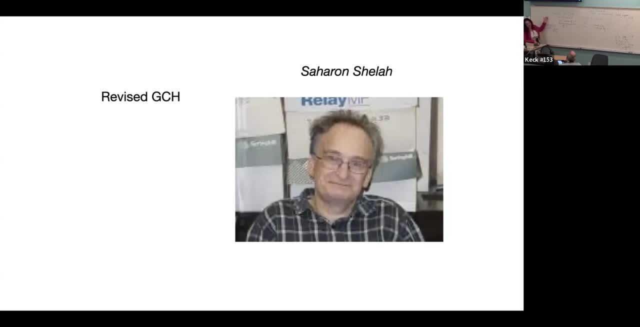 in some circumstances, this is even closer to the lambda. Yes, This is my question. So how is the existence of this operation telling us something about the other two operations? It isn't. It is not. So the idea is to move from those two other operations. 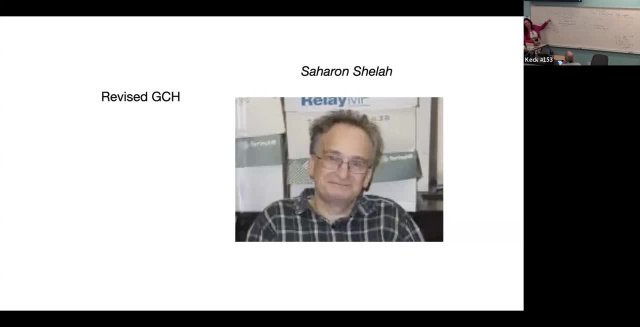 because we can change the value. So this is telling us something about lambda plus or kappa plus, Yes, But about two to the lambda. Two to the lambda is just very sensitive to the universe, so we can change things And this is not. 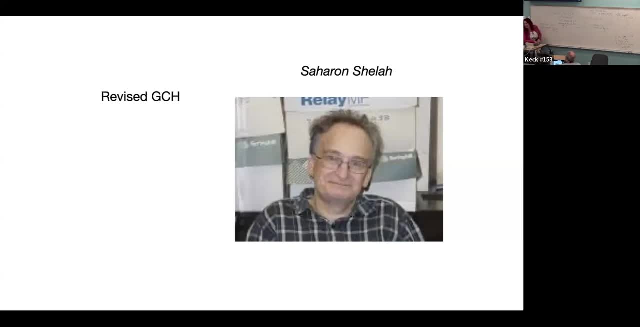 So kind of this is something that is more. Thank you very much. Thank you Great. So this is the idea to perhaps look at things that we can say something about, which I think is so much of the Yes. This was also the idea that Mark and I expressed. 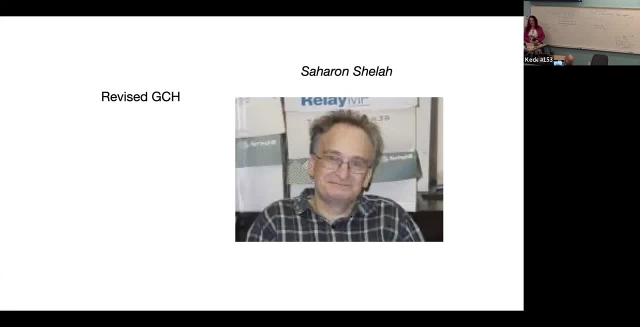 in our joint paper, which was called Asymptotic Thought in the Universe, or something like this, in which we argued that well, even though the universe of Sathya seems to be very vile, if you look somehow to some asymptotic behavior, 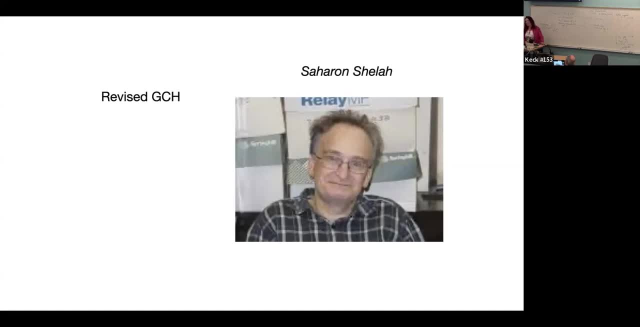 which we defined there. then you can actually say more things. We were concerned about singular kindness, not behavior. But the most fundamental point of this paper, according to me, was that this drawing of V is not a good one. We suggested a new way to draw V. 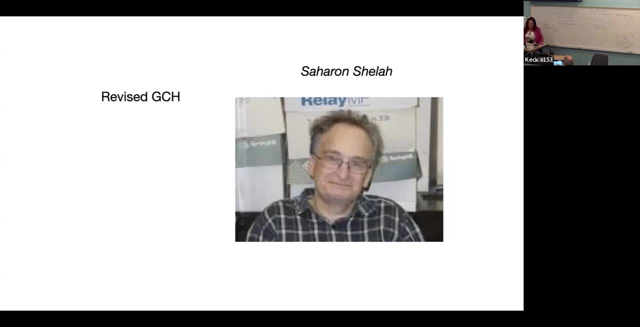 Yes, This was a new way to draw V and we still haven't done it. I'm very proud of this. We should really work harder on this propaganda for our education. But you tell me your question. It's time, Sorry. 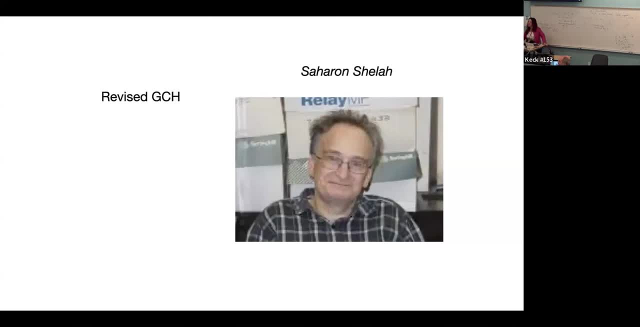 Is it a question, With this kind of work, you turn your back on not doing work. You don't turn your back on that. You just don't need that for this particular? It's the idea that we have some job to do without this kind of work. 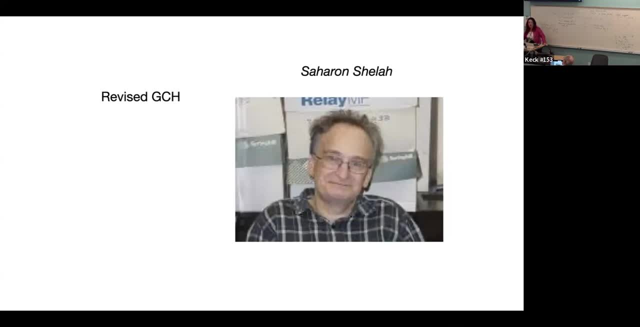 Even without them? yes, There is combinatorics there, So I think Antor could have understood it to answer this question. But isn't it something that, if we have, the inspiration of the large cardinal hypothesis is that we are going to settle the pilot by 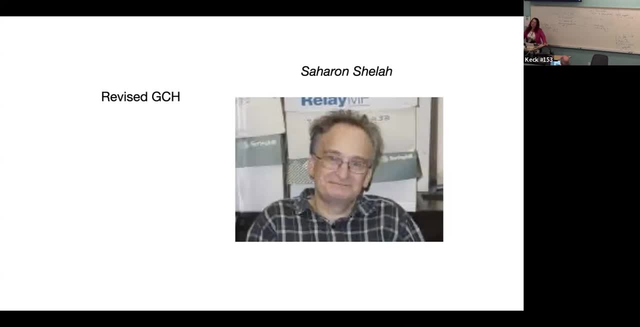 jumping into a very large infinity. Yes Well, large cardinals were defined before this action. They were defined actually, the motivation was by Lebesgue. So Lebesgue constructed the measure which he thought would measure all substance of the reals. 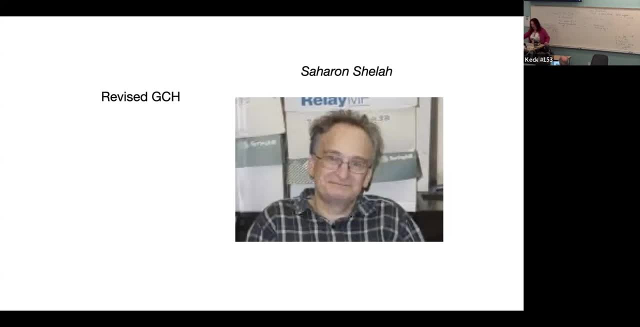 And Vitaly showed that by the axiom of choice this doesn't happen, And the two of them had very different opinions on the bridge of this, So Lebesgue just thought this means this obviously proves that the axiom of choice is wrong. 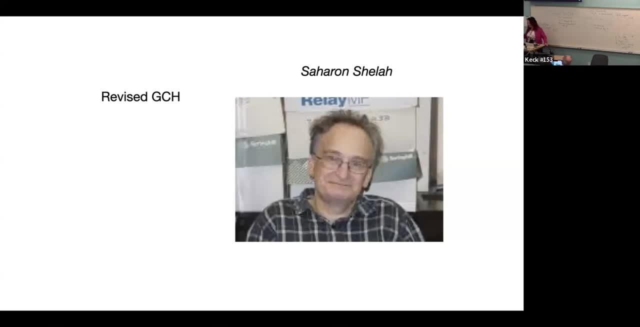 It doesn't seem to have been a very modest thing, Lebesgue, from what I read. And anyway, some other people said: okay, but could we have something like this? We have some different numbers in which we have a measure. a measure, that's all substance. 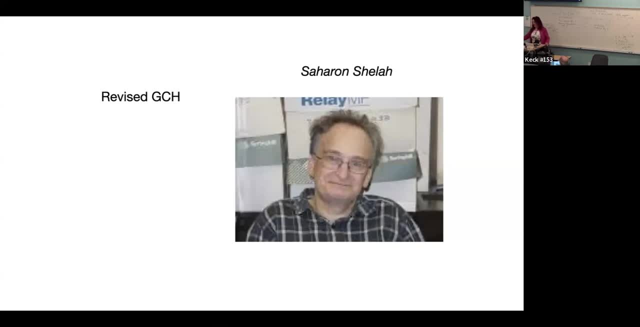 of it And this became this question of measuring the sum of stations. that is, how the large cardinal. Yeah, any questions? Yes, Is the good order, or you want another order? Okay, Let me start with a very naive question. So in the second round I try something more involved. 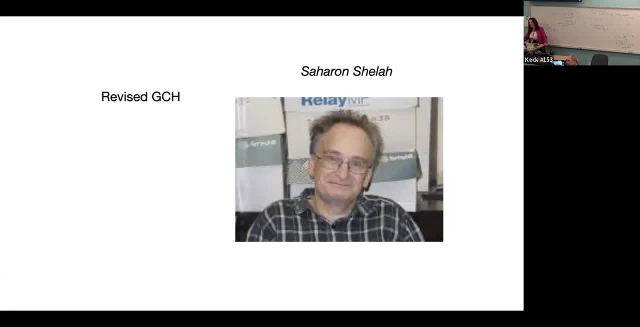 In the 19th century there were big discoveries: first of all, that the trisection of the angle cannot be done with this triangle, And the second one, which makes a very vague mess, the Frobenius theorem on real ardebras. 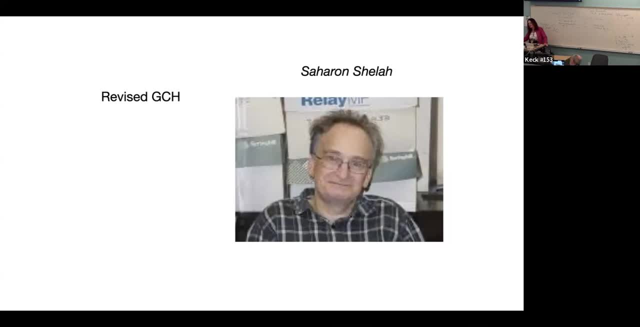 when you've got Cartesian products of reals. Frobenius showed that we can introduce the structural field only real numbers, complex numbers and Hamiltonians and no other, no other, And it was a shock for the mathematicians of the time. 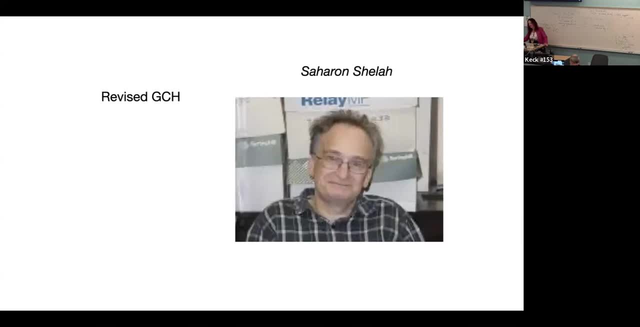 I wonder: what's the difference between these results, 19th century results, and the Cohen result? There is a Chtonian. Yeah, algebraic, Yeah, algebraic, Yeah. There are ardebras. There's one more. 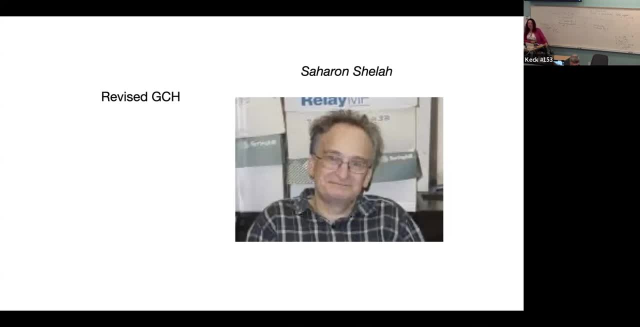 Ardebras, not field. There's one more, It's not a structure: More ardebras. What's the difference? What's the difference? But I think these results are positive effects. You know, they say this result of Frobenius is positive because it's classified exactly. 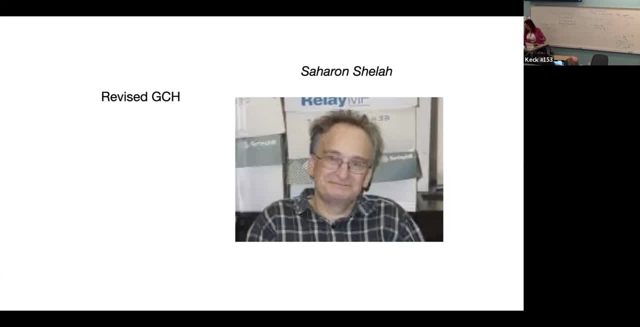 these objects that have certain coefficients and no others can have. I think this is a You can do it in a negative way. Yes, you can do it, But usually we like So, for example, the fact that the coefficient is negative. 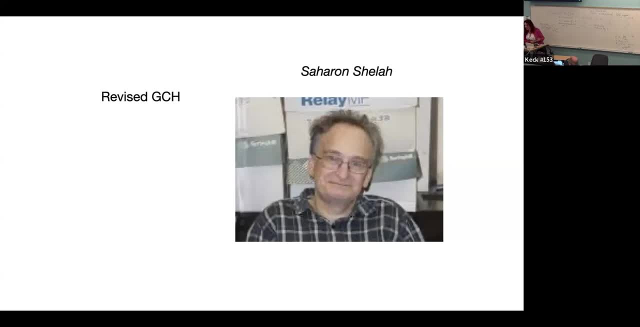 The fact that the complex numbers are complete for solutions of algebraic equations. This is a great propaganda for complex numbers. So the other ones, you mentioned that we cannot do a dissection of a triangle, So they kind of go down to showing the piece transcendental. 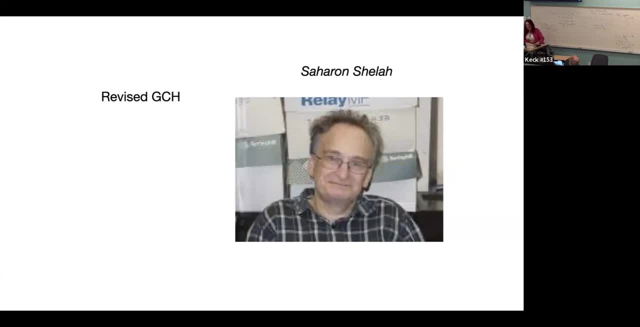 Well, obviously these are great results and I think perhaps they are in some sense like So. in that sense, maybe the discovery of Poisson could be seen that way. Yes, It's not close, because you've got the techniques, the contradiction of techniques. 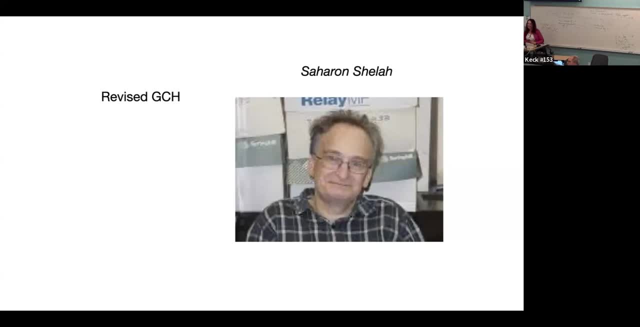 Frobenius, you were going to just do what you want and you cannot introduce it. Yes, Okay, Prima, Thank you very much. Thank you very much. Thank you, Maybe just a curiosity, I don't know, But it's a question I wanted to ask before. but then, 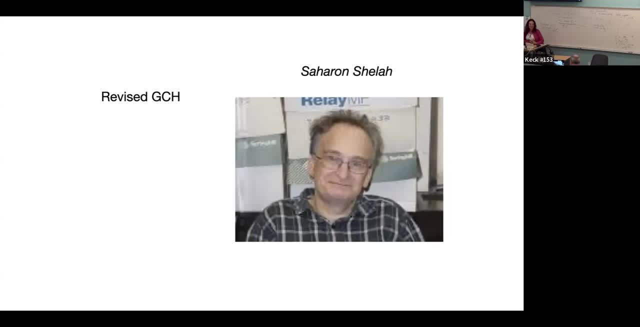 In the multiverse version, the argument that you need an external universe V, is that universe actually requiring all the axioms of ZFC, or can it be done with less? I'm thinking of replacement. I think that's the question, Uh-huh. 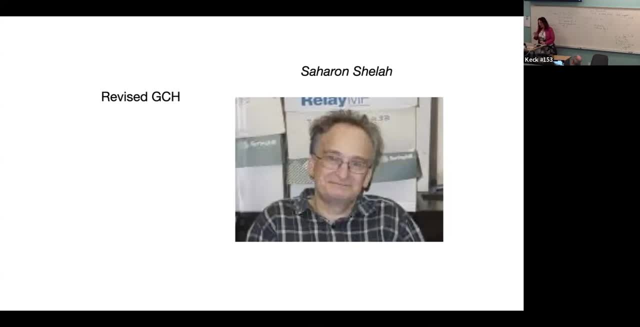 So you need replacement for forcing? Uh-huh? Well, this is something that on the top of my head, I would say no, but here what he looks at: all possible forcing accesses that can exist. Ah, So perhaps in that context you probably 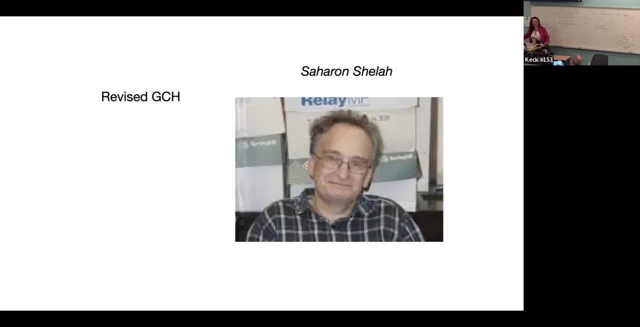 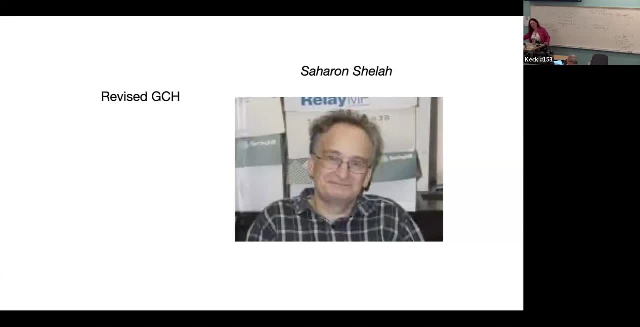 Yes, Yes, Yes, Yes, No, Let's continue. We'll come back to you now. Okay, I have a question. This is really a topic with the reps, so I always said I never understood why people do not accept V equal L as a good explanation of what the set theory is, and so in this, 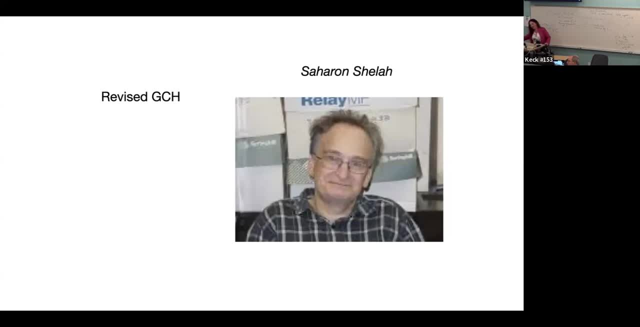 particular case. also, I did not understand why you wish a measurable Cardinal to exist. Well, the answer to both is… Why can't we give up? just say they don't exist? Why not, We can. So you know, we can do. 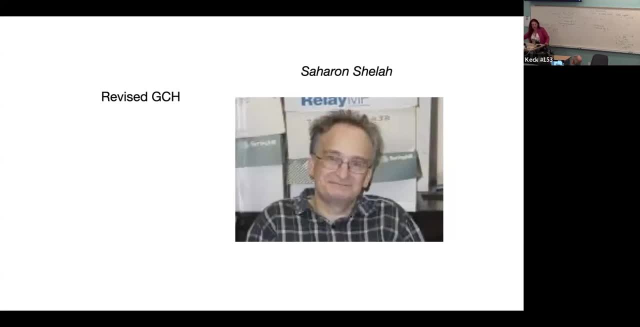 finite mathematics like there is not this. no, it's much bigger than mathematics, of course, but it is depends on your personal interest in mathematics. discover the questions that you're interested to resolve or not. some people's questions can be resolved in finite mathematics, but what are the questions relevant? 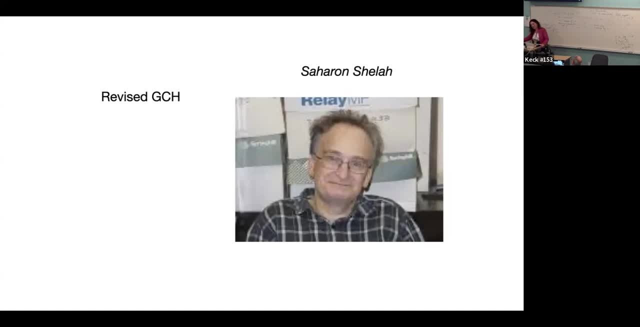 for applications, for instance, that you cannot do under the assumption v equal. well, so this again. so why would we only consider applications? and what do we mean by application? a few years ago, you know? okay, well, I will say something about application. I think that the applied mathematics of today 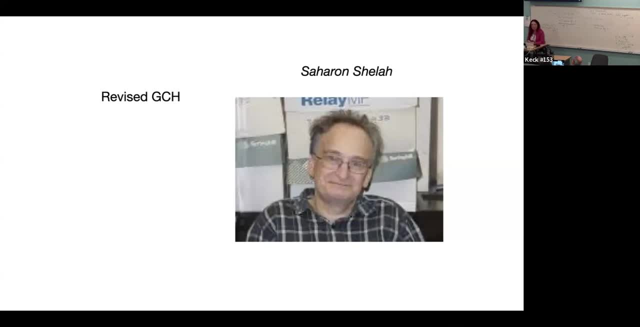 is not happening with mechanics and subjects that I think are applied and ready and so forth. I think the applied mathematics of today is happening with logic and theoretical computer sciences. so you know the artificial intelligence that everybody's talking about, that people neural metrics. now it has neural, not logical metrics. 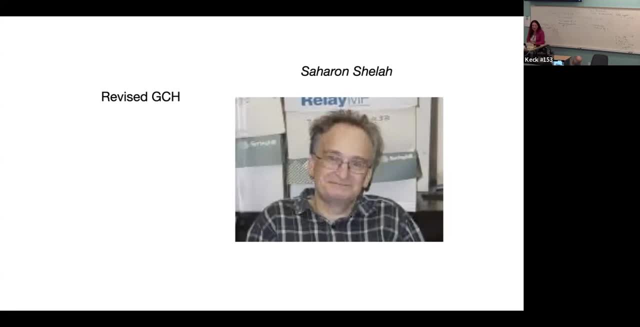 there is a paper called alpha geometry that came up a few days ago- perhaps you've seen this very recently in Geneva, yes- which is talking about how which has trained the model of artificial intelligence to solve olympiad level models at problems in geometry- very difficult problems and most human people. 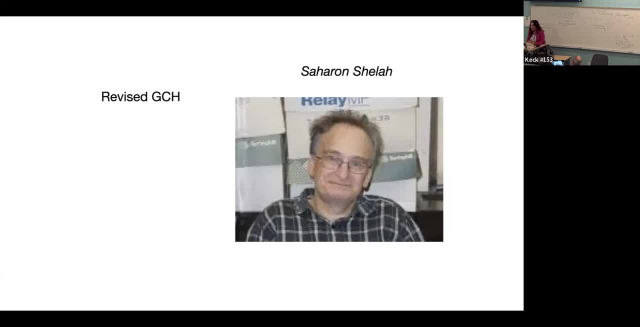 beings, including mathematicians, cannot solve. there's quite a skill to go to the laboratory. this problem is: these are patients. what logical? okay, not really. I think that the answer to your question, I know equally, is to see no, just applications of logic. that's what you define. a lot of points. 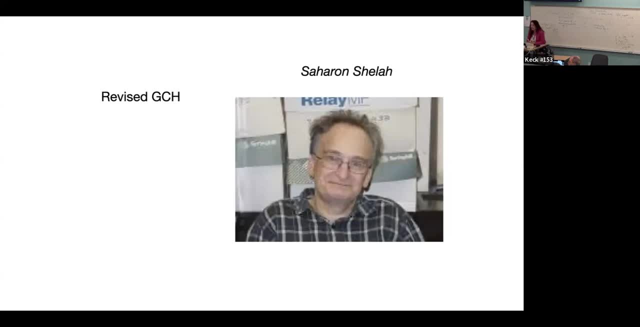 I can answer in a regular way, okay, I can answer in a regular way, okay, I can answer in a regular way, okay. so I actually work in the theoretical. okay, I've started the paper because I'm dealing with the automatic growth in geometry and what they did they. 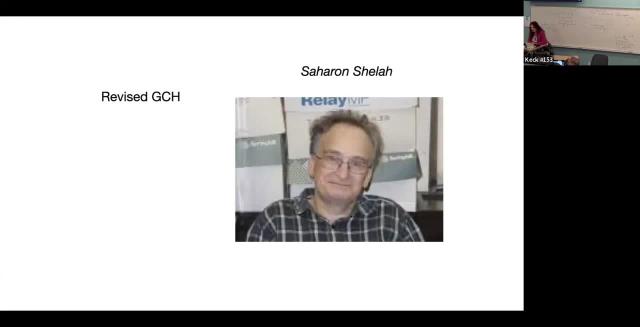 uploaded thousands of geometrical theorems, and they are those. however, it's not taught based on actions, or definitely not so this: there is no axiomatic background for this theory. for example, they assume that you can draw a perpendicular. however, in axiomatic systems, it takes a lot of. 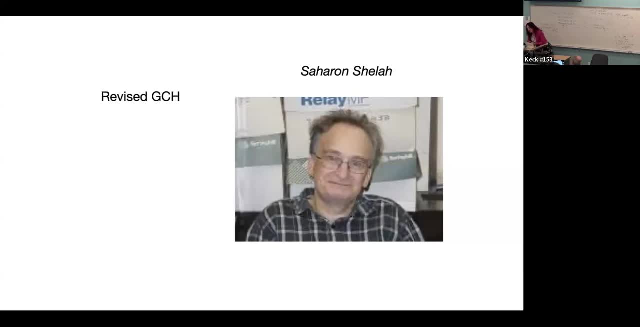 time to draw the yours. so, if I may, if I may address another question, because it's okay, go ahead. okay, because I defer, it's a good. it's a good, it's a good background for my question, because this particular problem, it's not based on axioms. and then the mathematicians. 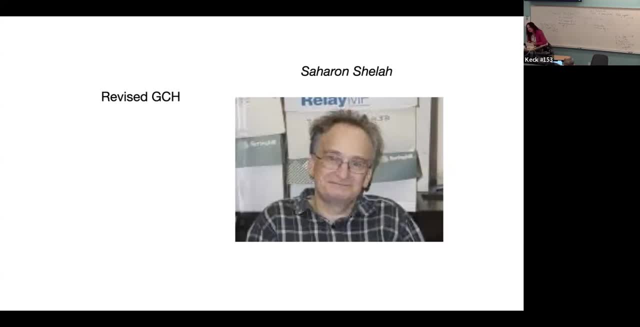 practice is not based on axioms as you, as you did for me. it's a philosophy, not in mathematics. let's say, for example, algebraic geometry: there are no axioms, algebraic geometry, non-standard analysis: there are no axioms or no standard analysis, or maybe there. 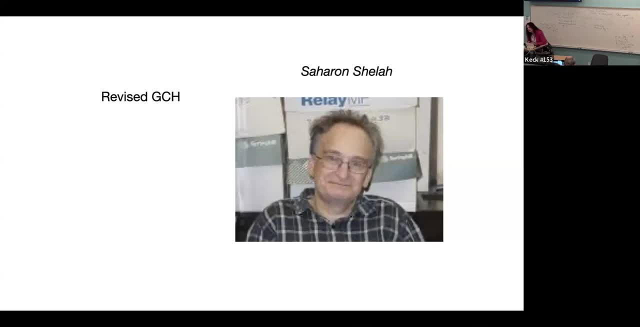 are different axioms. I even dare to say that there are no actions for the real calculus mathematics. it's not based on axioms, it's a philosophical idea, not a, not the idea of real mathematics. so, from my point of view, what we are talking, what you presented, is just a philosophy. 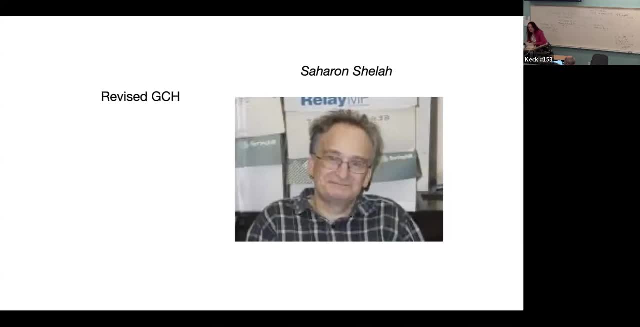 very technical philosophy, okay, but not mathematics. we are the mvp here, yeah, so I had a question about. it was kind of a technical question about your talk. you have row bottom, you said row bottom: cardinals, and then you say zfc proves that they do not exist. 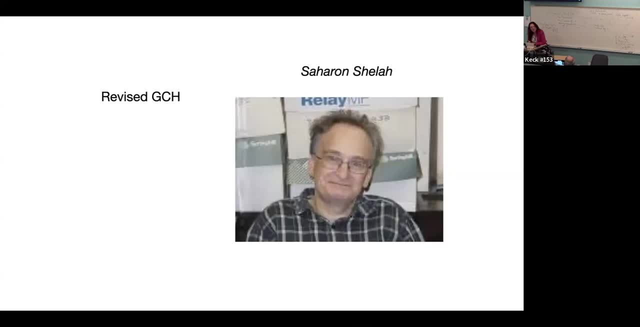 right. so in what sense are they cardinals? so I'll let you see I can answer that very completely. so they're not cardinals. like measurable cardinals are not cardinals. they are properties, as I mentioned. yeah, you didn't say that, so I want to clarify. 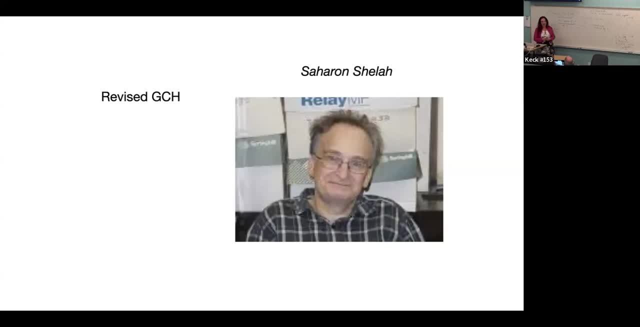 what is the property that makes a cardinal the robot cardinal is that there is a non-trivial elementary embedding. this means non-identity from vk to vk to vk. ah, that's the definition of a robot, and the woman showed that this actually exists. and you see, the point is that, uh, many. 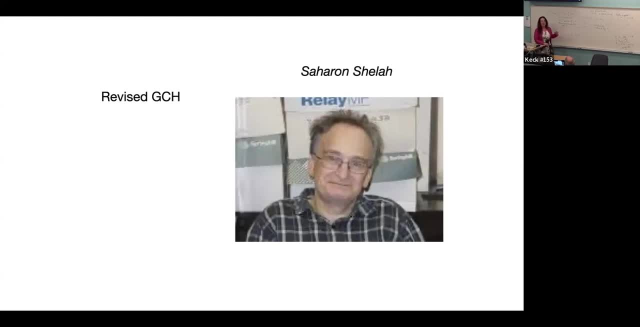 of these other life cardinals, or all of them, have an equivalent definition in terms of the existence of some element, and so the measurable cardinal whose existence doesn't seem to really complement something over here. so you need a definition of large cardinal as a roughly a cardinal. 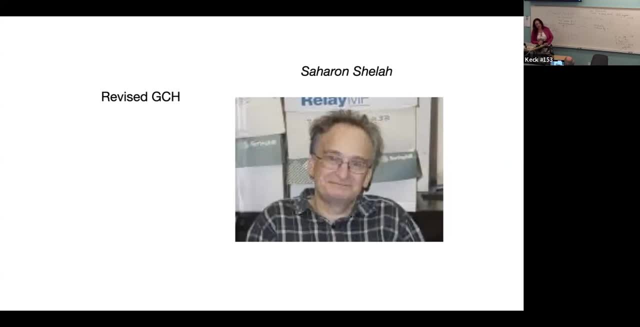 that can't be proved to exist in zfc. yes, right, yeah. and I know Tony Martin years ago talked about this idea, so for him omega is already a large cardinal, because you start from finite set theory and it's and it can't be proved to exist. 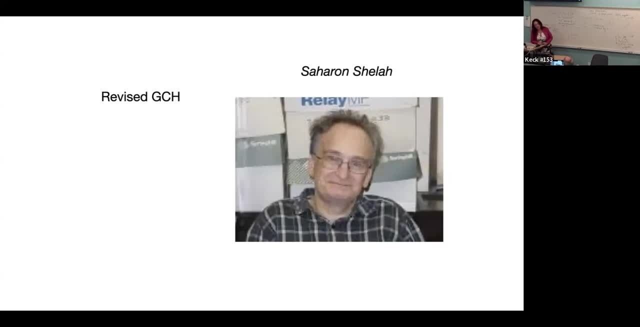 but it. but it's a reasonable axiom, right. so for him, a large cardinal is a cardinal. that is, a set that reflects the property of the ordinals. so, for him, the fact that the ordinals are infinite is the reason why you want to think of omega as being a large cardinal. 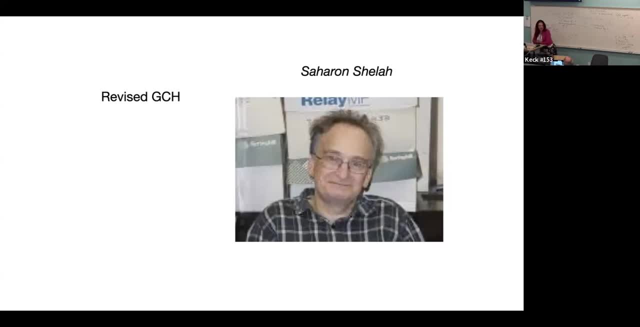 that's the, that's the first large cardinal, so to speak. yes, so that's the first large cardinal, so to speak. the first large cardinal is a large Protean, and so that's a different conception of what you mean by large cardinal. no, if you argue in the, in the finite, 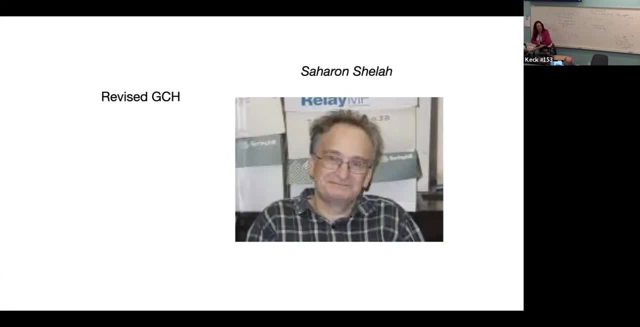 setting. yeah, you just have mechanical of chronicians. then this existence of omega, as you mentioned, cannot be proven, right? no, but my point is that, for for Tony idea of a large cardinal was that you look at so n you look at this, the structure of Of all the ordinals. 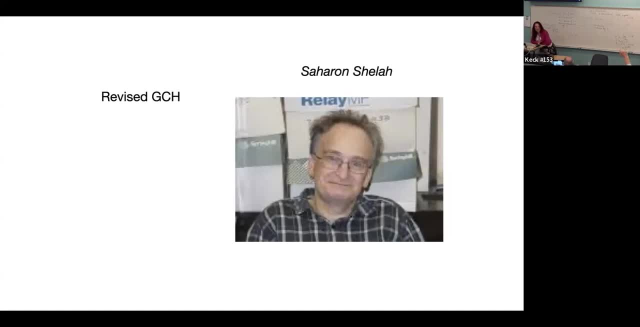 Yeah, And then you ask, well, what property does that have? And then you want to reflect, And then you want to reflect. So for him, large cardinals are cardinals that reflect a property of O-N. This is true. but you see, this definition has a small problem: that you have to know what the proper class is, because the O-N forms a proper class. So this is perfectly, this is true. 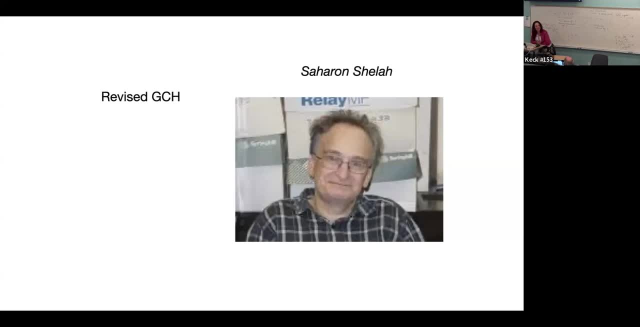 But that's another piece of this. what you called- I think you referred to- the California set theory, right, Yes, And it is a. it is a platonistic position, Totally a platonistic position. And what is fantastic about the work of Tony and others- but he was, I think, the most important contributor in this- is that they proved theorems of this type. 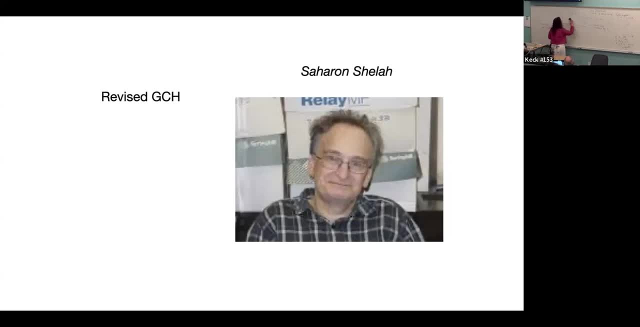 If some large cardinal exists, then you can prove that in some model. so let's say, consistence of the large cardinal is actually consistent To the consistency of all sets, subsets of R of some type, let's say projective or whatever, are determined in the game. 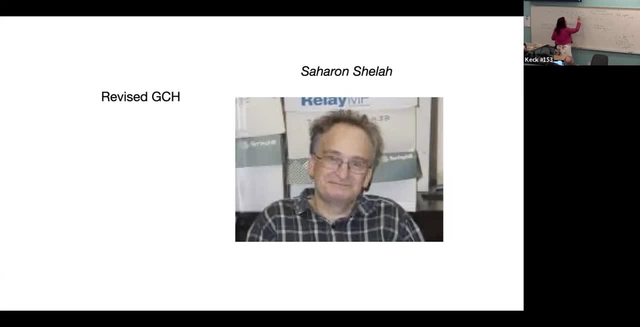 So, so I think, and they have a whole gradation, because we have a gradation of those types of subsets Here we have gradations of large cardinals And these two agree, And this is just about sets of real. So this is, I think, a very convincing argument. 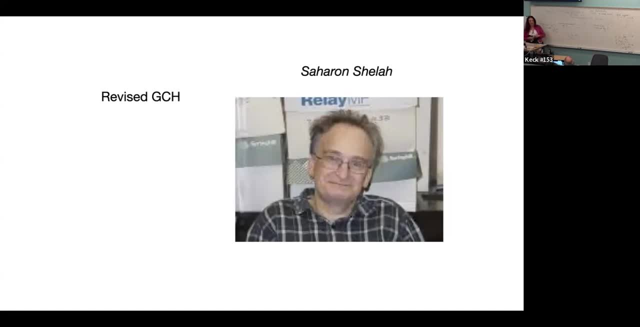 Yeah, exactly Yeah. So this is, as you pointed out, this is, this is descriptive set theory on this side. Yes, exactly Right, And perhaps this, perhaps I'll convince you a little more into the naturalness of this. 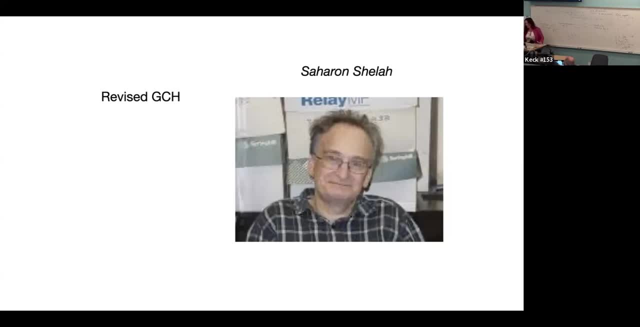 A little, Peter. Very, very nice talk. Thank you very much. I was wondering because you asked: what is an axiom. I think that an axiom is something that you would like to have to do your mathematics, And so it depends on where you work. 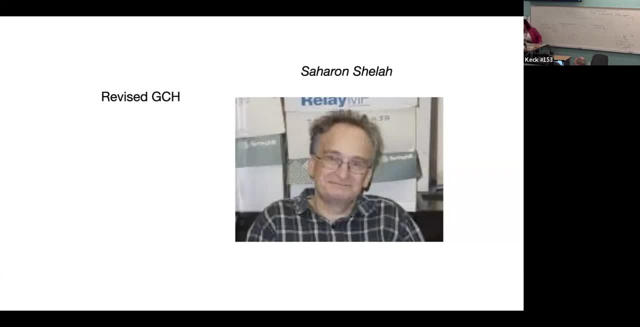 And that's why we have different proposed axioms, But of course, you would prefer to not choose an axiom that makes your mathematics inconsistent, And this is what can still happen. If you are Brazilian, you will. You're fine, sir. 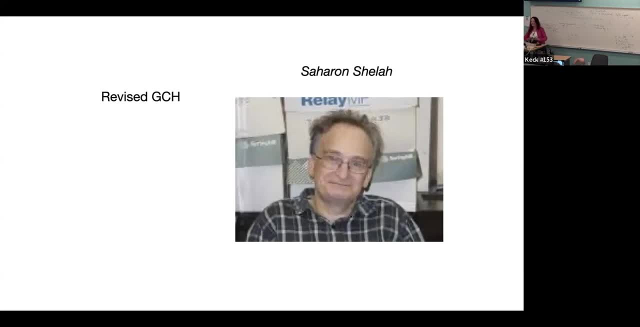 But this is paraconsistent. It's not inconsistent. It's not consistent, Yeah, And so we just got to the point where we accept that there are many different kinds of mathematics we wish to do, And the axioms help us understand which area we really work in and what we are assuming to make this worthwhile. 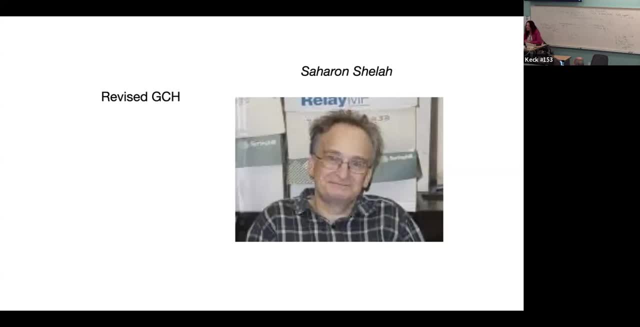 And all this can collapse. That could be inconsistent, We don't know. But it's to help us organize the space that we work in And I don't see a problem with axioms that talk about certain things. They talk about certain complicated forcing conditions. 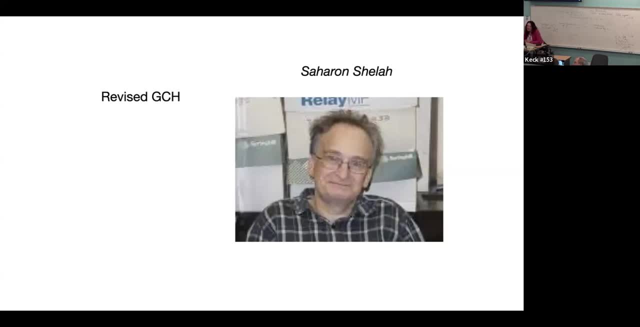 That's what you need to do: your mathematics. Thank you for the answer. Well, I couldn't agree more with 98% of what you said. You can agree with two more percent, So I totally agree with this. We work with mathematics. 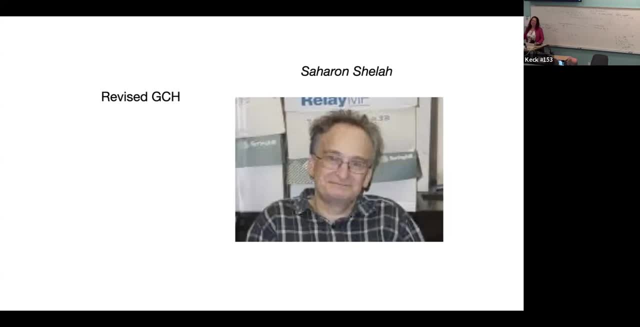 Except that these axioms, actually they're not formulated to do all mathematics. If you take, for example, proper forcing axioms, It was formulated as a consequence of results that people have had without using an axiom, And then it was said: well, look, now I could formulate the statement that I can do this type of mathematics as an axiom. 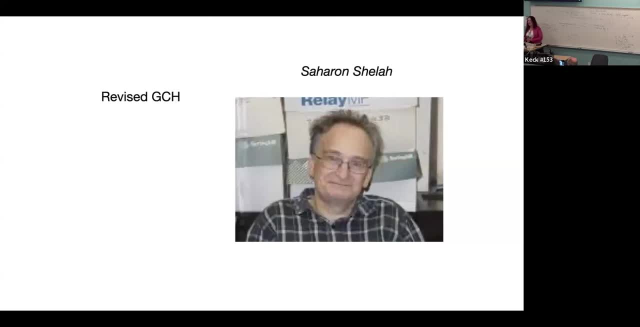 And then I could use this as an axiom. So it is not that this has helped discovery of mathematics, but rather the other way around. So that makes them somewhat less natural. Wow, This is an interesting point, because I wanted to react to Piotr in a way that is partially different, but perhaps 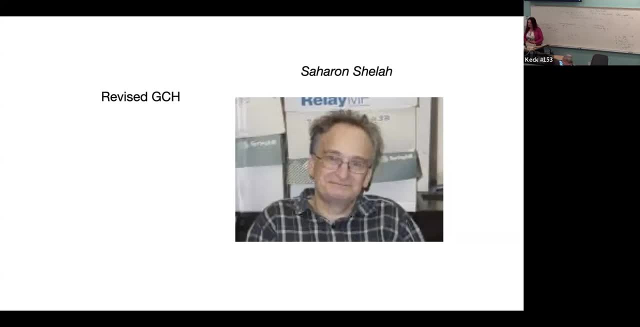 Okay, So the point is the following: It seemed to me that I totally agree with you, Piotr, that I could not agree more, in fact, that there are a lot of mathematics without axioms. I think that mathematics came before axioms. 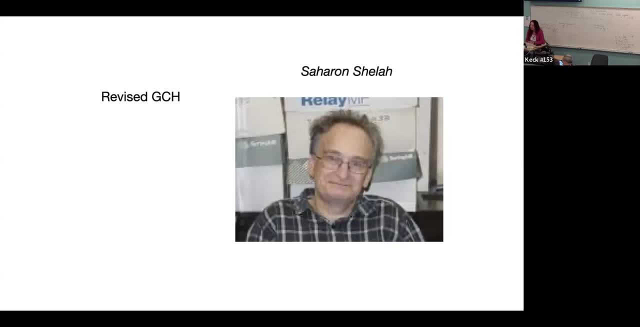 But I think that the theory is in a very positive way. The theory is in a very particular situation with respect to that, Because we can do geometry without axioms, We can do geofanthine analysis without axioms, But we do not know what the set is without axioms. 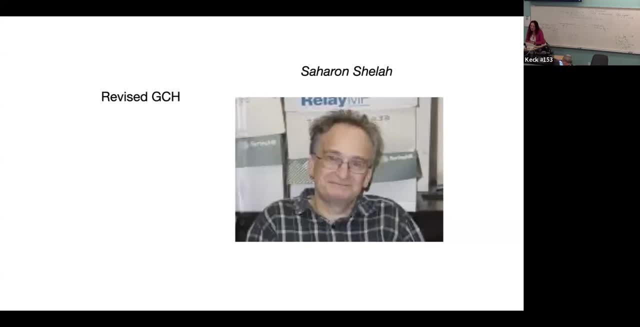 So the Zeta-F formulation, the Zeta-FC graph, is not but the Zeta-F formulation, If India is happy to make it clear to us what axioms are. So we are not in formal set theory. that is not contradictory. 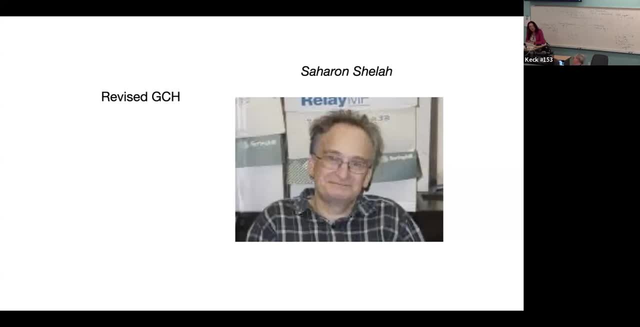 So you mean there is no such thing as set theory without axioms? There is nothing as informal set theory? The informal set theory is a way to work with axioms in a formal way. Of course there is in this sense, But there is no consistent set theory that can be done outside the axioms of Zeta-F or some other axioms. 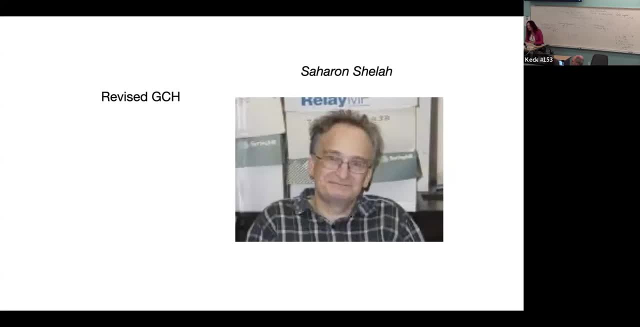 And in this sense the axioms that we can add are not in this way, Because in this sense the new axioms in some sense are there to formalize the informal mathematics that I've done, But at least the axioms are there. 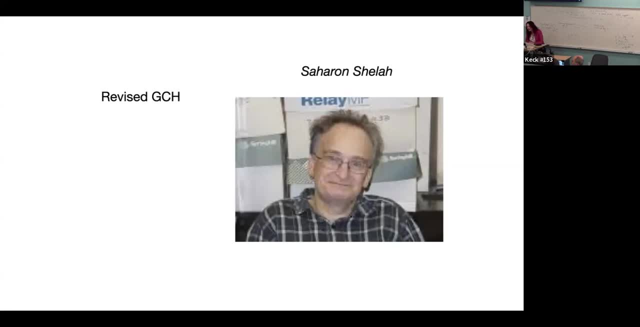 At least the axioms that I have picked up, without the regularity. The axioms are there to make clear what axioms are. We don't know what sets are without Okay. Some argument is this: that usually the axioms follow the mathematical practice. 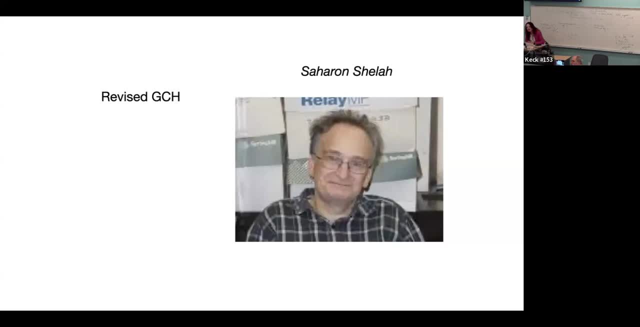 And they are to explain the practice In most cases, Yes, in most cases. So what is the mathematical practice, The mathematical practice of this theory, To what we refer when we provide some axioms? So let's just say, As Kavayes already showed a lot of years ago, 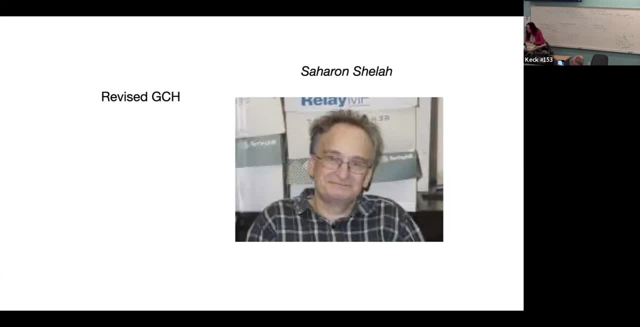 For example, the mathematical practice to prove convergence of serious theory. The notion of a set was used much, a lot before set theory. Yes, you see. Why don't you speak about it? Because it's a continuous function, Function with a certain number of points: discontinuity point. 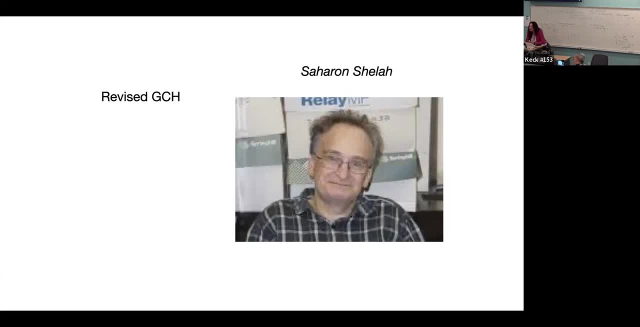 When you can integrate certain function of- not How many points you need, etc. It involves a very naive notion of set. So there are a lot of mathematics that involve a very naive notion of set. That is done with set theory. The problem that the paradoxes showed: 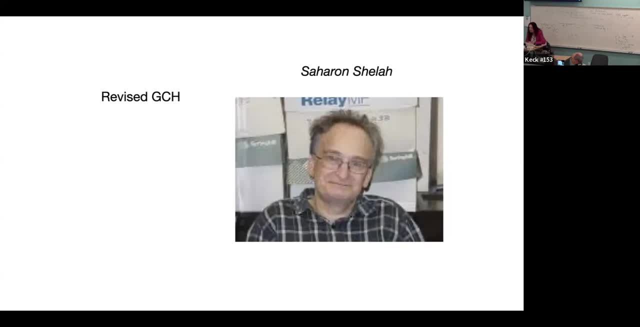 That this naive notion of set That is involved in this mathematics is contradictory. So we need to make it And you see, the point is that we- If I may continue on this discussion, The point is that That happened to set theory. 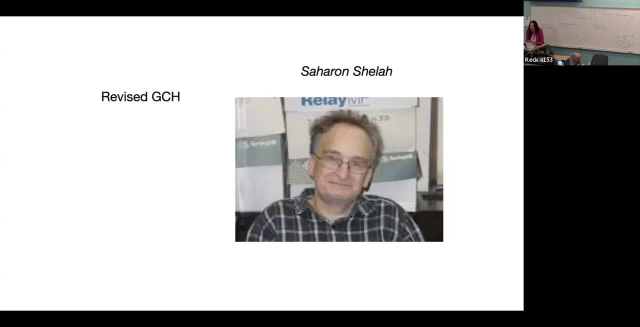 That something came That looked perfectly natural and was shown to be inconsistent. Well, this, I think, says that we need to be careful about that And that we need to have some manner of consistency about that, And set theory provides it. This is, I think, one of the rules of set theory. 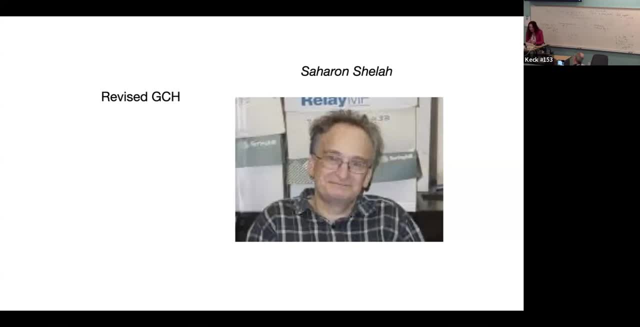 Although I don't believe in The generosity of foundations by set theory, I strongly believe in the strong role of set theory As a way to measure consistency of other theories. I think that's Okay. My, I could use a completely different. 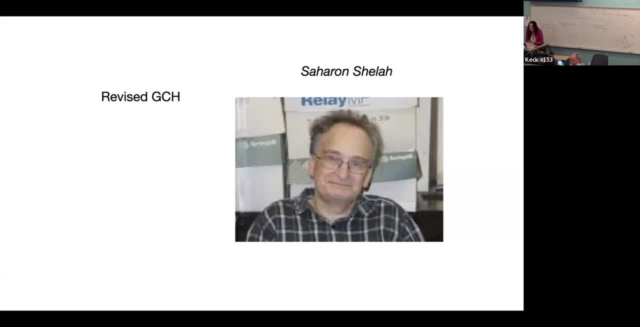 When we take MATLAB or Mathematica, They don't care about us, About foundations, And nowadays AI don't care about foundations of mathematics. So I didn't say Well, I should also point out that I never said that AI cared about foundations of mathematics. 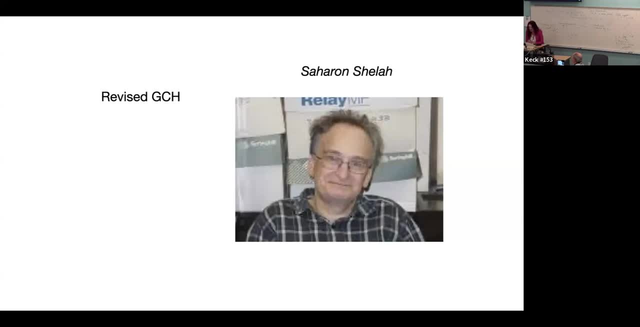 I said it cared about, And logic and foundations of mathematics are not the same, But I think as mathematicians we care about foundations. You know there are a lot of great mathematicians That would think about foundation here: Euclid Descartes. 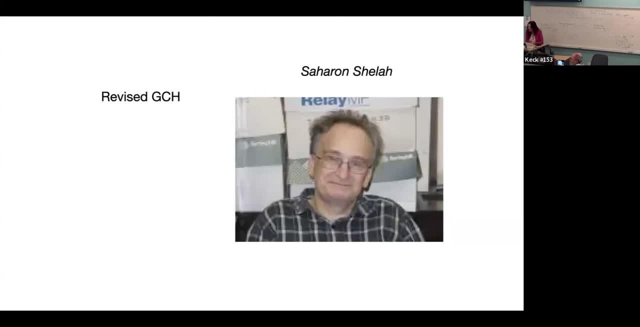 Newton, Leibniz, Hilbert Poincaré- No Poincaré, Perhaps Not Lagrange, Euler. So this, All these people were working about foundation And, of course, Michel. Yeah, I only wanted to say that. 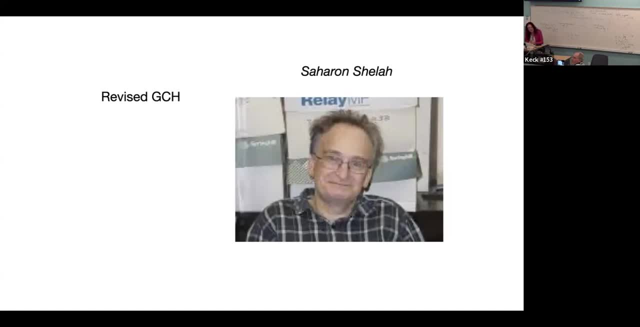 I don't think that mathematics can be done without axioms. What I think is that mathematicians, While they do what they do, They usually Do not speak about the axioms that they are assuming, but for sure They are assuming that they have some axioms. 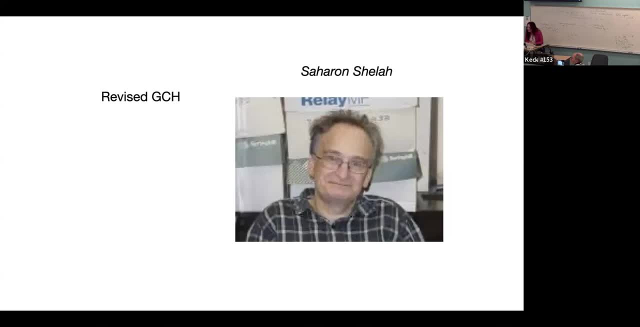 We perfectly know What are natural, number enough to make the analysis without that? No, I don't think so. I think that they are doing this. We are there, They are saying: okay, we agree that this is okay, We do. 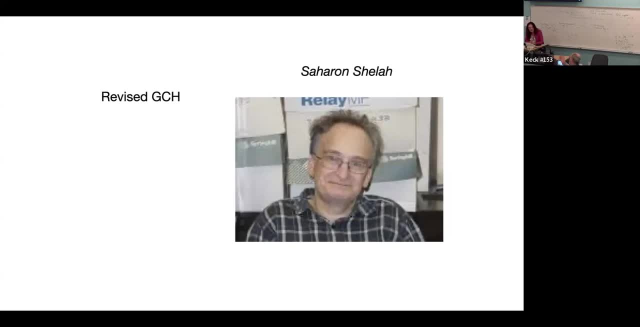 Do we agree that natural numbers are those? Okay, Let's, let's do then Equations, Different in equations, But I think that they start by Even, Even if they don't say that They start by agreeing on some, Some foundations. 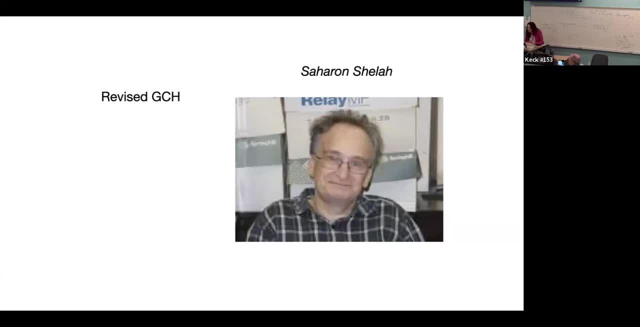 You cannot. You cannot do mathematics On a capacity to Identify And the basic Proper to some Objects, But it is, And that is axioms, Okay, Yeah, But the action In the end of the story. They're in order to formalize. 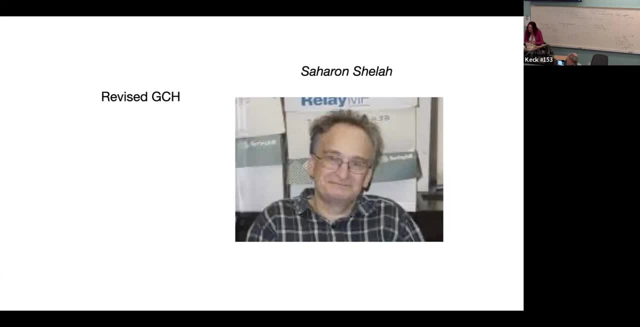 He's a believer. That came before the actions, The formalization, I think. so I know, Yeah, Michelle, And then So he went there, But he wanted to, If I can, Okay, Support Point of view. 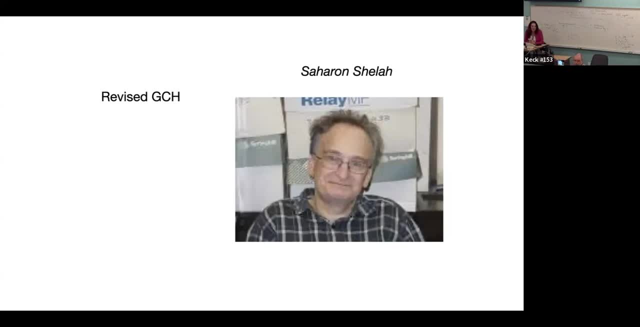 Because I would say that The, The, The, There, I would say that there Are Actually Many Mathematicians Who take Even Theorems As axioms, Because They wouldn't even Care whether the proof is correct. 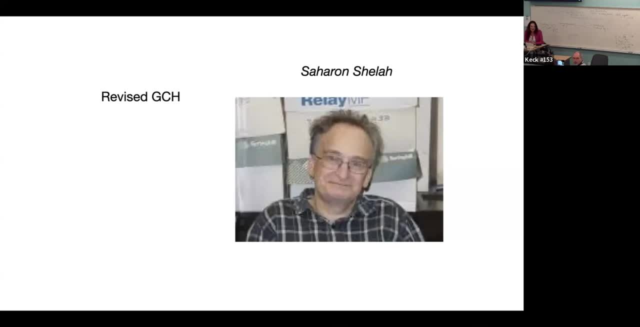 Or not I In many places In mathematics, You learn Certainly Rules Of behavior And not Logical Rules, And And You Perform Your theorems according to those Rules. rules, but they have axioms in their mind without knowing. 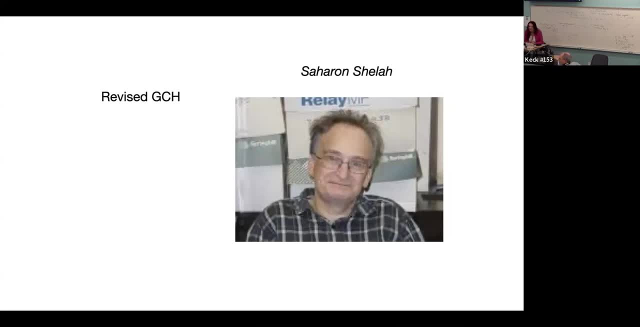 Without knowing. I do not understand- If the axioms are there to formalize a practice that is there before axioms. the practice before axioms in some sense implicitly contains the axioms, exactly because axioms are there to formalize the practice. 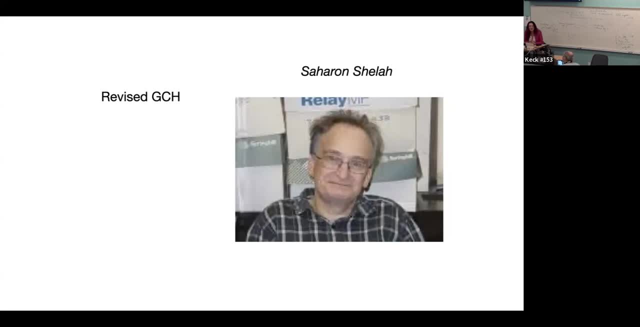 I don't know. Take our friend Daniel Struppa, that is not here but in this university, is everywhere and he does a complex analysis. As to him, what is the axiom that is applied? I bet you No, I don't know. 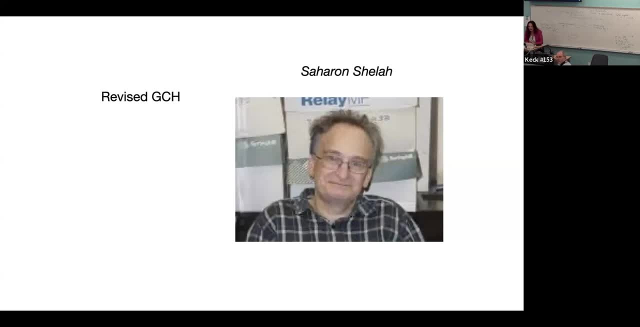 I'm not care of that. I bet you a beer that he tells me the axioms. Sorry, I bet you a beer that he tells me the axioms. Okay, So just to comment on Pino. Pino was making the point that there is no axiom. 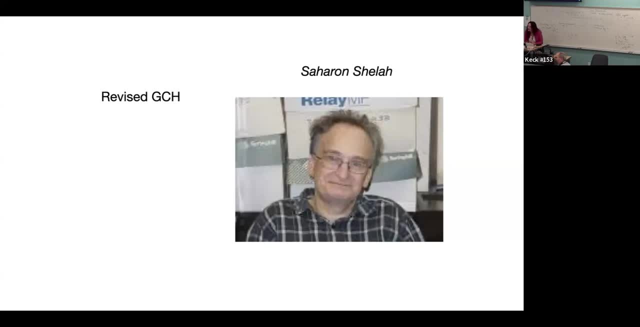 We have rules of behavior which come about axioms. Axioms is already a sophisticated way of enforcing some axioms within practice. I wanted to come back to the question of Piotr, which was about: is there a mathematical practice? 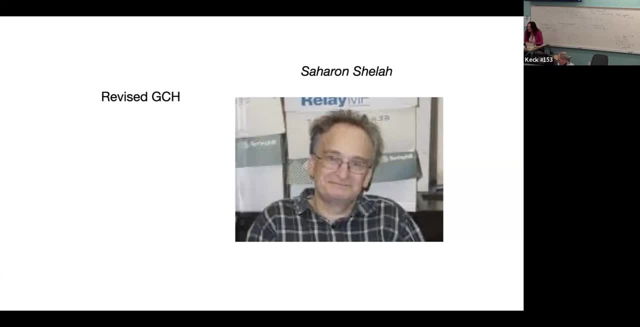 And I think that from your talk we hear that there are at least three branches of this mathematical practice with sets, which is definition, Descriptive theory, combinatorial set theory and the work of Saron Shella- because you presented it as a kind of investigation- which is on the basis of ZFC and which is extremely 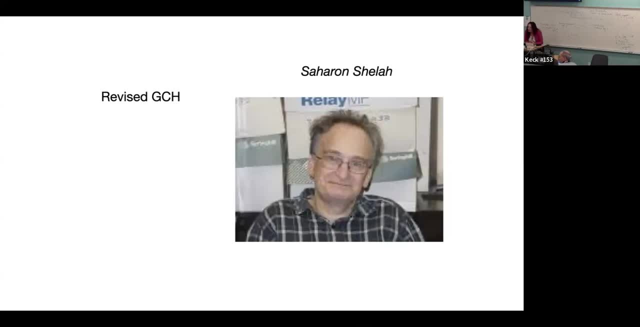 interesting, And so if we are looking for good axioms, it could be in order to have a framework for all that. Of course, You were describing a practice that I wanted to insist on. Yes, Well, certainly There are different branches of set theory. 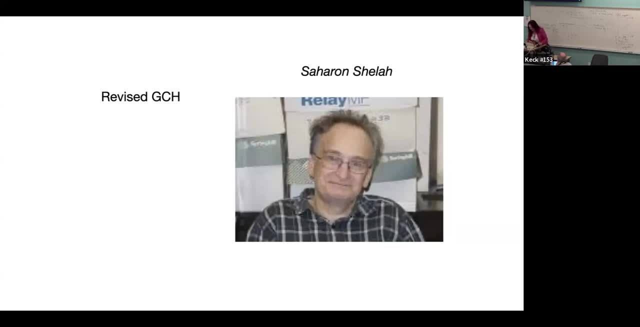 The practice of set theory is very wide. The work of Saron Shella is perhaps not a different practice. It's an overwhelming practice because I think he has done work in almost every part of set theory. But there's more on the combinatorial side. 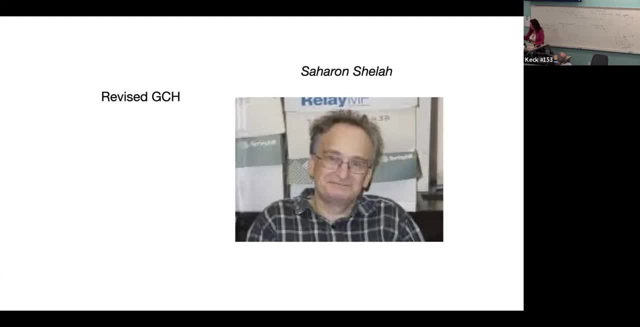 Some part of his work is about large cardinal axioms, Much of it, Yes. So this is the particular work that I described I wouldn't like to use. Needless to say, This is the particular there I. they may join that. 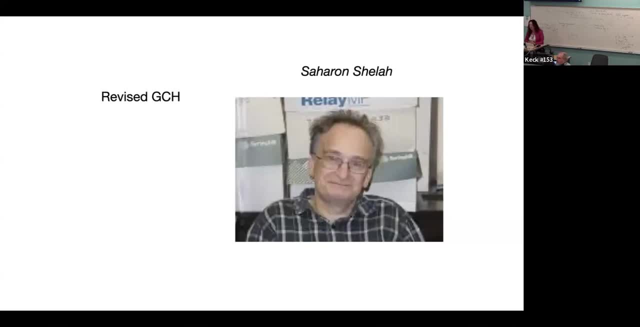 Yeah, it's related to your point about not knowing what sets are without the axioms, And I mean I could be wrong on this, but no one objected to it, But Marco asserted that, But I always understood The situation would be that there was the iterative conception of set. 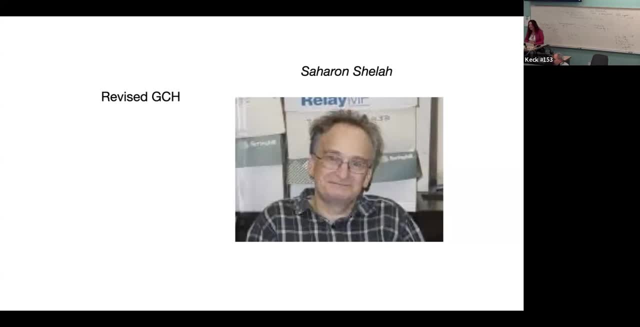 And that's something that I think is very important, And that's something that the axioms then codify, but there's this conception of sets that is outside of the axioms, and we don't need the axioms to understand the iterative conception of sets. 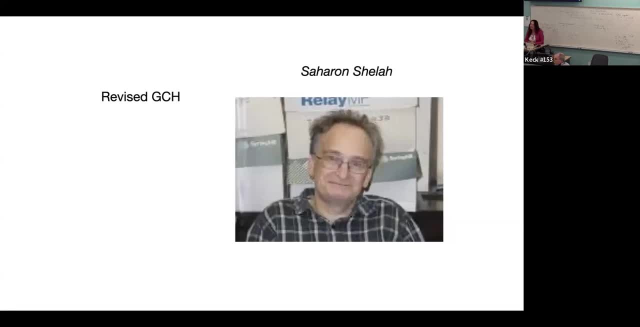 What do you mean by iterative conception, The iterative conception of sets that you say Yes? what do you mean by that? Built out of the natural language, Sorry. Or sets built out of the natural language, Or just from the empty set. 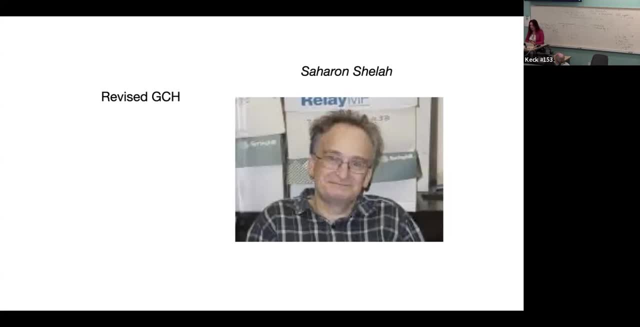 You mean the cumulative chiral? Yeah, So I mean, this is my conception of it, which is against the idea that you need the axioms to understand the iterative programming. So you mean that we do not need the axioms that I've seen in order to understand that an empty set is a set, that there is a singleton or empty set of a set, et cetera, et cetera, et cetera. 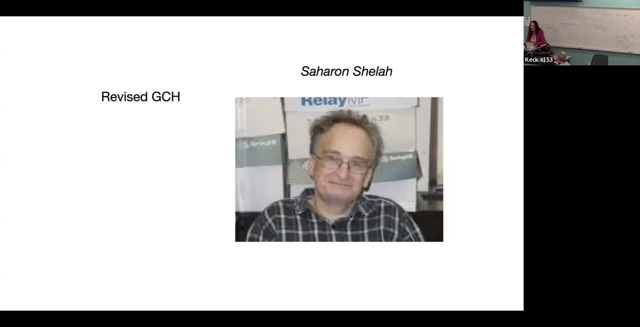 We equal. well, I agree. Is that an axiom or a consequence? No, just a way to summarize what I said. That's what he says. We agree that sets are just cells. We need no axioms. Yes, Our notion of set is: 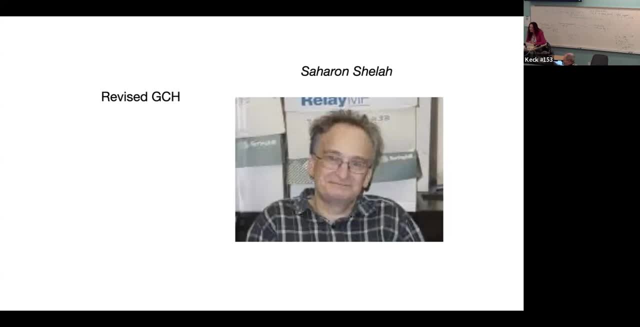 But still there is a big problem: How do we define the new sets? And then you need comprehension, And when you have comprehension you need contradictions. Sorry, You have no way to equalize comprehension. I would say Piotr. 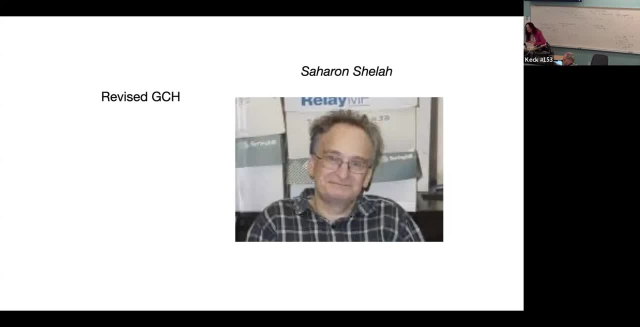 Okay, May I go back to the history In 1947.. What is Godel's continuing hypothesis about? And in this paper, this very paper, he argues that there is no alternative to the theory of infinite numbers, Cantor's theory of infinite numbers. 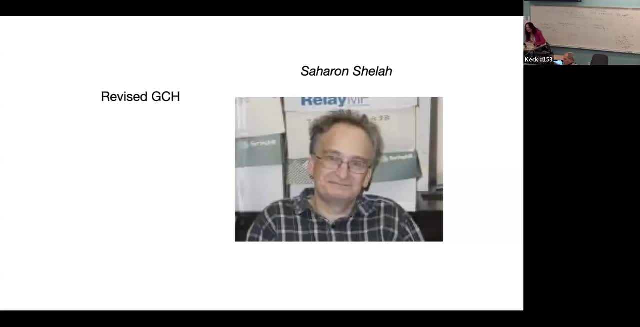 It was published in 1947.. In 1905, Heisenberg provided developing alternative, a so-called natural product. This is about ordinal numbers. Ordinal numbers- He refers to ordinal numbers. How can you explain it? What did Godel say exactly? 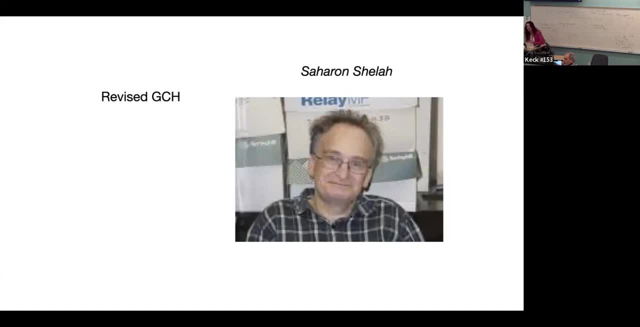 Excuse me, Could you repeat this? There is no alternative for Cantor's theory of infinite numbers. I don't think he. He refers to ordinal numbers. Anyway, Forget the Godel, This operation, the natural product and the natural sum. 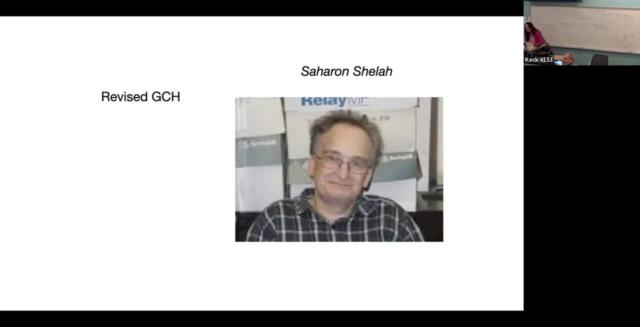 doesn't have any impact on the problems you're dealing with. Well, this is a fantastic question, actually, Because what happens is that there are questions about countable orders that are still unresolved since the 1950s. These are the questions that mathematicians 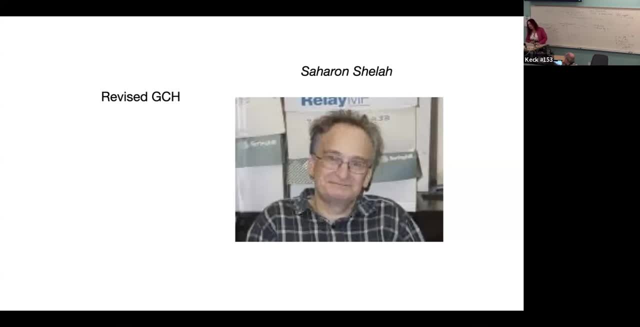 and computer scientists outside of the century want the scientists to think about, But most of our work does not apply to all of this. None of these things say anything about ordinal numbers, For example. here is a question that I can tell you immediately. 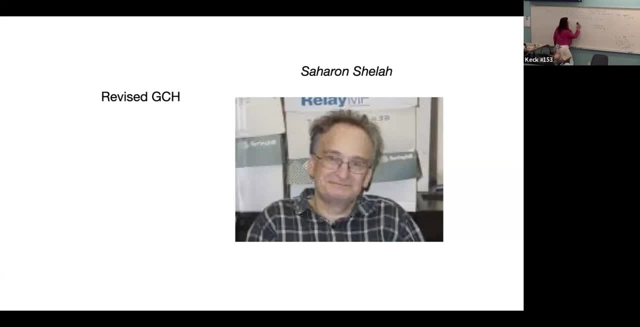 Take three ordinal numbers or four. Take four. I think for three. it is now known. Look at the product of four ordinal numbers. Look at it as a partially ordered set when you look at sequences from this product and you look for an ordinal invariant. 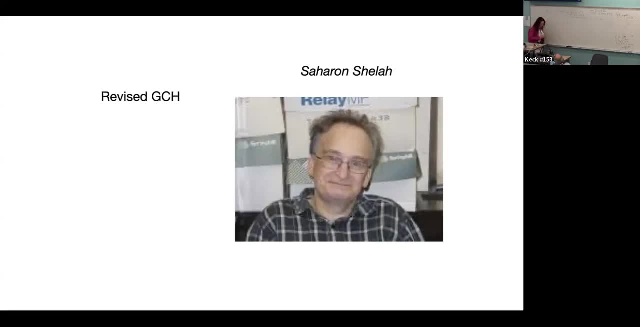 which is called double weight. This is defined as the rank of the three incompatible sequences in this order. So it's a countable, It's a rank. Can you express this in terms of these orders? It's known for two, It's known for three. 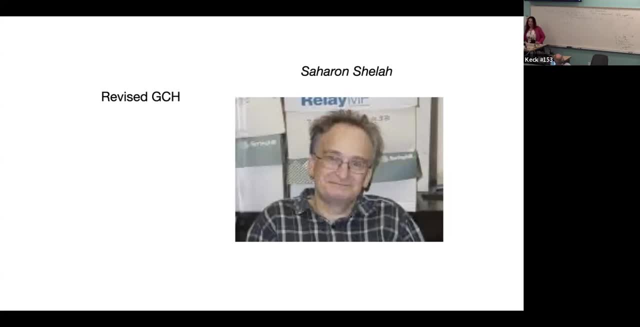 It's known for four. It's been open for a very long time. There are papers written on this. And why do people care about this in computer sciences? Because they use such ordinals to model processes and these operations have something. And the answer: 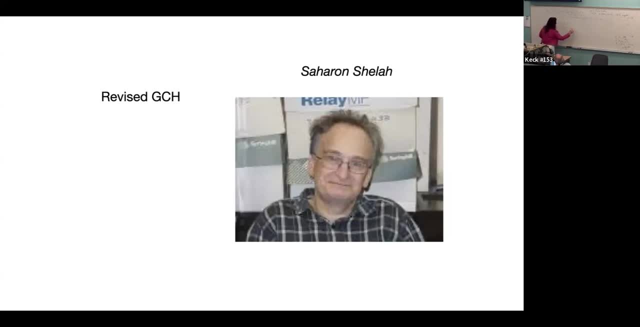 is to be exactly the formula that we know about. So they do come up. They're not sure they're nice, And set theory doesn't deal with that. It simply just does not. It's invisible to set theory. Here is an open problem. 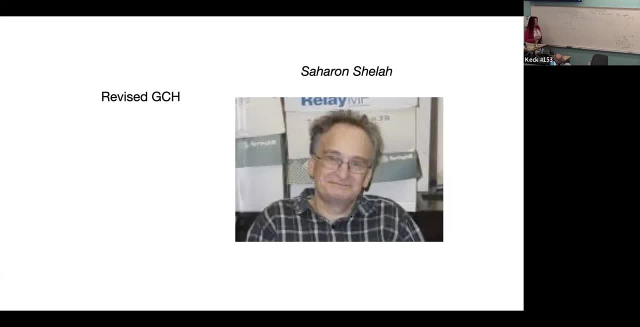 from 1956. Characterize all countable ordinal cells such that every time that you color the pairs of alpha into two colors, there exists either there exists, so two colors are called zero and one. there exists. a subset of order type alpha, called subset H, such that all the colors 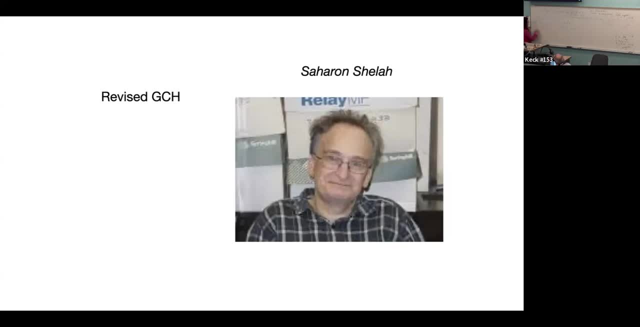 of H are zero or there exists a subset G of size three, three such that C restricted from G is one. Characterize those ordinals Since 1956? question by Erdos. some work, very important work, was done by G Larson. there are no methods. 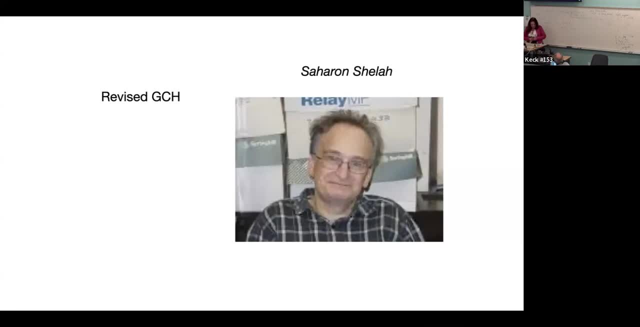 of set theory. this is all done by hand and I actually thought that we could advance this by using automatic theorem provers. if you want, I have a paper with Laurie Paulson and Angeliki Kutsuku- Agiros Kutsuku- where we tried to reproduce. 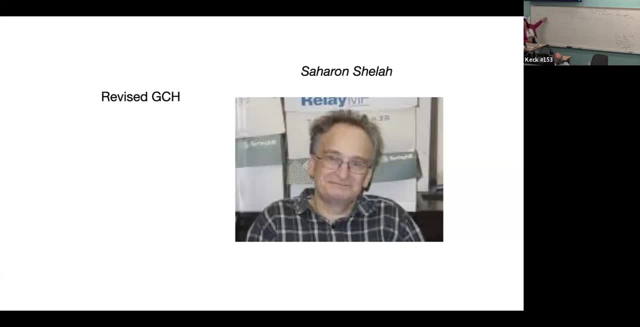 some of the known results in this using to formalize, with the hope that we would build a library of knowledge that then we can use to finish. but this is hopeless. We are building a library in Isabel. If you are Laurie Paulson who speaks, Isabel as much. 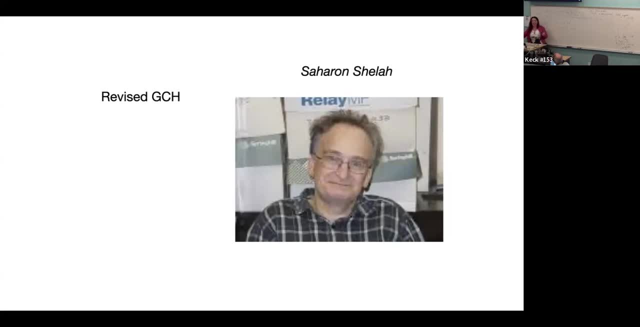 as he speaks English. it takes you six months to formalize the first ever paper that G Larson wrote. So for the moment it's hopeless, But I think that maybe this type of problems is a big, has a potential That could exactly be the way to fill in the missing. 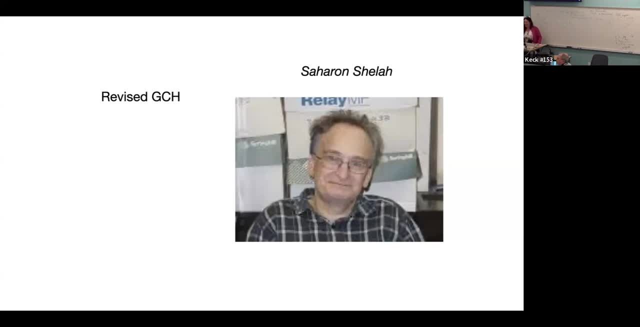 gap there, right? Okay, So I remember this very long and nice discussion, only regret that you put three problems there. what this foundation of mathematics discuss, You answered the way what is action, But this to solve a problem not work. So I would like to know: